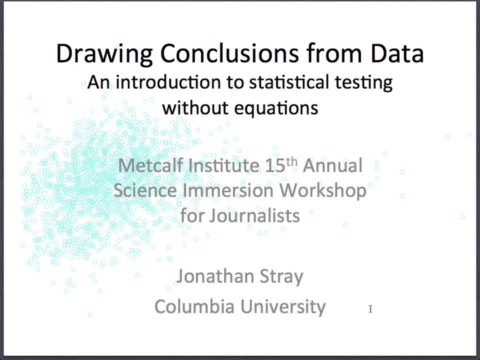 show you the underlying logic of statistical testing and in fact, we're gonna start with: what is that and and why do we care? And, as promised, there is not a single equation in this talk. The trade-off is that there's some code, small amounts of it and doing, I think, relatively straightforward things. We're. 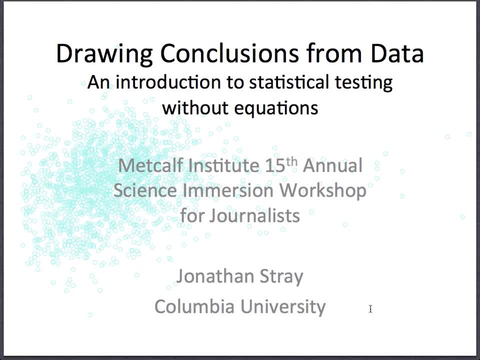 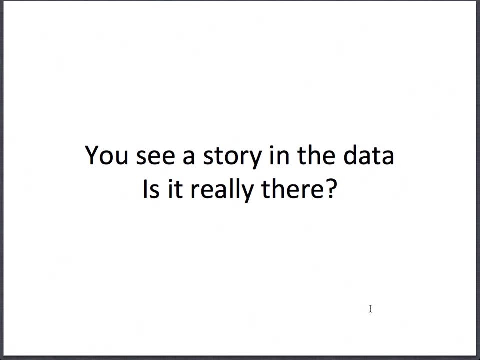 gonna. we're gonna talk about a lot of rolling die and rolling dices, dice, dice. there we go. Somebody call a copy editor, Like a lot of rolling dice and sort of taking random samples and things. So this is the problem that we're trying to. 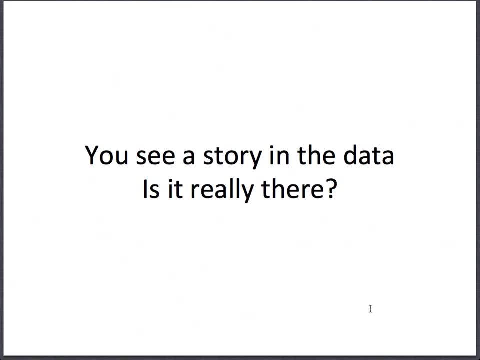 address this morning is: you've plotted, say you plot your data on a map and you're like, wow, everywhere that it's near an oil refinery has a higher cancer rate. and the question is, The headline you want to write is: pollutants from the refinery are causing cancer. Is it justified? 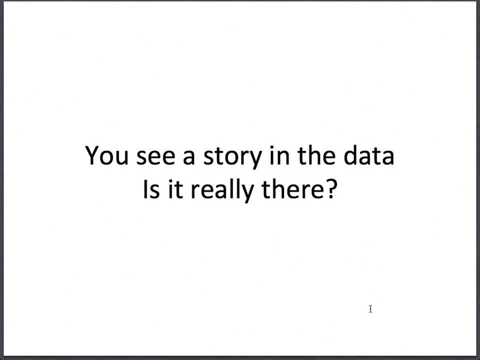 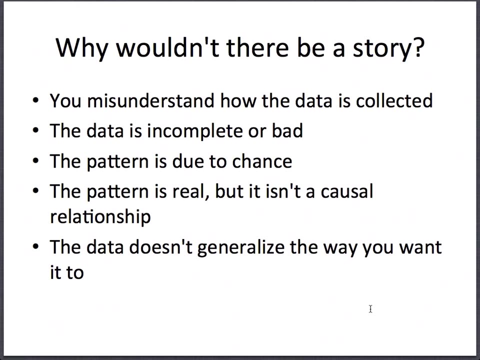 There's a lot of reasons why what looks to be there might not actually be true, and we're going to talk about a lot of those reasons, So we're just going to jump right in. Okay, so some reasons why there wouldn't actually be a story. when you think you see something right, You've plotted your. 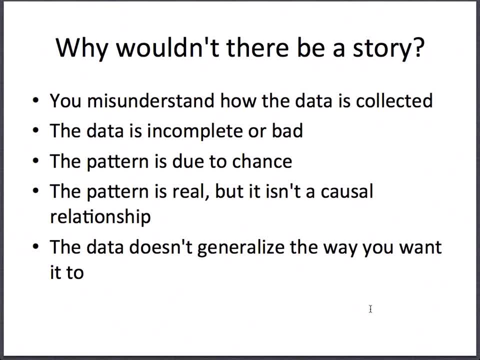 cancer rates on a map. So, first of all, this will be up as a video, The slides will be available, The code would be available. So anything that I show you today, don't worry about trying to take down. You'll have it all. 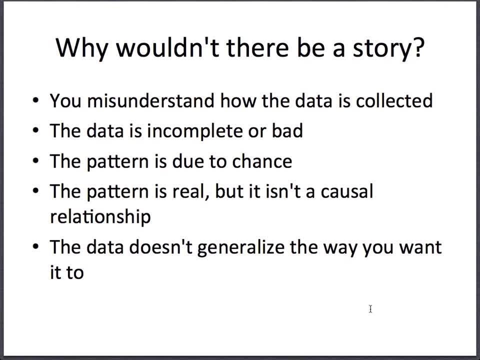 These are some basic reasons, right. The first two have to do with what the data actually is, where it came from, what it represents, how it's counted. and then the middle two have to do with really the heart of what we're going to talk about today. 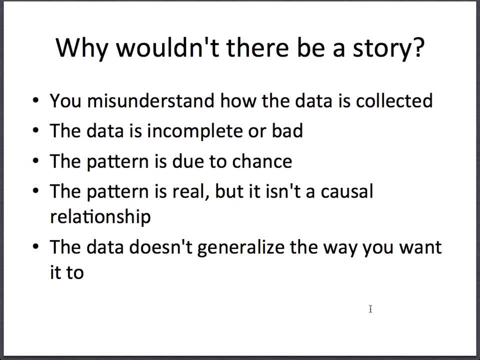 statistical testing why you need it. We're going to spend most of the time talking about chance. In fact, an earlier title for this talk was the shape of randomness. I want to give you an intuition this morning as to what randomness looks like. 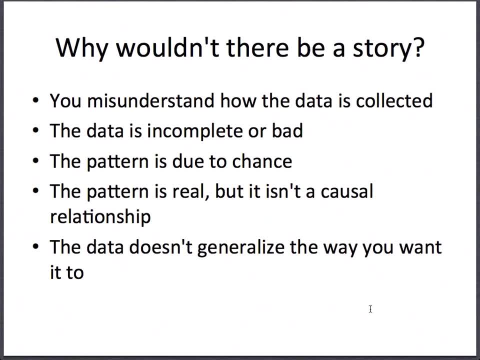 Because randomness doesn't look like what most people think it looks like It's. Randomness has far more pattern in it than most people suspect, and we're gonna. we're gonna try to show that this morning. And then the last thing we're talking about is generalization. 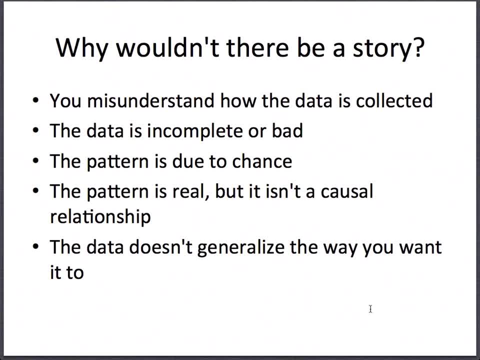 Which is very often when you're writing a story. You know you, you talk to five students, But really the story is about the experience of all students and those five students are standing in for that. so we're gonna say a little bit about when You can. you can make those sort of generalizations to go from the specific to the general. 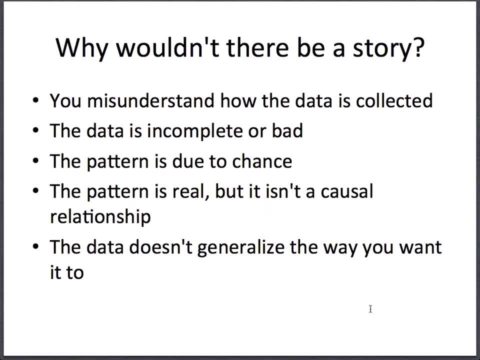 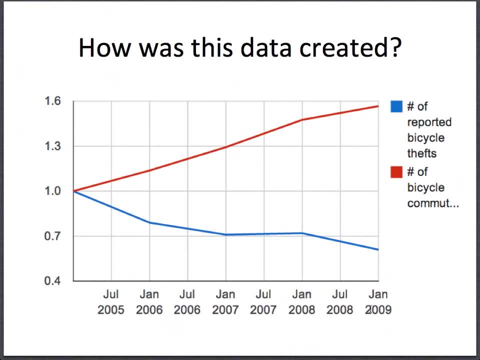 This Is one of my favorite slides because it's about as simple a piece of Data-driven reporting as you can get. this is actually done by one of my students in a workshop last year And I trained them to use some basic graphing tools And I showed them where a bunch of government data could be found and I said, okay, go find me a story. 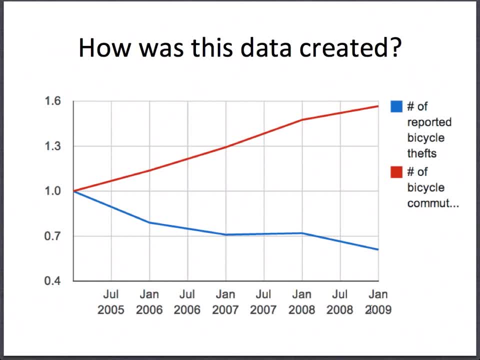 You have three hours And this is what They came back with. they got data on. this is actually in Eugene, Oregon, I Think all Oregon- for these numbers- the number of people commuting by bicycle and the number of bicycle thefts- right, so they're at the top- is. 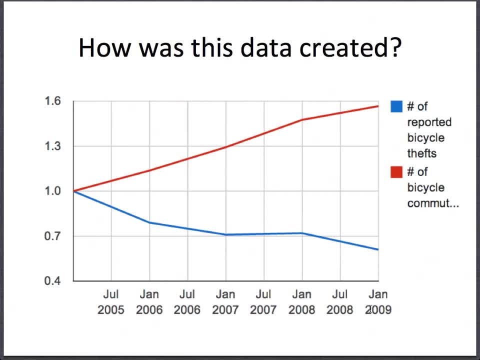 In the red is the number of people commuting and in the blue is the number of thefts, and we see the pattern over in five years. What's what's wrong with this? There's a million reasons why bicycle thefts can be done in the United States. 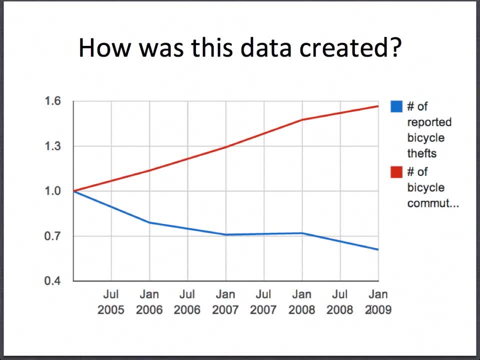 right, but There are you thinking other than just a number of What's that? Yeah, we'll get into all of that. I mean good, but but when I look at this chart, something immediately jumps out at me as weird. Well, yeah, because if you think there are more people commuting by bicycle, there are more bicycles around. 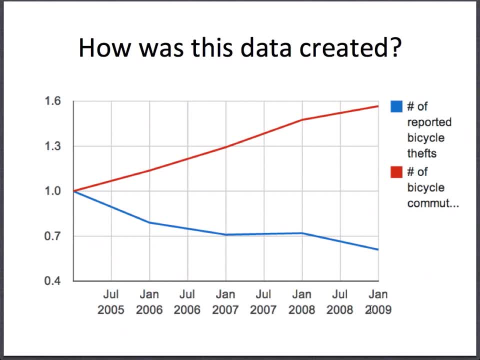 you expect a proportional number of thefts to go up the same way if you don't consider other variables, Right? so commuters are going up, thefts are going down, so they're normalized to the starting year, which was January 2005. just so you can see the comparative. 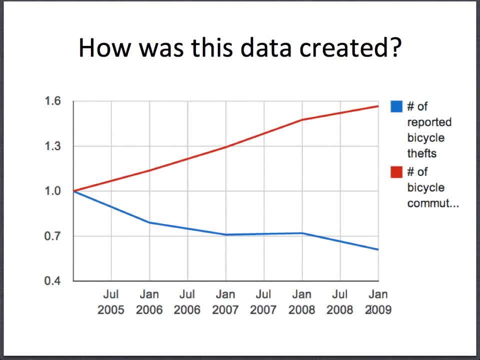 differences. so you know, and you see they've gone, they've sort of mirroring each other, which is kind of weird, right. and so the student showed this to me and said I don't know what's going on. the first thing I said is: well, okay, well. 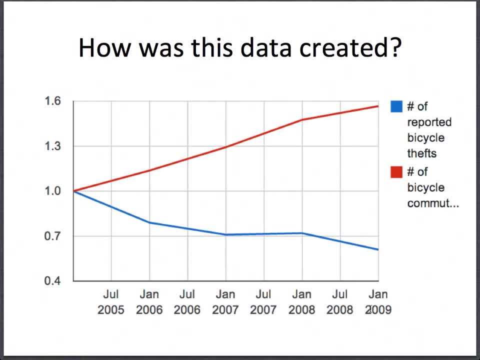 first of all, you've got a story, because either this is really happening, and it's weird and noteworthy, or it's not happening, which means that something is wrong with the official statistics. so I asked how we could check the these numbers. so I'm gonna ask you: how would we check these numbers? you know, say, 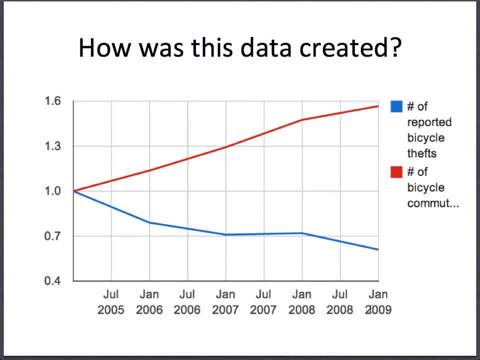 downloaded them from a government website. yeah, so they are actually police report data for the thefts. anyways, the commuting numbers, I'm not sure who collects those. yeah, yeah, that would be so congratulations. you have, in one question, hit upon what it took my, my journalism students 10. 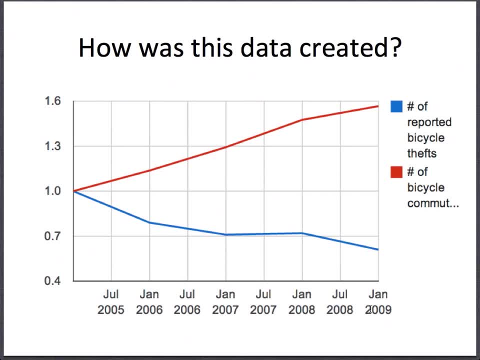 minutes to get to. so they were talking about. well, we could, you know, read the footnotes on the data and compare it with other data sources and you know sort of all of this, all of this sort of internal consistency stuff. but the first thing I would try is call up 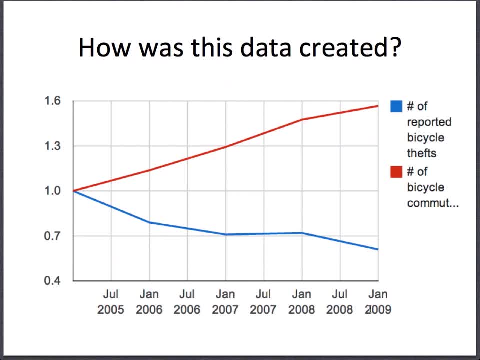 the person who collected the numbers, right, right. so data doesn't come from nowhere. it comes from a person, ultimately, or a group of people. it's collected by somebody for some purpose, and until you understand where that number comes from, you don't understand what your data can't or can't say, and so 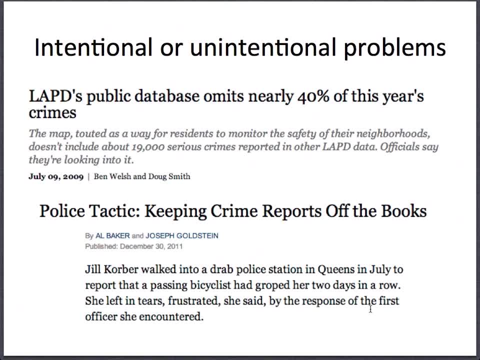 if you were to look at the data and you can不到 that number, you could say: we're gonna have funny, so you can have unintentional problems as in. so here's the same type of data, right crime data, and in the first instance the Los Angeles Police Department published this crime map to much fanfare and said now: 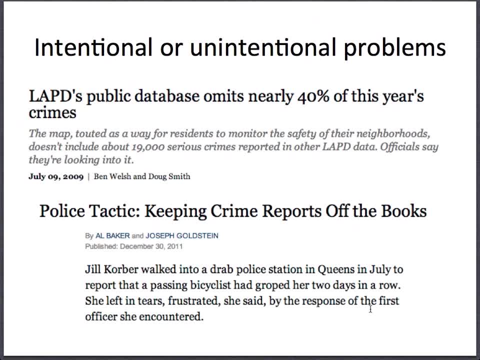 you can see where this crime in the city only when the Los Angeles Times started pulling in the data feeds both from the LAPD and from the sheriff's office, it was a complicated process to get it all in one place and made their own map. this data, coming from plots, resembles data that exist within the area and then you can call that as quote anti-h опасities issues. as an additional important factor is to remove where there is crime. I think the DOJ isや. 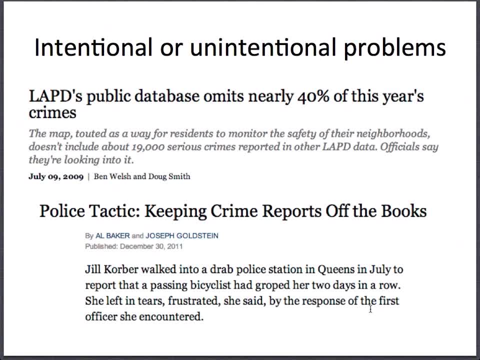 discovered that the crimes were missing. They don't think this was intentional. the LA Times people, As it says: you know officials say they're looking into it. it seems to have been just technical sloppiness. In other cases there is 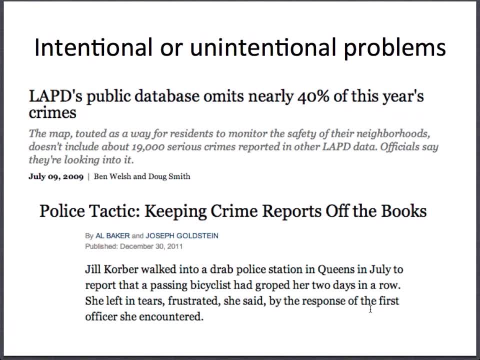 intentional deception going on or, let's let's say, counting that favors a certain interpretation, right? So this story from New York is the lead. there is about a woman who walked into the police department and said: you know, two days in a row, this guy on a bicycle broke me as he rode past And they said: well, you know. 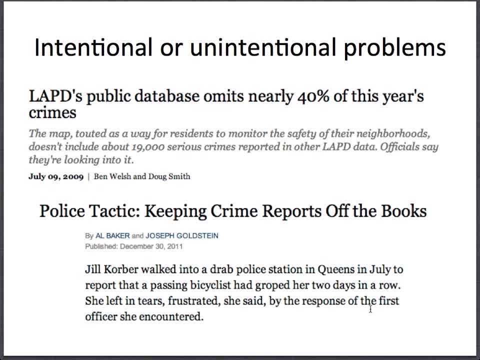 we don't have a name, we don't have an ID. you know, there's really nothing we can do. sorry, Which may be true. however, they didn't count. They counted it in their crime statistics, right? So it turns out the police weren't. 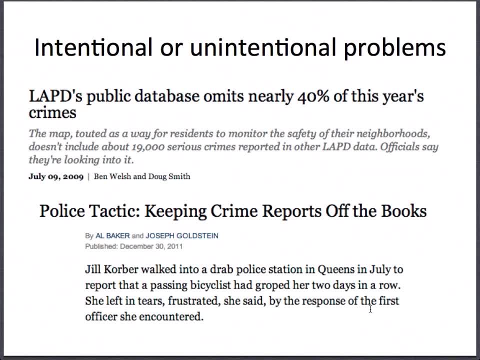 reporting crimes that they had no way to follow up on, Which almost makes sense, right, if you're looking at the statistics in terms of you know cases, right, But you don't want to count cases. you want to count reports in this case. So you really have to ask where. 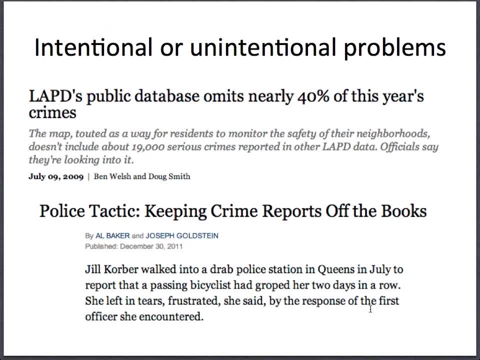 these numbers came from, And this is not unique to New York. I found three other cities where there were stories about bad crime data in the last couple years. That also happened in LA and Milwaukee, I think. So one can only imagine that you know this is happening. 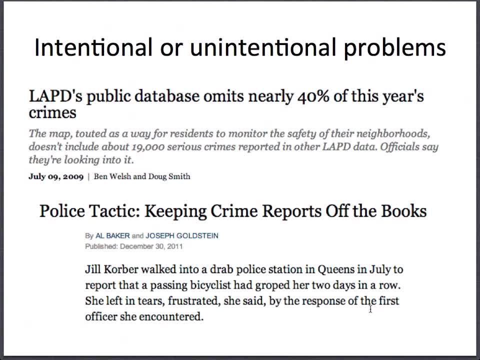 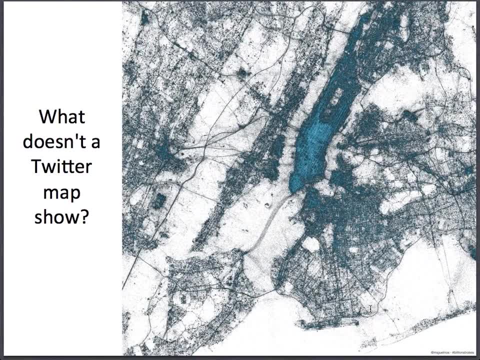 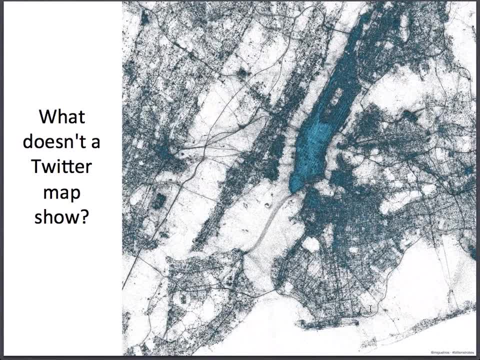 I live in New York, so I have some idea. when I looked at this, what was wrong with it And I had my suspicions. What's this map going to miss? What's not going to be on this map? So what it is is it's every time someone tweets when it's got a location it's going. 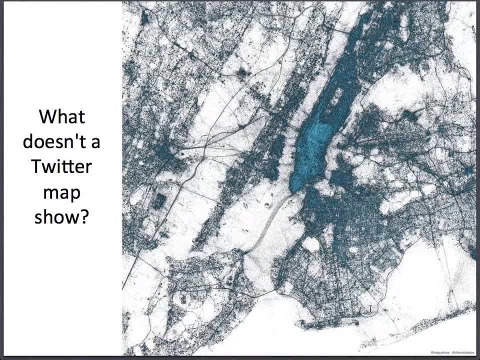 to make a dot on the map And it's a heat map. so the lighter blue areas are a greater density of tweets And it's an accumulation over several years And they're saying: wow, you know, you can see. it's amazing, You can see all the highways, You can see the areas. 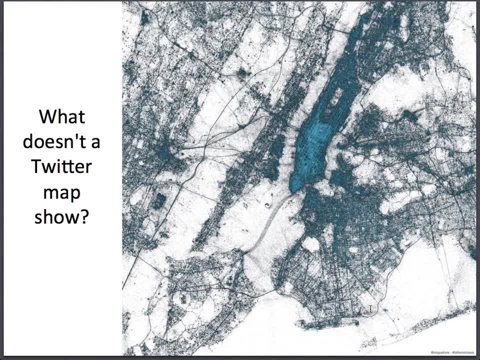 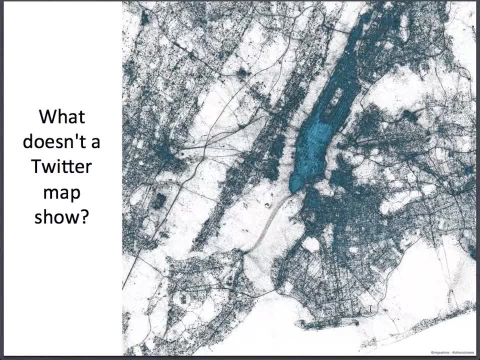 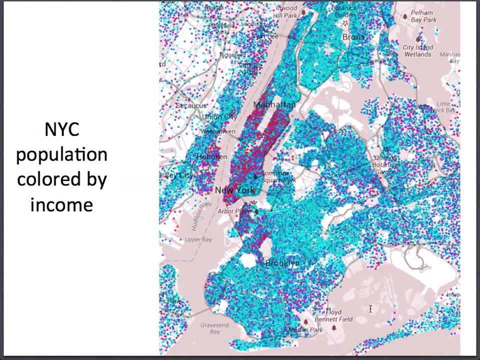 by some people. This was presented by some people. as you know, this is an amazing new way to make maps of the world. Well, no, It's an amazing new way to make maps of Twitter users- Right, Of course, Twitter users who are using. 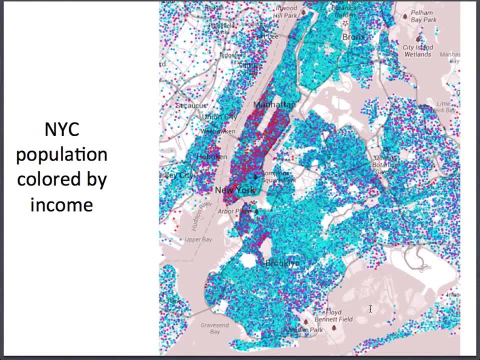 And Twitter users have particular demographics, So take a look here. So New York is dense, right? So look at Brooklyn. This is, you know, it's all filled in with dots. Each dot is a hundred households. I think Right. And 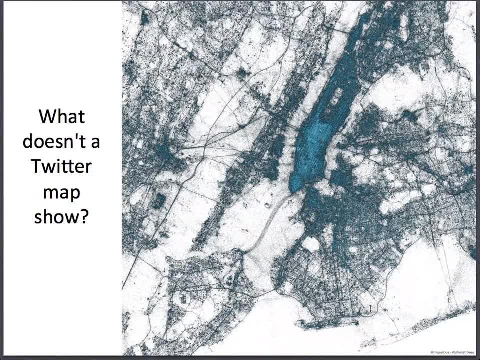 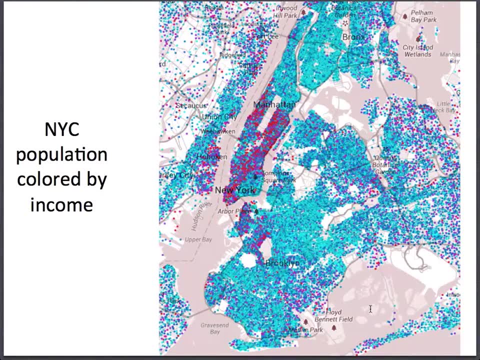 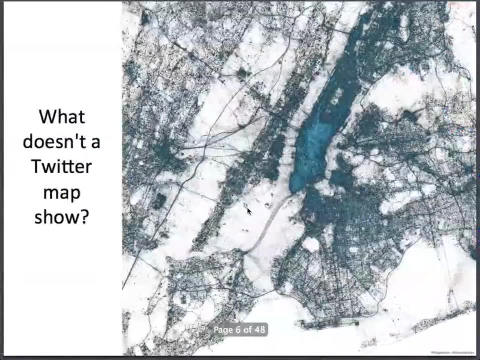 the Twitter map Brooklyn's pretty sparse. Is that some bad service? Yeah, that could be it as well. And the other thing you notice is there's this correlation: the densest parts of the Twitter map are also the richest parts of the city. 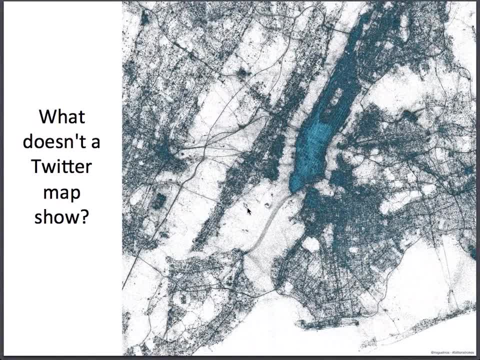 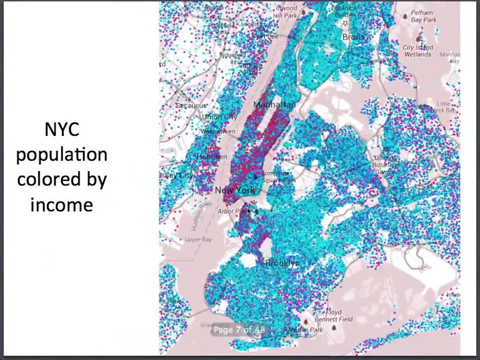 So if you want the Twitter map to stand in for all people, it doesn't, It's going to be systematically off. So these are the sort of questions in data interpretation that you need to ask: not only what's there, but what's not there. 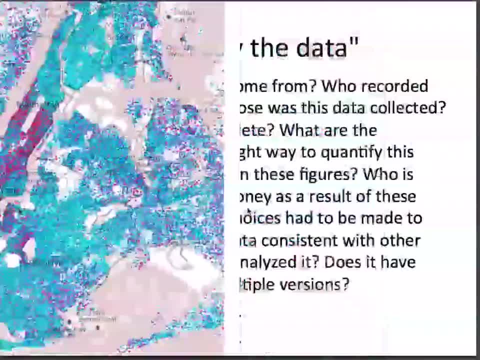 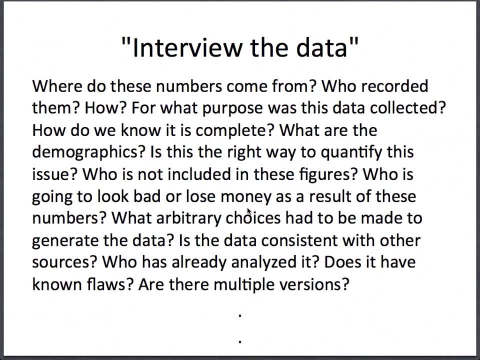 And there's come to be this phrase in data journalism, which is interview the data and treat it with as much. what's the word? I guess respectful skepticism is maybe the way you would treat an interview subject, Because there's just so many reasons. 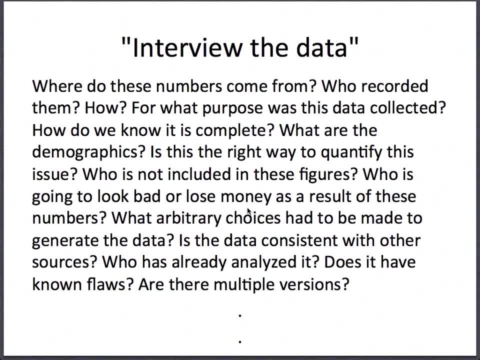 There's so many reasons why it doesn't. it's not going to mean what you think it means, And some of them are innocuous. data is always collected for a reason. That reason may not be the reason that you want to analyze the data, or you may not even. 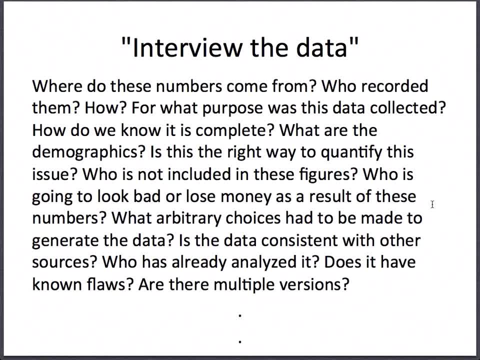 be collecting the right thing right. So if you want to look at gun availability, well, how do you measure whether somebody has access to a firearm? You can count the number of gunshots. You can try to estimate the number of households that have guns in them. 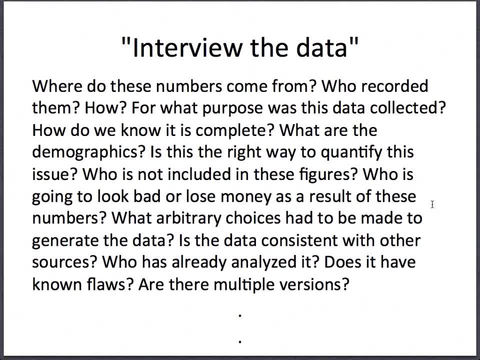 You can look at the fraction of suicides that are by firearm, which is actually thought to be the best possible indicator. But this sort of hazy concept: how easy is it to get a gun? there's lots of different ways you could measure that, or try to measure that. 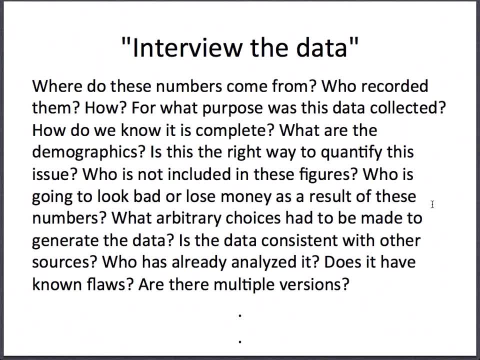 And each way is going to give you a particular bias. So you have to think about it. Think about that. What am I collecting? All of this is prelude, because I think this is relatively intuitive for journalists. We're used to asking these types of questions and there's a few of them. 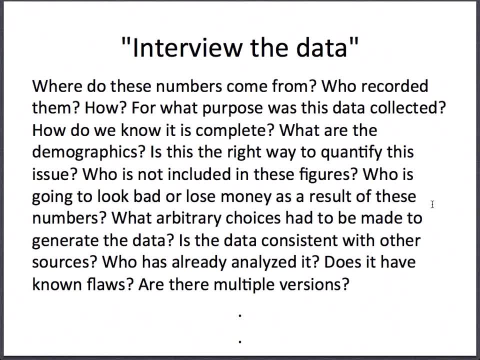 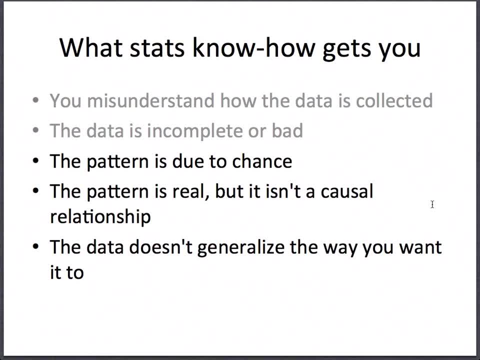 Demographics doesn't normally come up when you're talking to an interview subject. But now we're going to get to statistical testing and we're going to talk about these other problems. The main thing we're going to talk about is chance. How many of you have done basic probability or randomness? 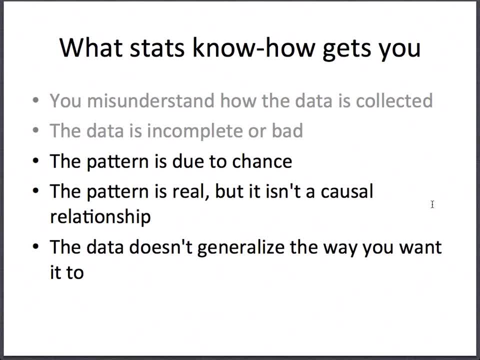 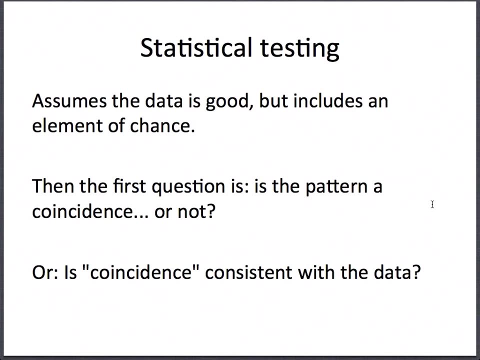 If I say probability distribution, how many of you does that mean something to you? All right, good, So we know where we're starting from. Let's start with rolling a die, a six-sided die. Oh, The first question we're going to deal with is: is the pattern I'm seeing by chance? 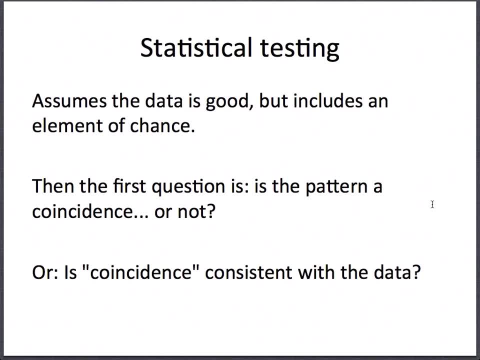 So let's take our examples. We look at our school grade data. We see that smaller classes have higher grades. We map cancer cases and we see that they're higher near the oil refineries. We look at tax rates versus industry. There's all kinds of relationships we might want to look at when we're exploring this. 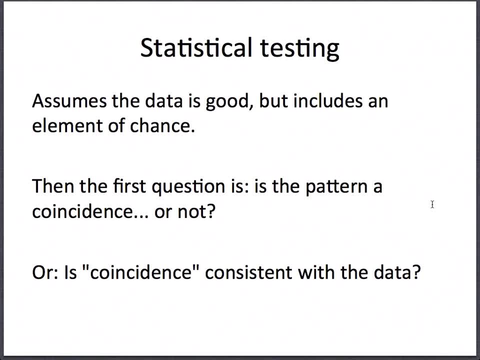 type of information. All right, All right. So let's say, we do use the four-sided die, But there can be patterns by chance, And patterns by chance are a lot more common than most people would suspect. So I'm going to try to build up an idea of what chance looks like for you. 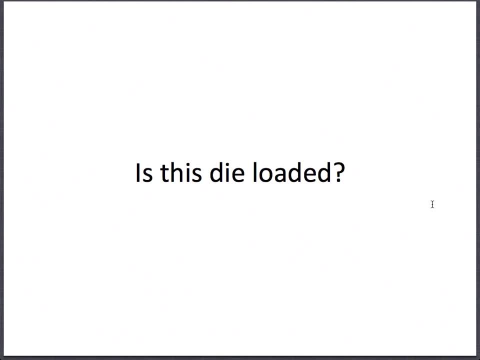 And again, we're going to start with a die and we're going to start with a fictitious story. You're a journalist. suspicion is that the die that is being used for I don't know craps is loaded right. 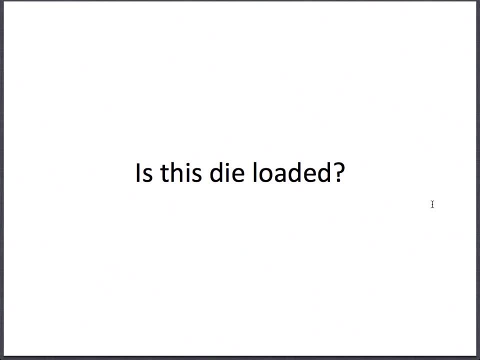 So it's weighted so that one of the die always has a 1 with much higher rate than you'd expect. So if I gave you a die and I handed it to you and I say, is this die loaded, Tell me? How would you find out? 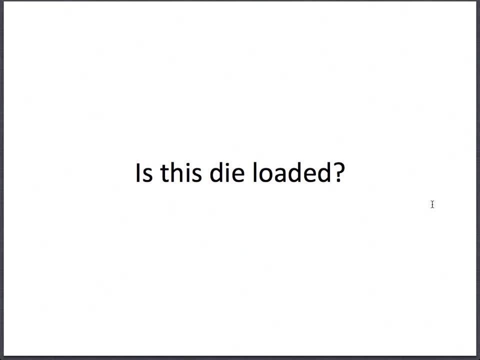 Right the number. it's unusual if the same number comes up more than the other numbers, Right? so you roll it and you- Over two times, six times, four times out of six is the same number. It's weird, So you roll it six times and four of those times. 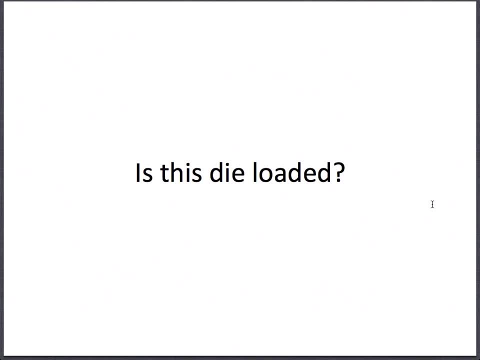 it's a bigger number. Is that good evidence? Many more times, OK. how many more? 100?? I mean, the more times you replace them, the more you do it, the more you do it. You probably look up the probability. 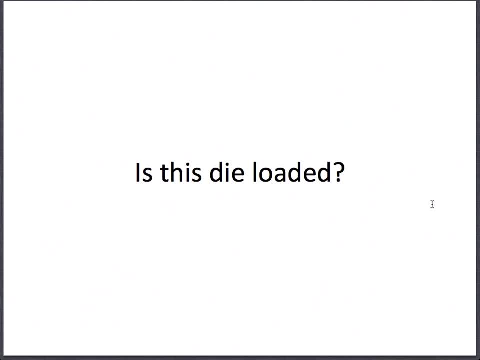 of a six-sided die online and see what the various probabilities are, But once I'm at a point where I'm rolling, I'm really overpaying the probability of getting one now. Yeah, so your intuitions are right. You want to do it a number of times. 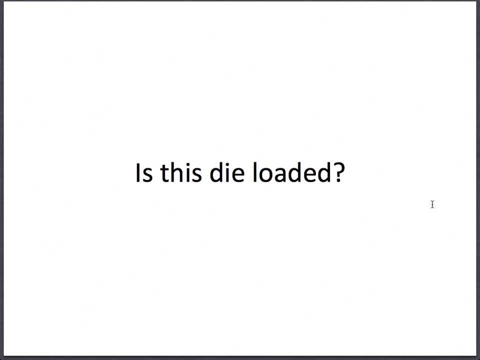 We're going to talk about how many more, and we're going to talk about what rolling a six-sided die should look like. So if I roll a die 60 times, How many times should each number come up? 10 times, Let's try it. 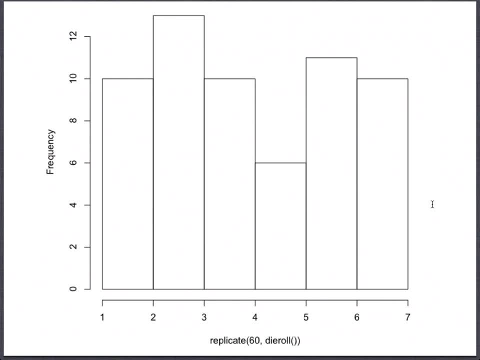 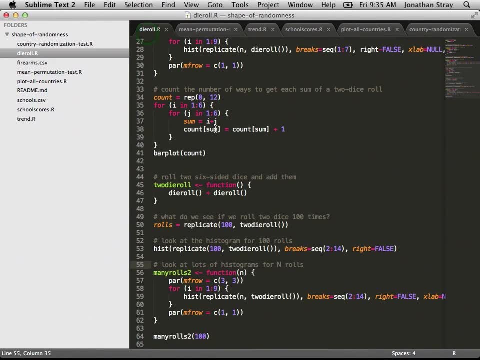 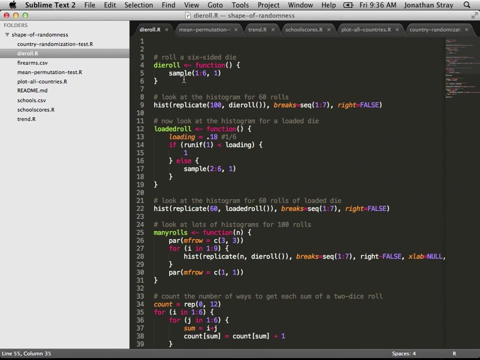 There's a chart that I made by rolling a die 60 times. In fact, we're going to start the interactive portion of the class here. Don't freak out. This is a language called R. R is a free piece of software for statistical testing. 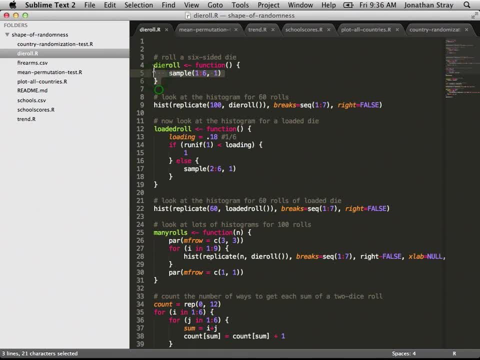 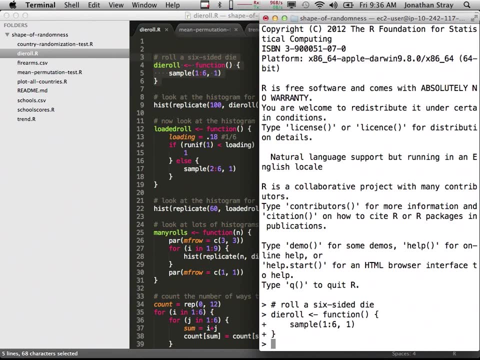 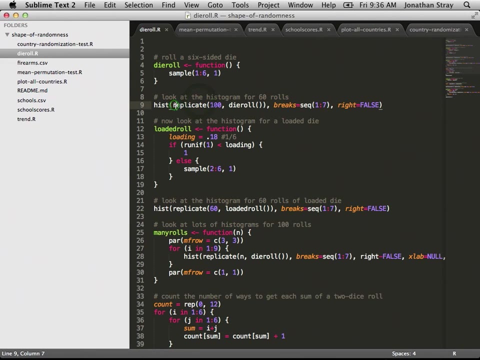 I'm going to roll a die 100 times and show you what it looks like. So first there's this little function that just rolls a die. So if I just say die roll, it gives me a number. If I say, do it 100 times, there we go. 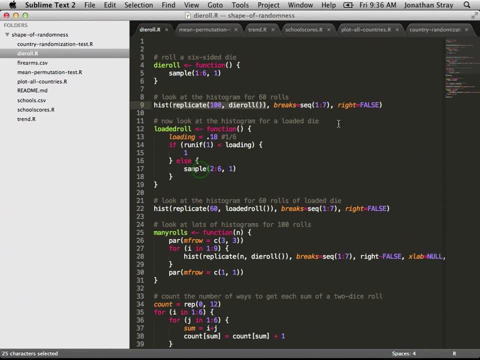 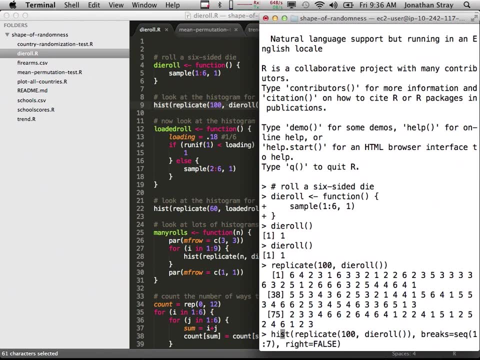 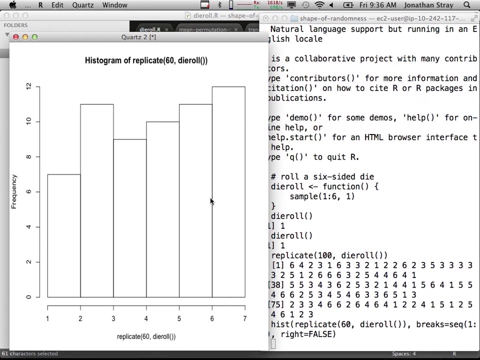 Gives me all these numbers And then I'm going to make a little histogram of them. You know what a histogram is. It just counts, right. It just counts how many times each number appears. There we go. There's rolling a die 60 times. 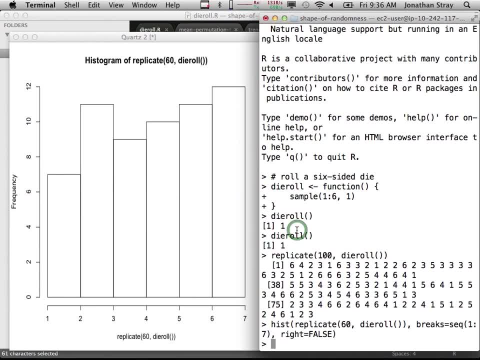 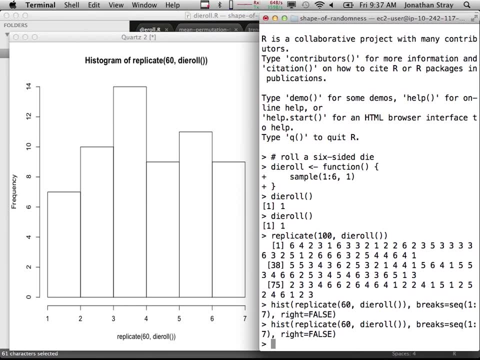 Does that look like you'd expect it to? All right, This one I only got seven times. How about this one Got a lot of threes? Yeah, Is it a suspicious number of threes? No, Not quite. How many threes would you have to get before it was suspicious? 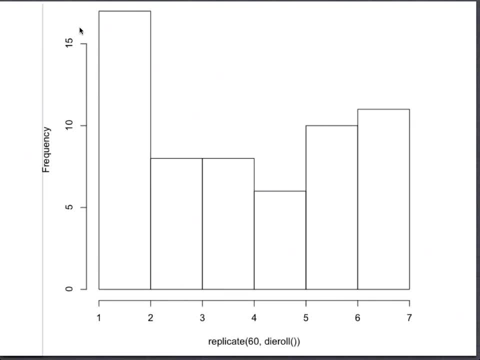 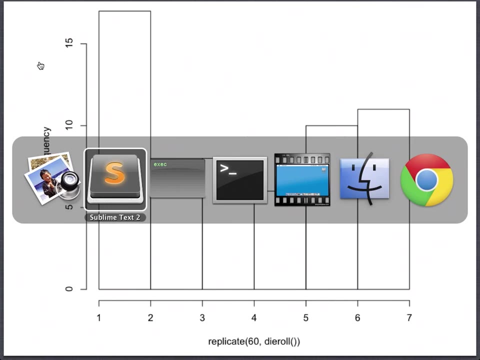 What if it looked like that? Is that suspicious? Why is that suspicious? Yeah, Yeah, That's possible. Yeah, Yeah, Yeah, Yeah, Yeah, Yeah. So let's try this a few more times, though I'm going to go to R again if I can find it. 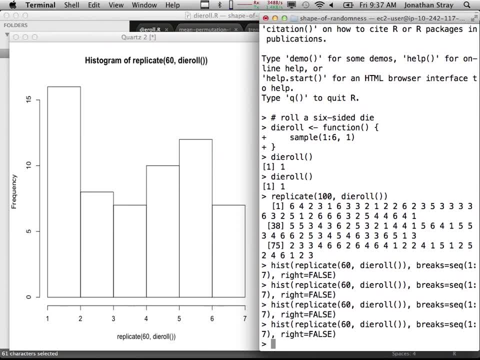 I'm going to keep It's random. It is random Exactly, You know. So I mean, yeah, sure, I mean I guess statistically it would be you know six chances to get you know, But I mean randomly, you know, I mean it could be. 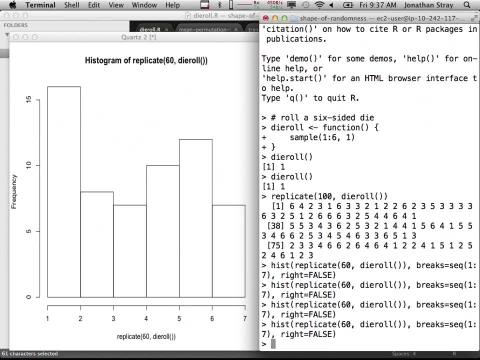 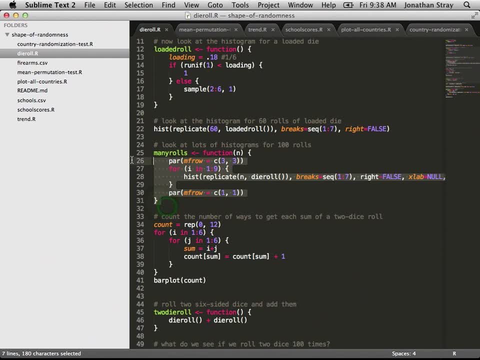 It's like: what are the odds that that could happen? Yeah Right. So what I'm going to do now is I'm going to- actually we're going to try to estimate What are the odds. I'm going to make a little function. 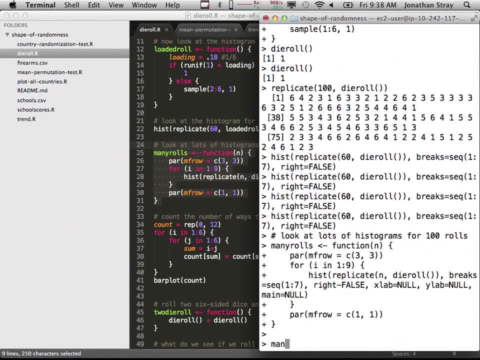 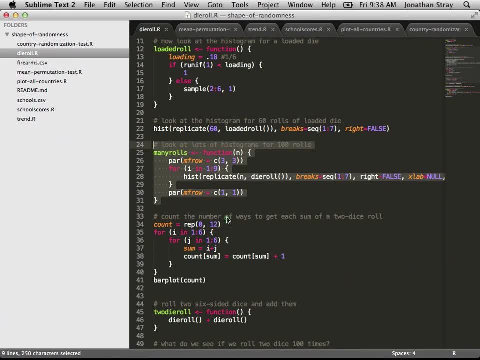 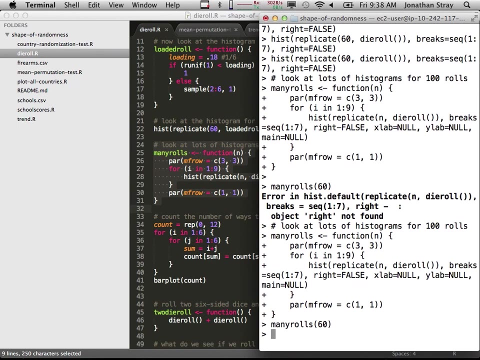 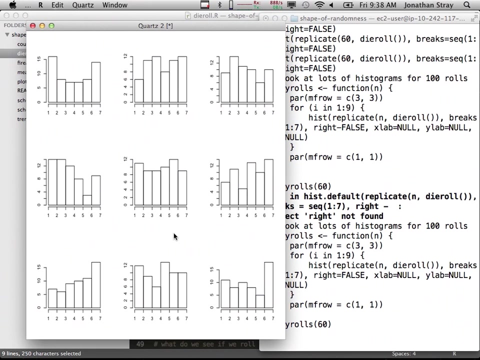 that plots many rolls as ones- And I'm going to say many rolls of 60- die. Oh god, What happened? There we go. We've got debugging on the fly, All right. So here's nine rolls. How many of them, would you say, have an unusually high? 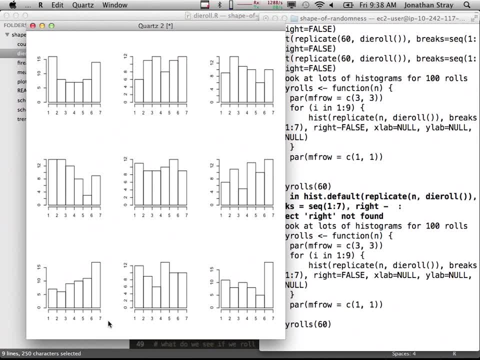 something that has an unusually high weight on one number. Maybe that one and that one. Yeah, So two out of nine. Let's do it again. How many of this one? Isn't this the one that? Yeah, I mean some bites can have a lot, some don't have any at all. 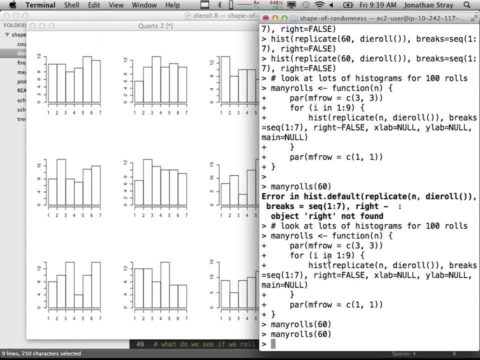 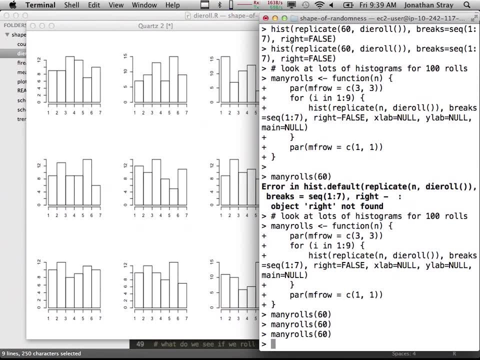 Exactly, But the question I'm asking is: how often do you get a bite with a lot of blueberries Right? That's an actual number, though, Because the question I want to ask is: how often does chance look like a pattern? 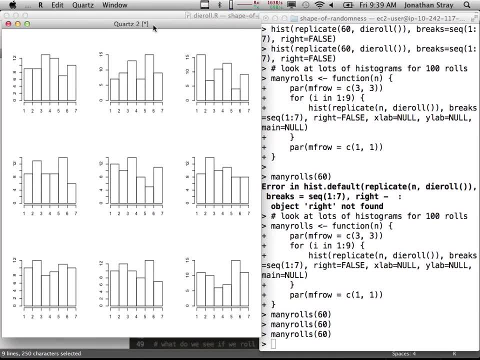 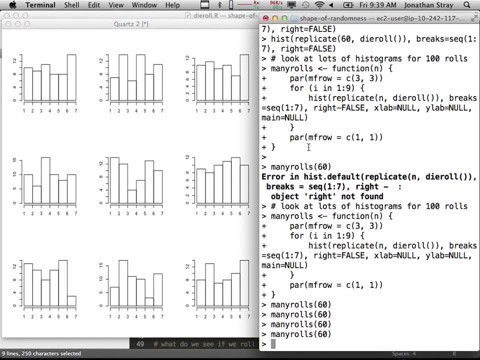 And so if I give you one of these histograms and I say, does this look suspicious to you? Either the die is actually loaded or, Yeah, It happened randomly. And here's the central core of the argument we're making this morning is that if you 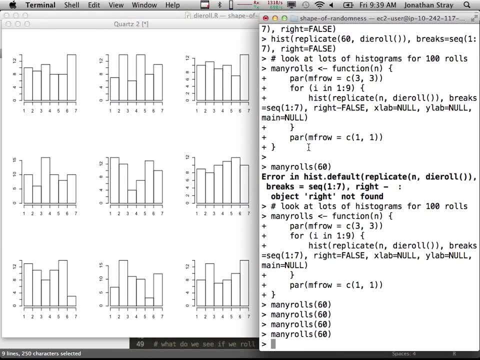 can prove that the pattern that you're seeing only happens very rarely by chance. that's evidence that it's a real pattern. That's the core idea of all of the things we're going to do today. So to prove that it's rare, the first thing you have to do 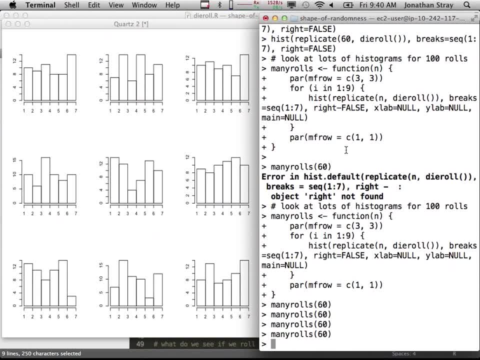 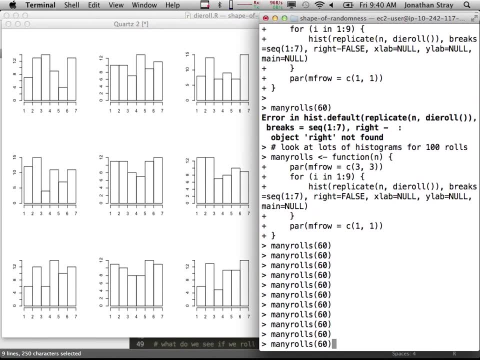 is you have to have some idea, Yeah, Of how often it actually happens by chance. So that's all we're doing here is I'm just trying to calibrate your intuition of how often, if you roll 60 die, it's going to look like the dice is loaded. 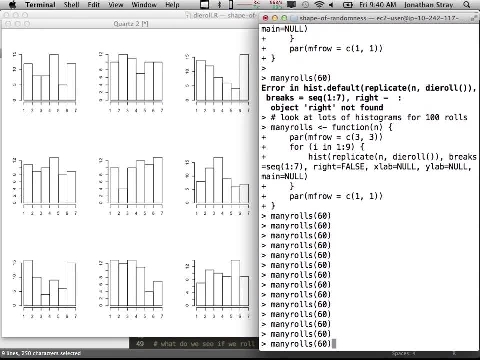 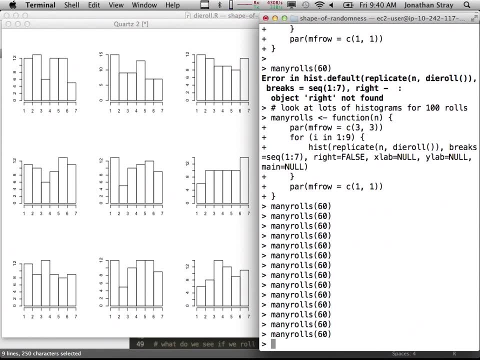 I'm thinking it looks like one or two out of nine here, right? So let's call it 10-ish percent. So that means if you walk into a casino and they let you roll, that die 60 times and you get something. 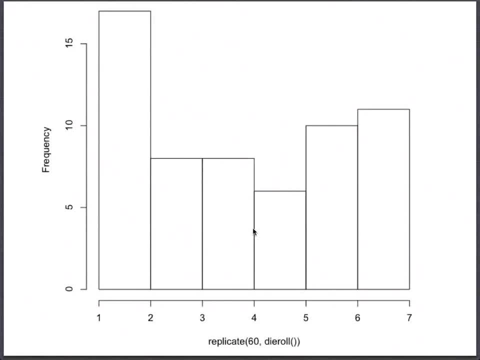 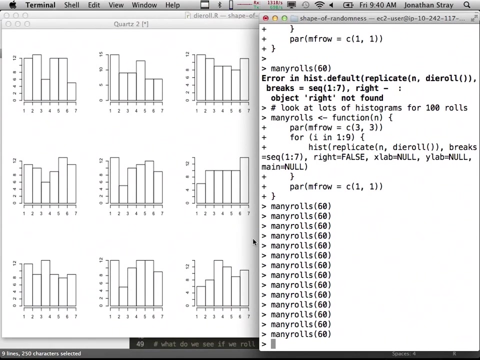 that looks like this and you're like, well, shit, this die is loaded. I got a story here about a gambling scam. What's the chances that it's actually just random? Well, about 10%, right, Because we just said that, if we're going to do this, right. 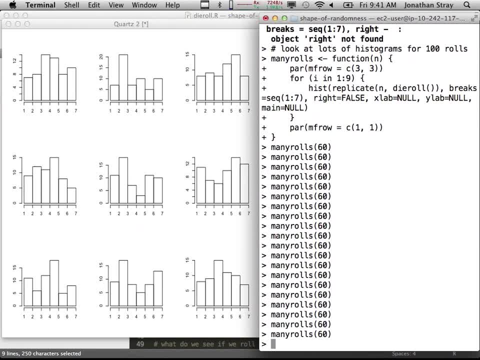 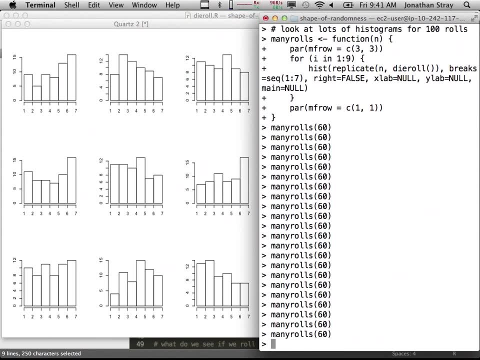 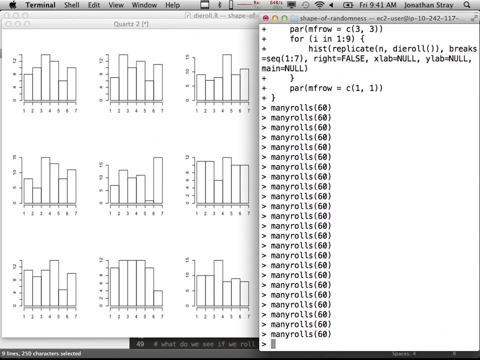 How often? So the question I'm asking is: how often does a random pattern look like something is actually there And we can do it just by looking at it a lot and sort of counting You with me so far? So a few other things. 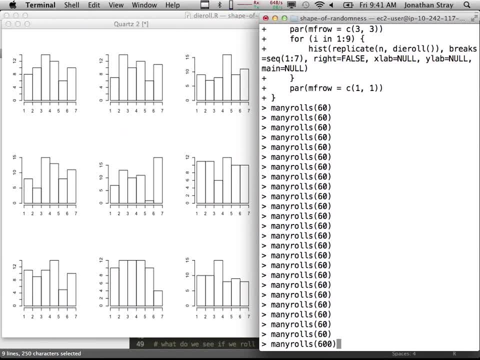 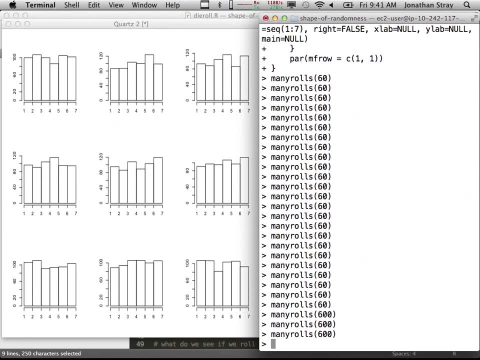 This is something that someone alluded to earlier. Now I'm going to roll 600 times. What's different? no question It's. you roll 600 times, then I get this. Yeah, so they're flattening out. Now they're looking more and more uniform. 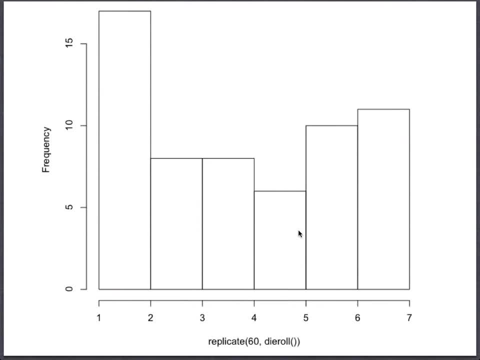 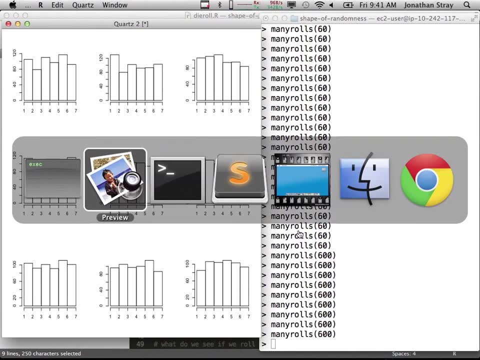 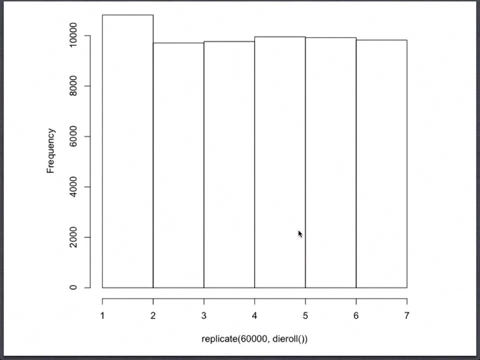 So now, if I roll 600 times and I get something that looks like this, am I more suspicious or less suspicious? More suspicious, OK, So this is a basic statistical idea, which is that that you used the word error. the statistics term is variance. 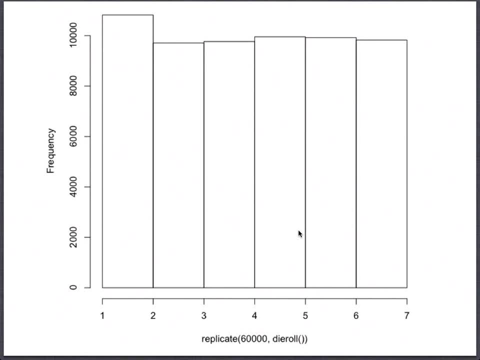 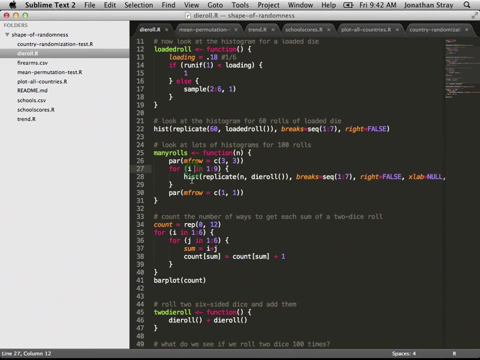 It's what is how much. I mean it has a technical definition, but the intuitive definition is: what is the spread of numbers that I'm gonna get when I try multiple times? I actually have here a loaded die, and so let's play with the loaded die a little bit. 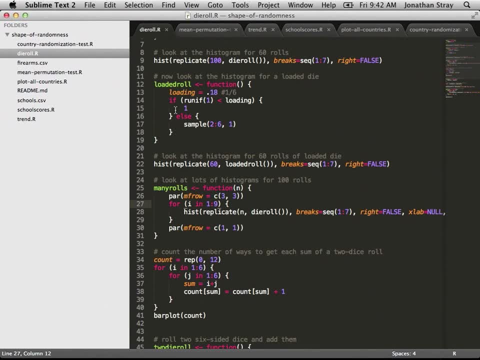 Can I ask you a question? Yeah, How do you figure out how many times you don't get to hear from 60 to 600? We could go to 6,000, 6 million. How do you know? how do you try to figure out? 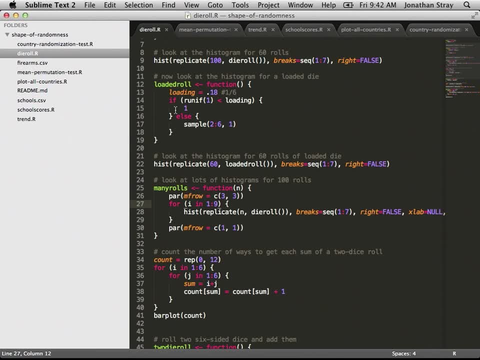 how many times you have to go before you can get an answer. I mean, maybe 6 million is unnecessary. Yeah, You don't get an answer before that, so how do you know what that one is? So, if you're so, the short answer is: there's formulas. 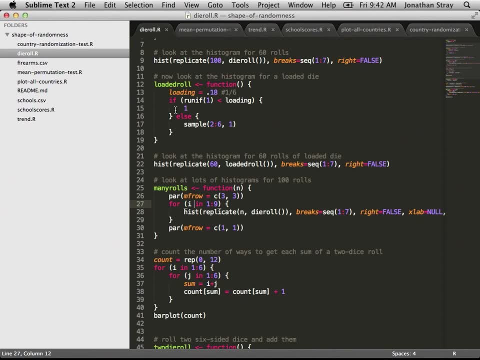 You can work it out. The longer answer is that in your case, normally as a journalist, you won't be generating the data. You've got data as given and you have to figure out whether you have enough of it to draw a conclusion. 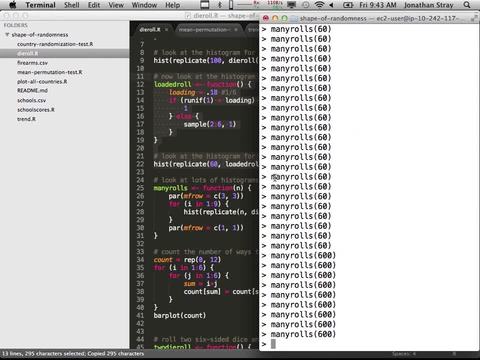 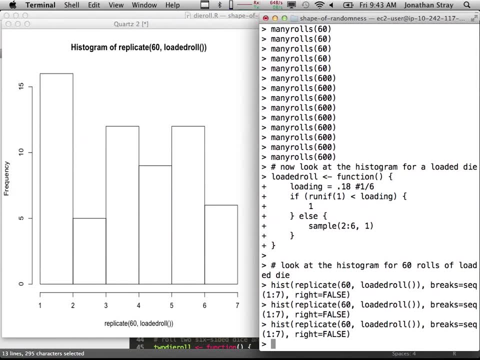 I'm going to play a little bit with a loaded die and I'm not gonna tell you how loaded it is, although you can actually read it right off the screen there if you were looking closely. So I'm telling you this is a loaded die. 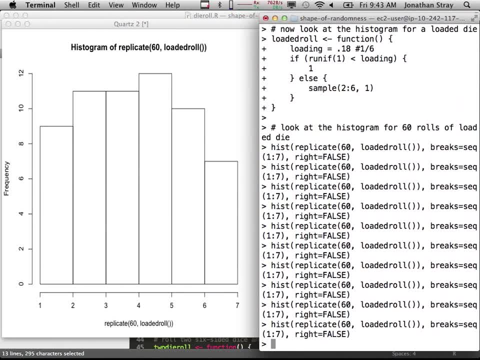 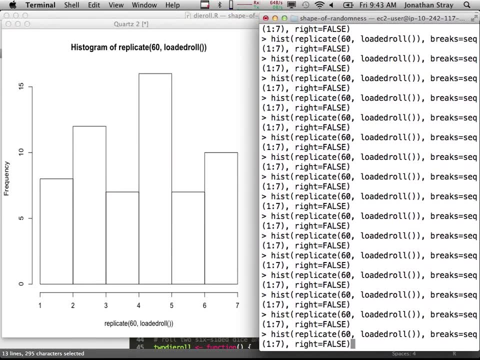 Tell me which number you think is loaded. I'll show you a lot of these. Does anyone have a guess? Number two: someone said four. What's really going on here is we're not rolling it enough to know, But now I'm gonna roll it 600 times. 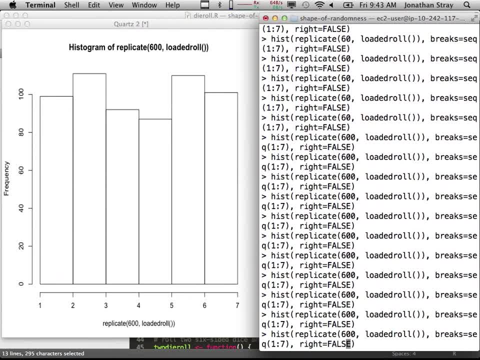 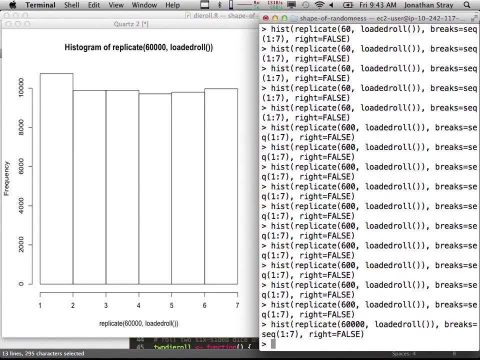 Anyone got a guess? now, Number one: Now I'm gonna roll it 60,000 times, So we should get 10,000 rolls for each die. I'm gonna roll it in, but I'm not gonna look at it. Yeah. 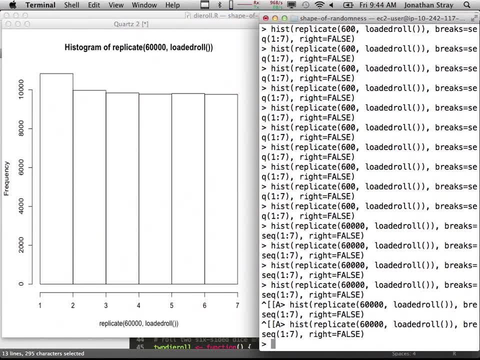 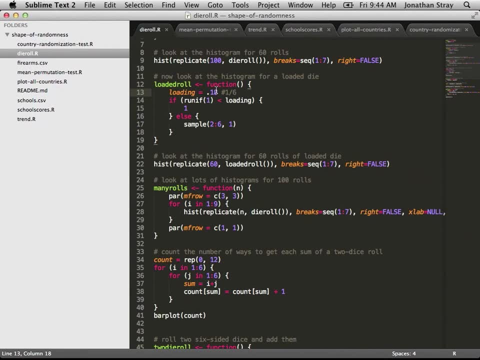 So there's two different concepts here. One is how much it's loaded by right. So a little bit excess there. in fact, What I've done, if you look at the code, is I've said it's gonna land on one 18% of the time. 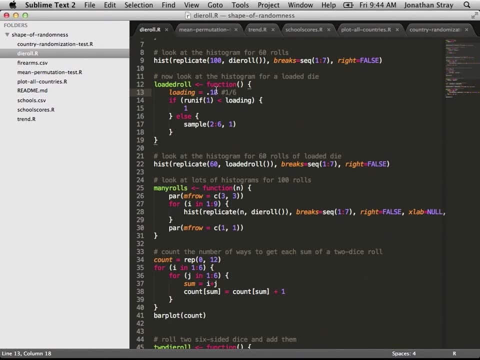 If it's a six-sided die, it should land on one about 100 over six, which is about 12% of the time, or 20%, my math no 16.. So it's just a few percent over and the smaller the difference. 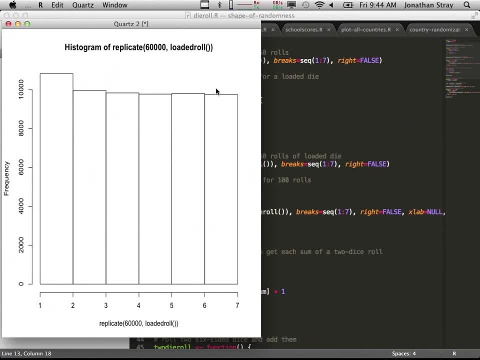 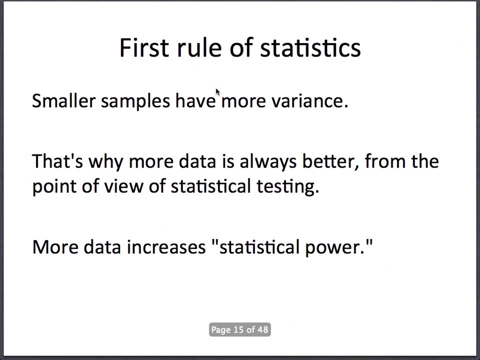 you're looking for, the more data you need to find it. So I've now, I've now tried to demonstrate to you that the very first thing you need to know, which is more data, gives you more certainty that what you're seeing is really there. 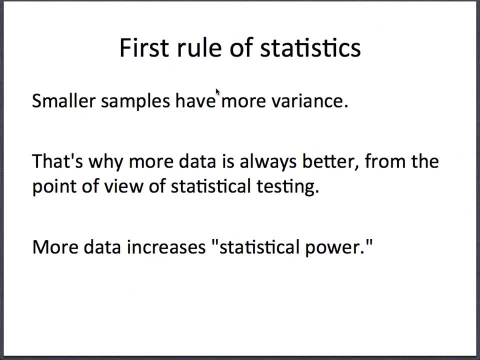 and the smaller the effect you're looking for, the more data you need to find it. If the effect is huge, right so say you plot your oil refinery data and census. blocks within a mile of the oil refinery have ten times the cancer rate. 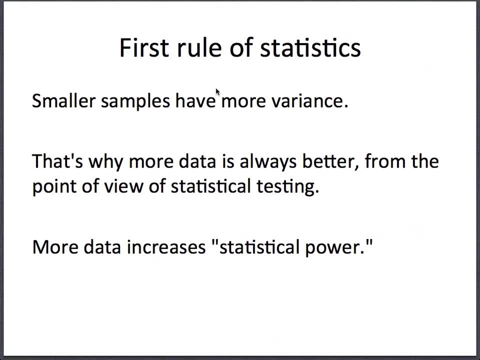 of ones that aren't. If you're starting to look at that level of significance, you know something that's that big an effect. you don't need very much data, right? Maybe you know if you have ten cases of cancer instead of one, but if 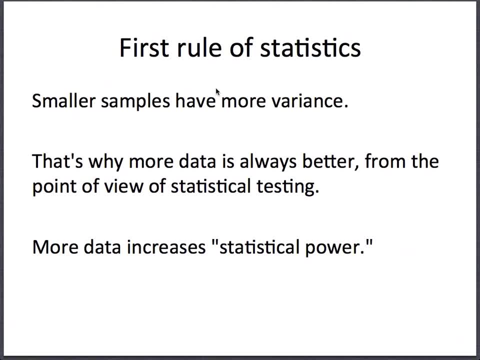 you have, you know, three cases of cancer instead of two, right, exactly. So which types of cancer are going to be hardest to link to the oil refineries? Oh yeah, so the time lag is a really important thing too, but statistically is. 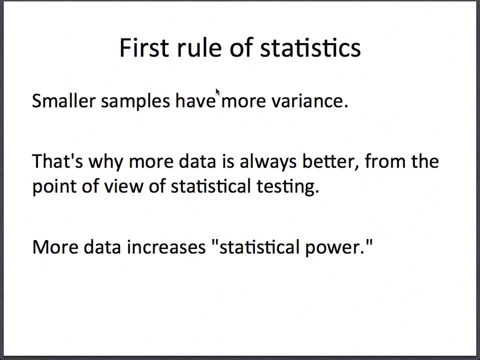 it going to be the rare cancers or the common cancers that are going to be hardest to Now? the common cancers are going to be easier because you have more roles of that done. does that make sense? It's the rare ones. If I'm looking at a difference between 10 cases and 100 cases, that's pretty good evidence. 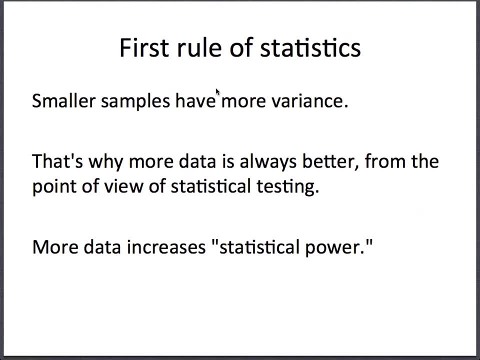 And we'll get to just how to tell if it's good enough soon. If I'm looking at three cases versus two cases, again, think about rolling that die. How often will I get three versus two? So the rarer the events you're looking for, the more data you're going to need to reach. 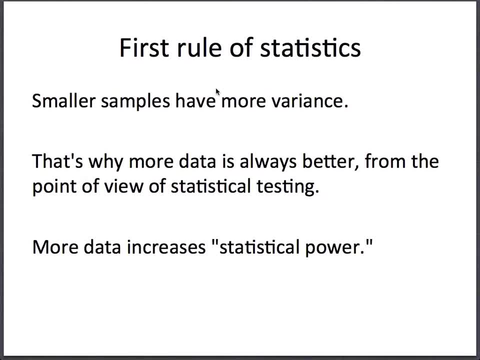 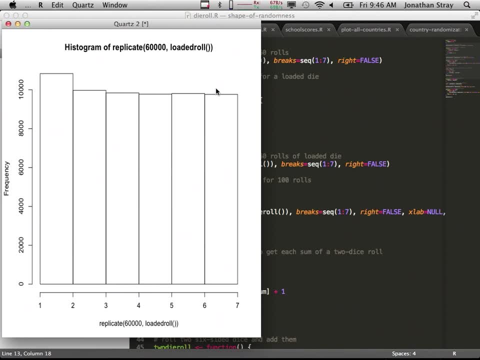 statistical significance, Just like our loaded die example. Sorry, If a rare cancer, then the fact that you have, you know, even if you're talking about 10, but if a really rare cancer, where are the chances that they have exactly the same place? 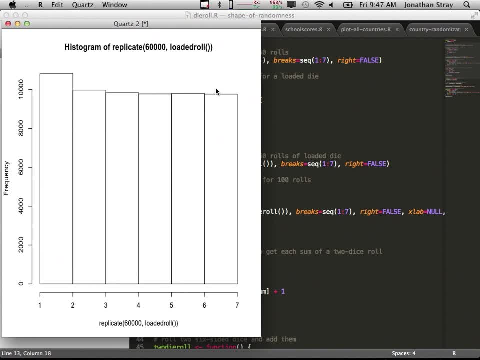 I mean, shouldn't that be considered? If they're rare, they don't, huh, No, but I mean, you don't, But if they, you know, even if they're rare cancer, if you have a small, even small concentration, 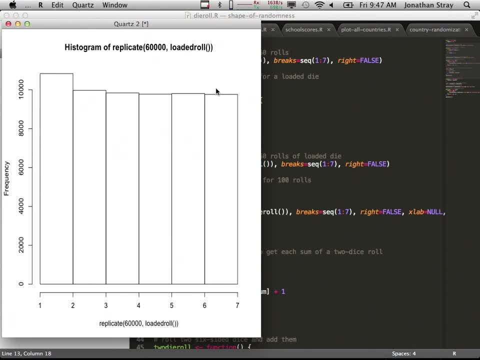 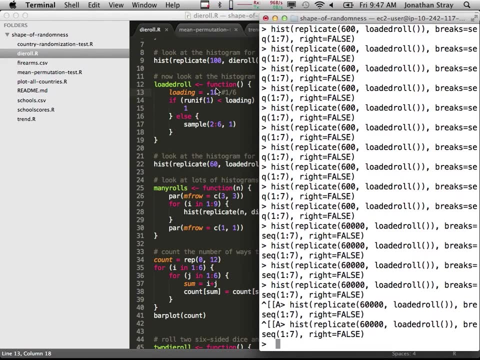 but you know generally would be one, and then you suddenly have 10 in the same place, which is really a refinement. wouldn't that be an indicator that there's something wrong? Well, the problem with rare events is that very commonly it will look like there's something. 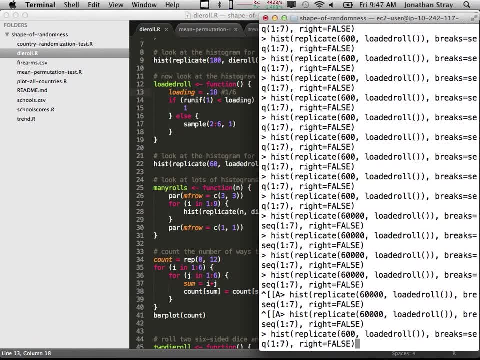 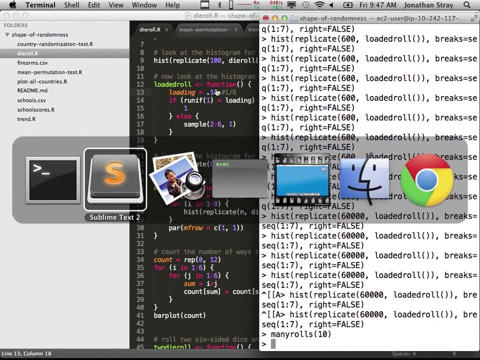 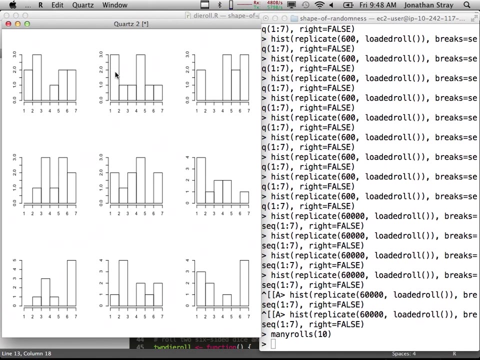 wrong when there's not. So again, I'm going to go back to our again the. let's look at our die roll for a second, Okay, Okay, Okay. So let's say that the number one corresponds to. let's say we're looking at the number. 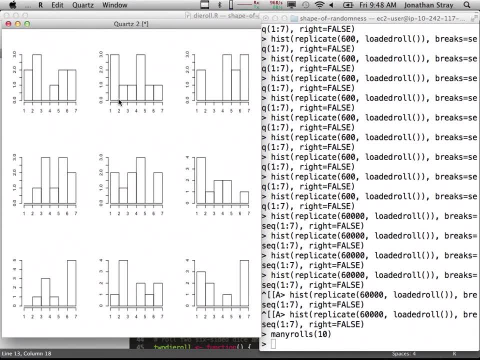 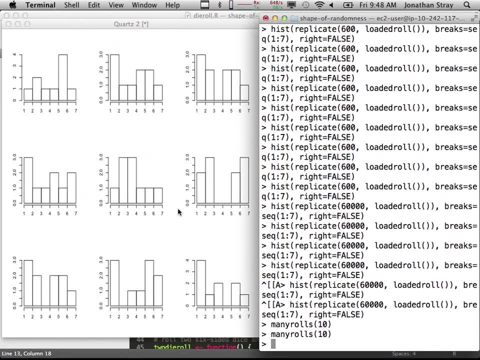 of cases of a rare cancer in different counties, and number one is the county that the refinery is in. If I only have 10 cases overall, how often am I going to see? just by chance? just by chance, let's say that the cancer rate has nothing to do with the 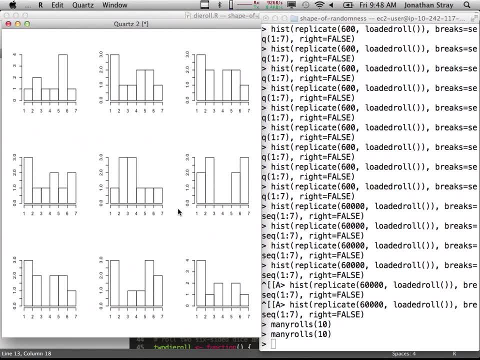 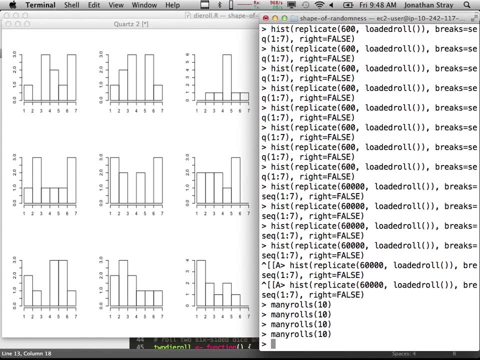 old refinery. let's say it has to do with diet. How often am I going to find, just by chance, that there's a lot of cases in the county with the refinery right? There's only 10 cases in the whole state. Okay, so there's one right That looks like there's the highest number of. 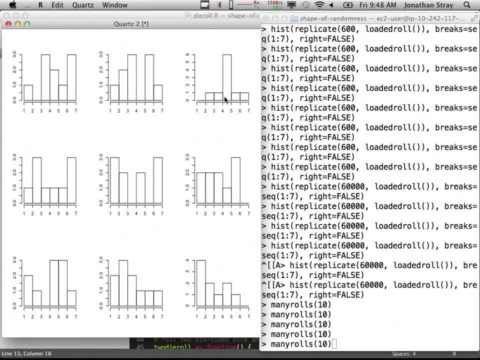 cases in the refinery. Let's take this one. let's take this one right. Look at that. If you get that data, you're like, wow, There's six cases in the old refinery and no more than one anywhere else. the problem is, about half of these graphs show that kind. 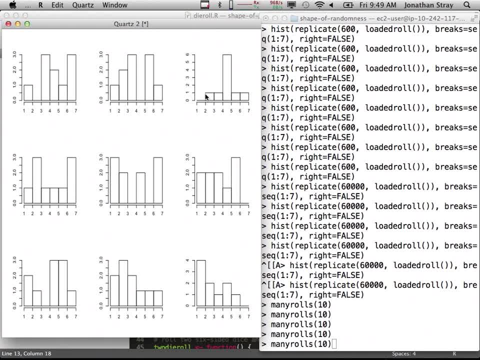 of pattern. So the problem is: how often do you из a year what is was your average? rarer it is, the harder it is to separate chance from effect. That's the problem. Does that make sense? Whereas if I roll, if I start to roll a hundred times, then the 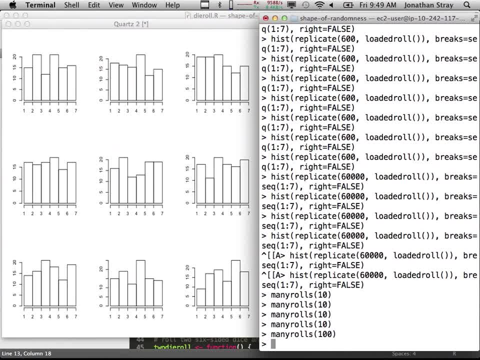 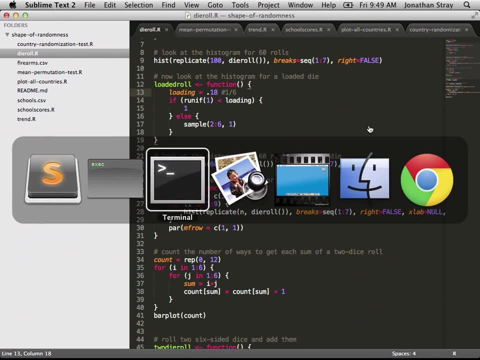 graphs sort of start to even out. So if I get that big spike when I have a cancer, that's there's a hundred cases in the state instead of ten. it's much better evidence And we'll get into how much better evidence in a minute. Okay, What if? 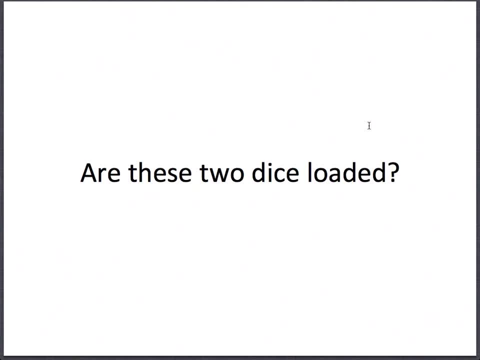 I want to look at two dice. If I rolled two dice and I, you know, look at the numbers that I can get, how do I? what should that look like? Anyone, anyone, a gambler here? Gambling will help you a lot in stats. No, seriously, that's where. 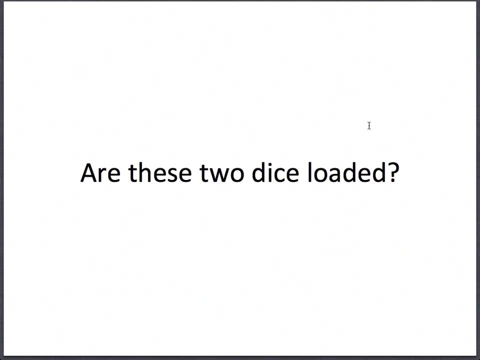 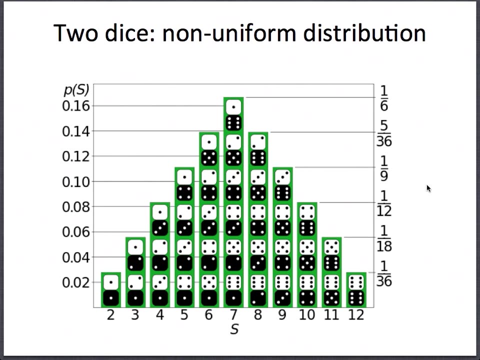 the science is. That's where the subject started. Probability theory started in the 1600s with games of chance, And the fundamental intuitions all come from these types of gambling ideas. So to figure out what it should look like, I'm going to take these: 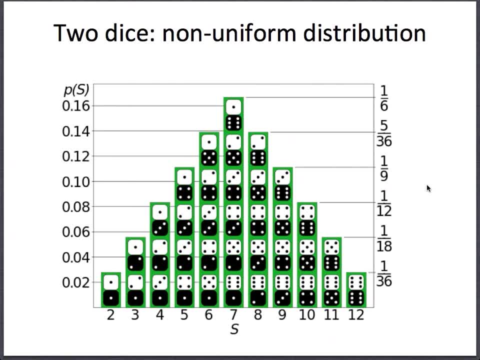 two dice and I'm going to count all of the different ways they can land. The first die can be any number one to six. the second die can be any number one to six, and then I'm going to take their sum And you know, in the middle here are all the 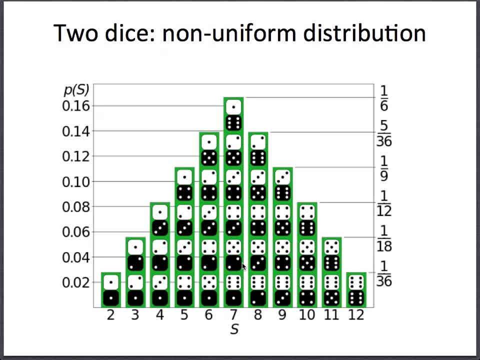 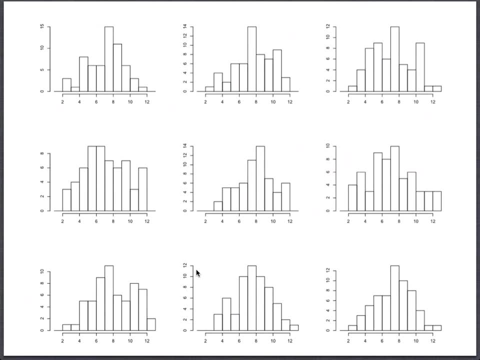 different ways. I can sum up to seven, And so when I roll these two dice, I should get a pattern that looks like that. What do you think I'm actually going to see when I roll the die? Is it going to look like this shape? No, It looks like that. Here's. I think that's a 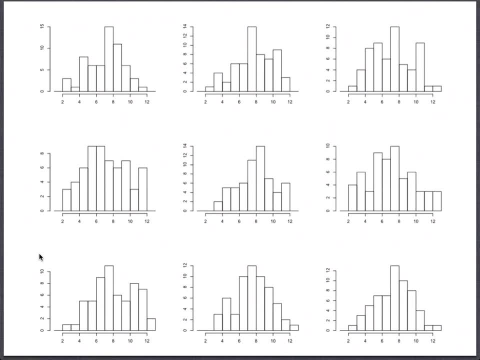 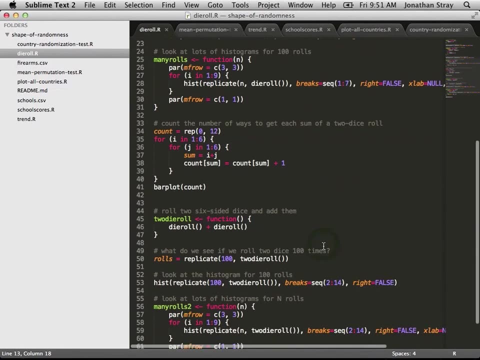 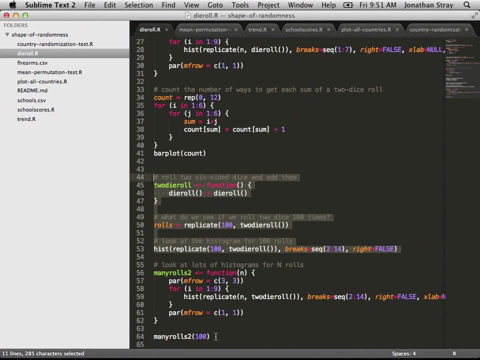 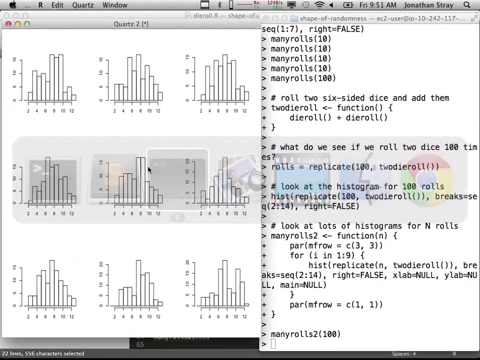 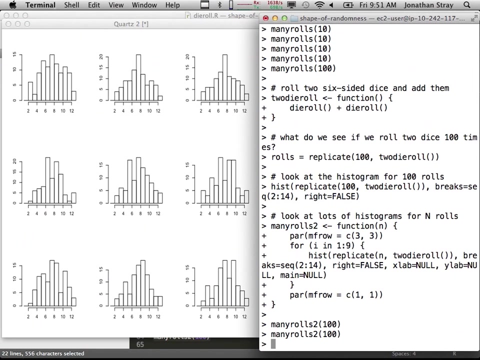 hundred rolls again. Sometimes I get that shape, sometimes I don't. And again, the more rules I make, the closer it's going to get. so I'm actually going to do this for you really fast. I can't imagine the scenario that I'm 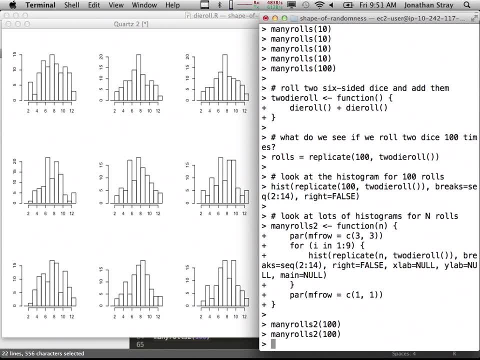 going to have time to do my own data like this, mm-hmm. so are you? I mean I'm just: is this a? is this a way for us to learn, or for me to learn, how to better interpret data that I do get, and whether it's? 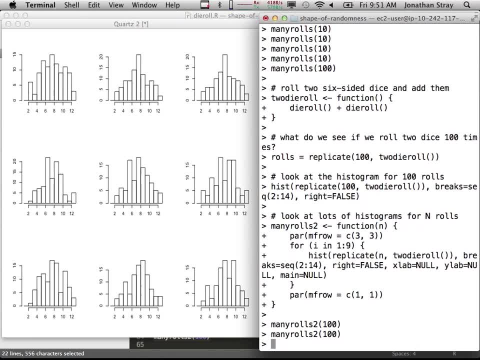 statistically significant, or whether it's just somebody who doesn't have an idea. it has a preconceived notion of what they want to achieve and and that's what they're showing me versus some significant. you know some real data that I want you to come out of this with it, with an 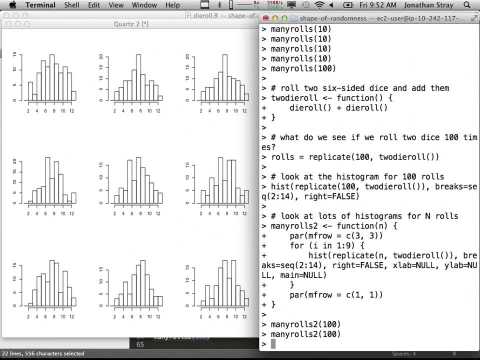 intuition about what statistical testing is. okay, I want you to understand the logic of it. okay, that's what I'm getting at, which is why I'm sitting here showing you die rolls, because to understand the logic of statistical testing, you have to understand the logic of chance. because 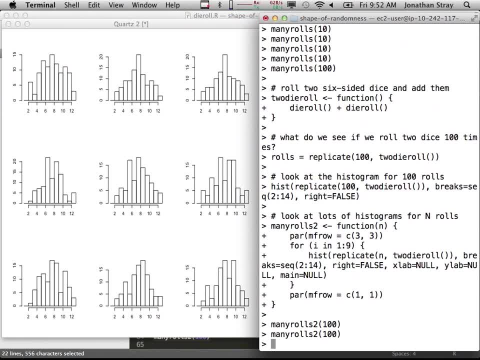 statistical testing how it works is you compute the probability that what you're seeing happened randomly. if that is low, you say, well, I don't think this is chance. and so I want you to be able to read a scientific paper or look at data and I want you to say: you know, be able to look. 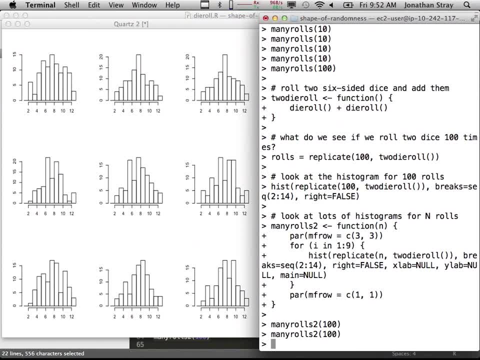 at and say 20 cases, that's not very much. you see, how often is 20 cases gonna look? look like that by chance, I see, and you know, if you have 20 cases of something and you're saying all of them occur, you know, next to the refinery, for example. 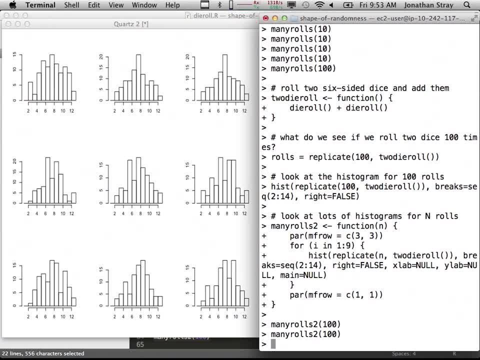 that's going to happen like 30, 20, 30 percent of the time. all right, so it's a way to be better at interpreting the data exactly and I'm going to have to follow exactly the die roll guys. they're just, they're getting a probability of. 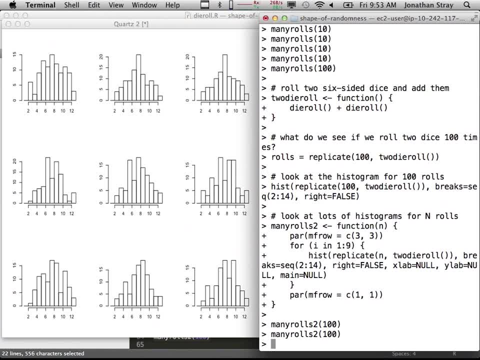 the numbers and betting with the probability and figure it out. well, I'm going to win a certain percentage. I'm going to win a certain percentage right, but only if they do it a large number of times. right and the number. so we all know, we all have this intuitive 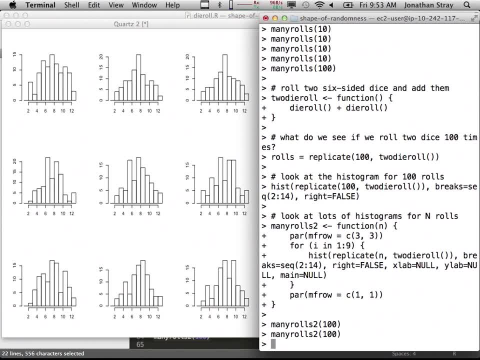 sense it's actually called the law of large numbers and it was worked out in originally in the 1600s by Bernoulli and it says that if I rolled, you know, do something, roll the die. but roll the die stands in for something happens with an. 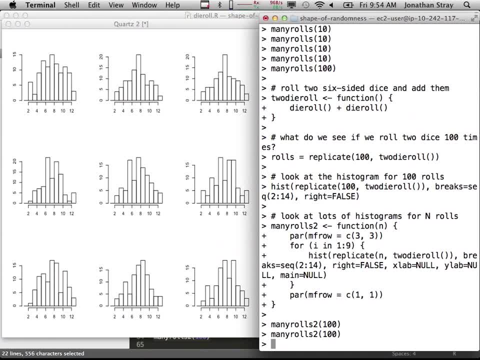 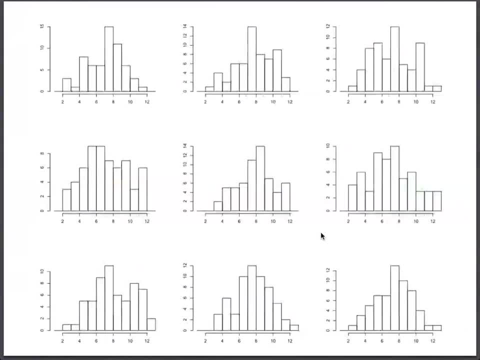 element of chance. many times over time it's going to average out to some pattern and we can count, calculate what that pattern should look like, because we can. we can do this right. we can do this, this theoretical analysis of what it should look like. but it doesn't look like that until you get a. 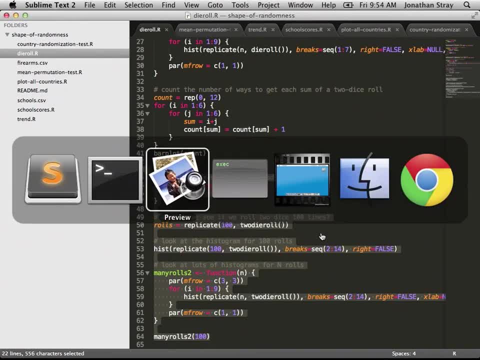 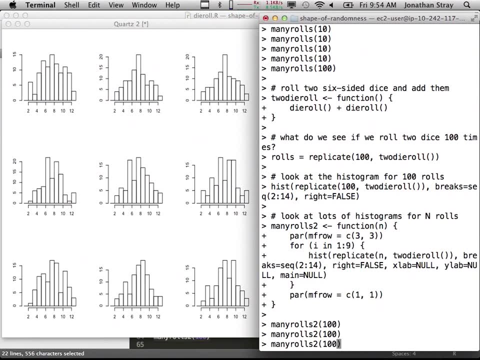 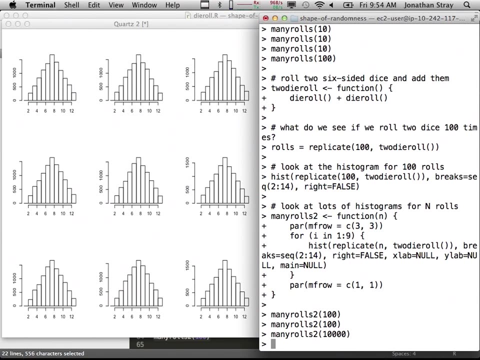 very large number, and the one I'm trying to give you a feel for is how big. all right, so that's a hundred of them, and we've still got, you know, all these funny shapes. if we get 10,000, that looks like what we would expect theoretically. 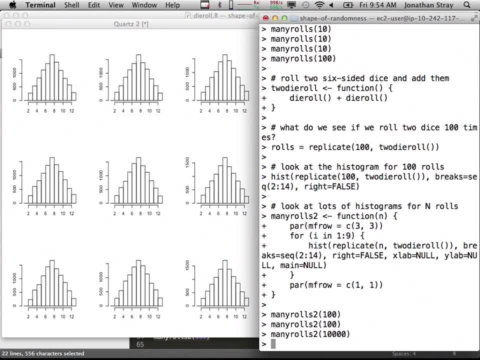 is that all, yeah, okay, so, and- and I'm actually going to show you a very simple statistical test- that that you can actually do as well, or maybe you can ask your friendly newsroom coder to do- let's, let's, let's ask actually that how many of you work in an organization where 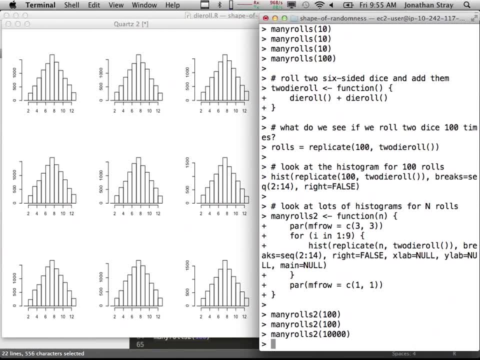 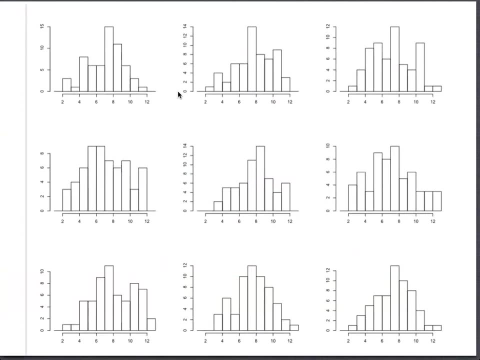 you have a journalist on staff- a little bit of a coding system skill- who can help you with this analysis. all right, so about half that's good. the the public talk is going to be about what that job is and why that intersection is interesting, so we looked at that. who's heard the phrase? 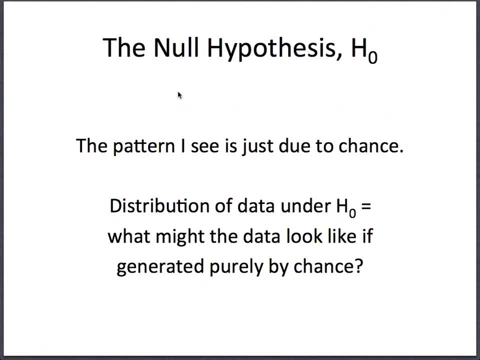 null hypothesis. we've got one, okay. so if you're doing any kind of science, you're going to come up with a hypothesis and you're going to test it- statistical and statistical testing. what we're trying to do is we're trying to choose between multiple hypotheses and we have at least 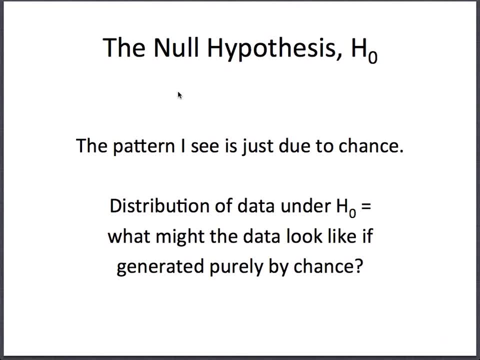 two. one is what we see happen by chance. there is no link between class size and school grades. one is what we see didn't happen by chance. smaller class sizes cause higher grades. the it happened by chance is called the null hypothesis, usually in in in scientific writing. 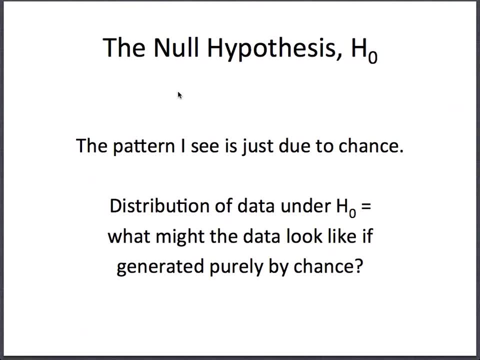 you'll see that as h0, and we've been, we've been plotting this little graph, like you know what, what the die roll looks like. when you roll two die together, that's called a distribution, a probability distribution. right, that is, if I do this many, many, many times, what? 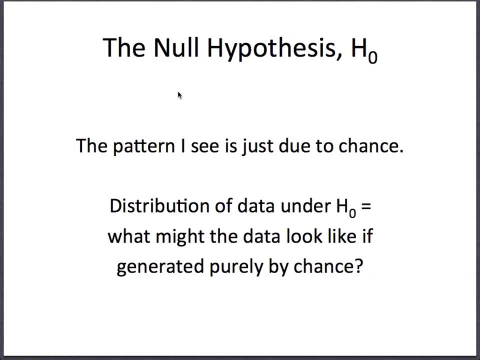 is it going to look like, but many means like 10,000, and you don't usually have 10,000 different classes with different teachers. right, you have every school in the city and maybe that's only 30 schools, and so, although there's this theoretical, 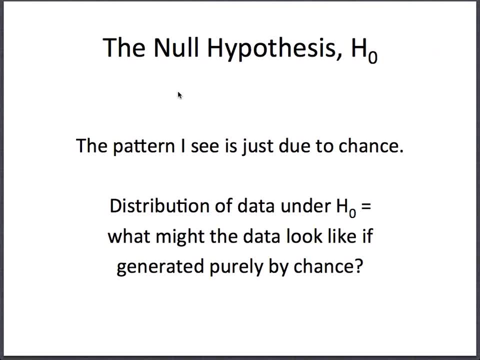 distribution. what you're actually going to see is something much more patternful, and so the question you have to ask yourself is which hypothesis is true, the null hypothesis or the alternate one, where I do think class size is there, and so you'll see, this is terminology, this 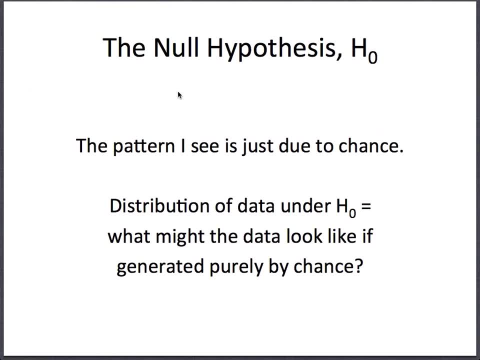 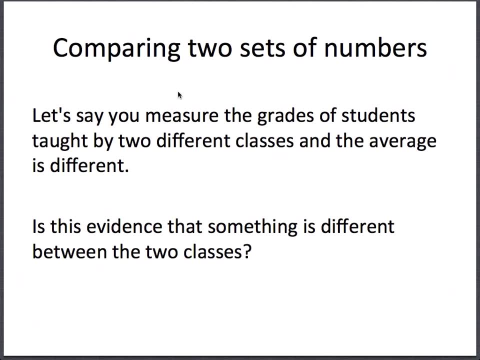 is the basic language of statistical tests, so let's talk about this. you get the class scores and you get the class sizes and you're like, wow, the average is 10% higher in classes with 10 students. so is that evidence that smaller classes give better results? well, maybe right. 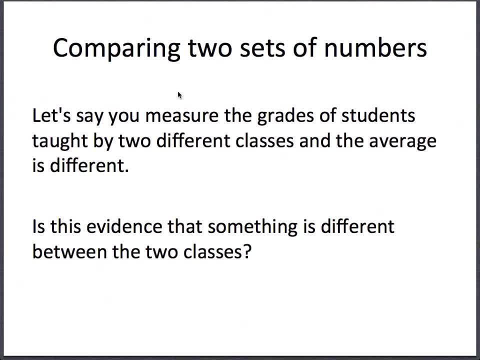 yeah, it depends. the question we have to answer is: how often am I going to see that result by chance? yeah, more years would help, although then maybe you have problem where different things are happening in different years. right you, you might not always be able to just go. 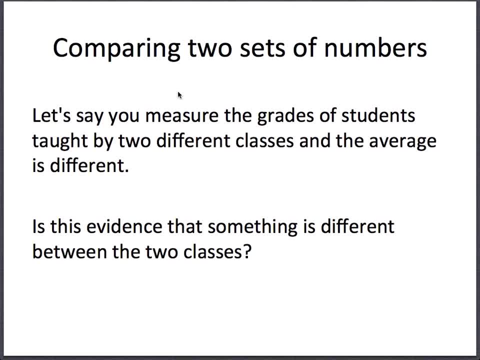 and get more data. you have the data that you have, and so the question is: what's? the answer to that question is: do you have enough to to draw a conclusion or, in the language of statistical testing, to reject the null hypothesis? has anyone heard that phrase before you're? 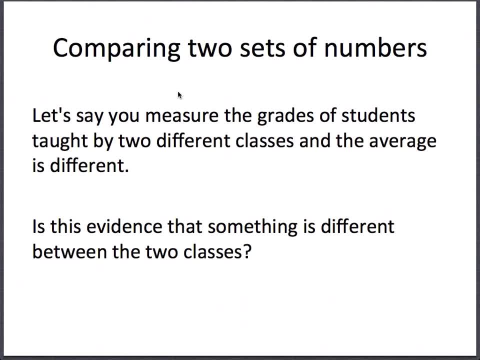 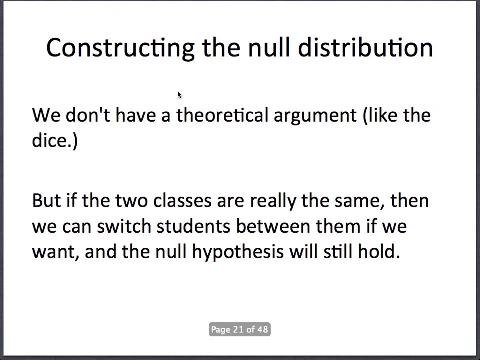 going to see that in papers a lot. that doesn't mean it's true that smaller classes get better grades. it means it's unlikely that we would see this by chance. that's what that actually means. so to do that, we have to know what this null distribution looks like. so remember. 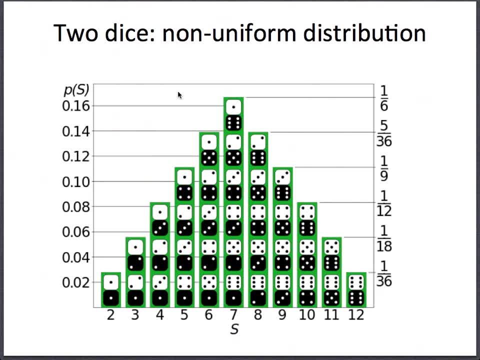 we made this little chart here, or just for rolling a die? we just expect it to be flat. what do we expect? the distribution of class sizes? so suppose there's no difference in teaching between large and small classes? are no difference in the students learning between large and small classes? what? 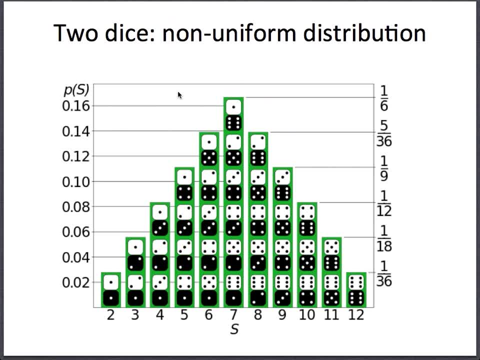 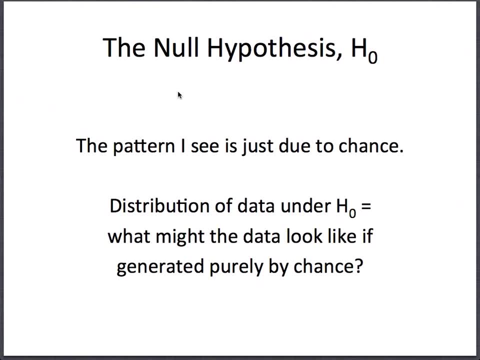 distribution do we expect for their grades? yes, then the grades would be equal regardless of class size, right, but not everybody's going to get a 78, all right. different people are going to get different grades, yeah, but we don't, so I, we don't need to have right, so you would. 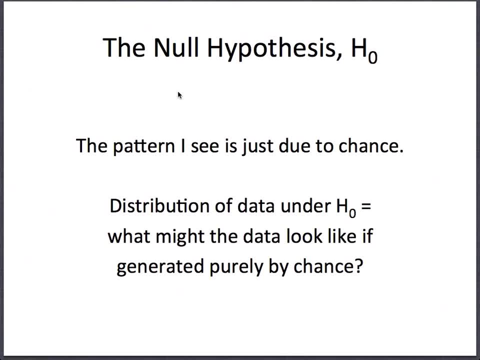 expect that the the. if you plot class size versus the grade, it would be flat. yeah, so here's where statistics textbooks normally go off into. someone set a bell curve like normal distributions and like modeling distributions. but there's actually a much simpler way and I'm going to give. 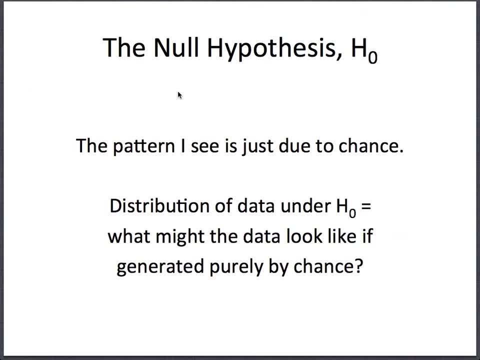 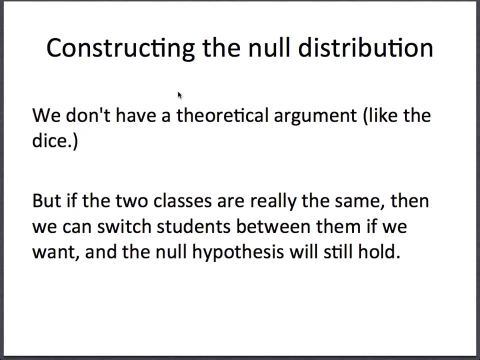 you a very simple technique to answer these types of questions, which is that let's talk about two classes for a second. if the if the students learning is really the same between the two, I can just switch them right it if all of the students are actually having the same. 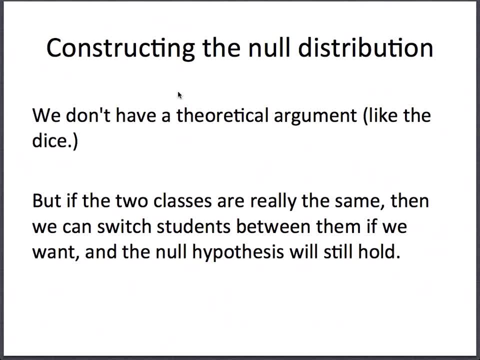 experience, then it's just chance that these students ended up in this class and these students end up in this class. so if I want to ask how often, given that I have this set of students, how often are the good half going to end up in class a, which is smaller? all I can do is: 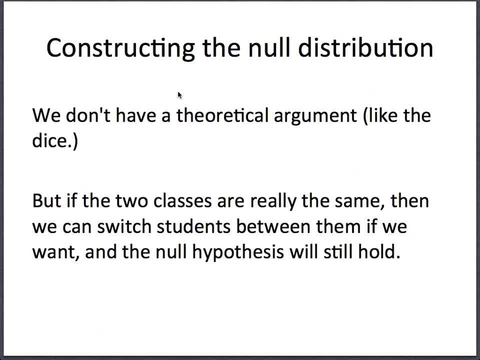 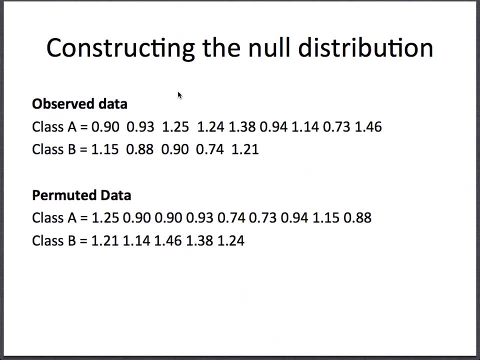 I can rearrange them in all possible ways and look at the average class score off on over all of those rearrangements. so here here's what I mean like in real practical terms. right, so say, these are scores on a standardized test. I guess I'm imagining that that you know, 1.0 is. 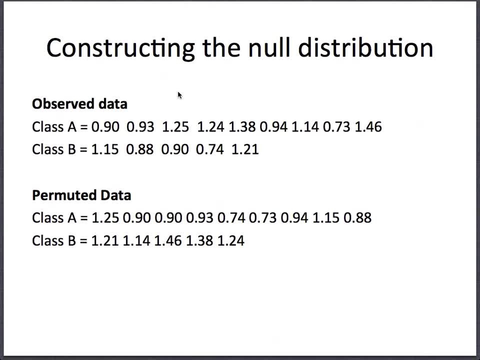 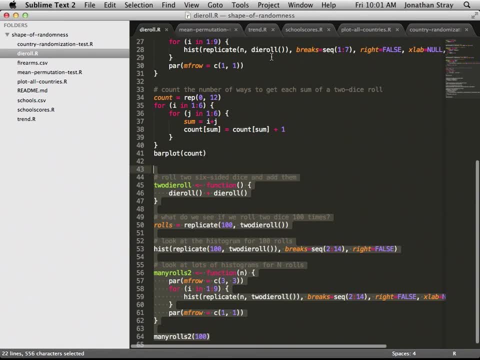 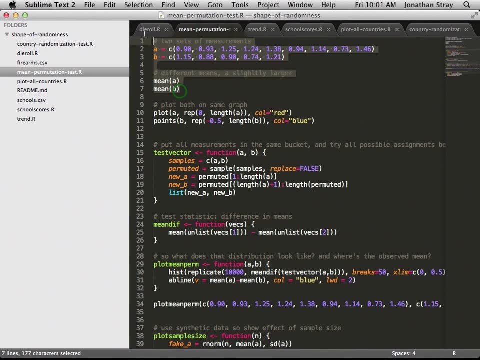 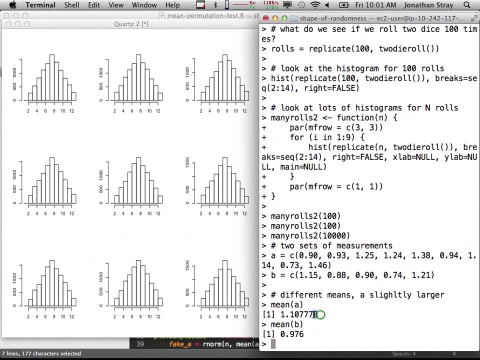 the average on your standardized test and this is what I see. I see class a has all of these numbers and I'm actually going to compute a. here we go. if I look at these two sets of numbers and I type them in and all I've done is I've asked for the average is 1.1. 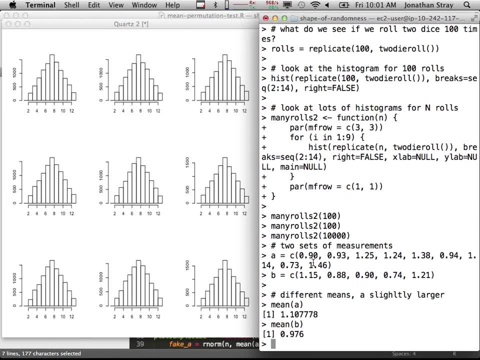 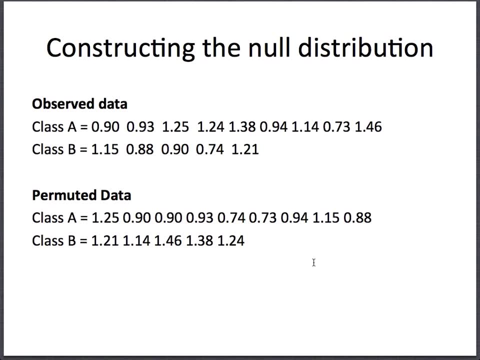 versus 0.97. so Class A has higher scores and they're not even the same size. in this case one class is smaller than the other. all I've done under permitted data is I just switch them up for the class A, And if I switch them up then they're going to have some different average and maybe 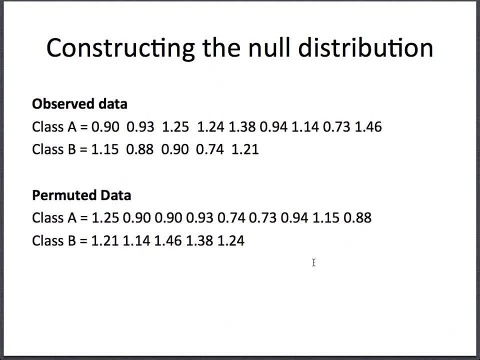 class B is going to have the higher scores. I think in this case it looks like class B has the higher scores. it's got 1.46, 1.38. And I can switch them up, all of the possible ways that they can be switched up. 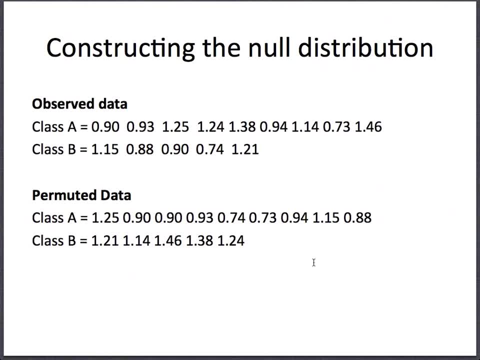 There's a few thousand different ways that this might have happened, right? So what I'm doing is I'm reconstructing chance here. I'm assuming all the students are the same and I'm asking: let's just look at all the different ways that could have happened. 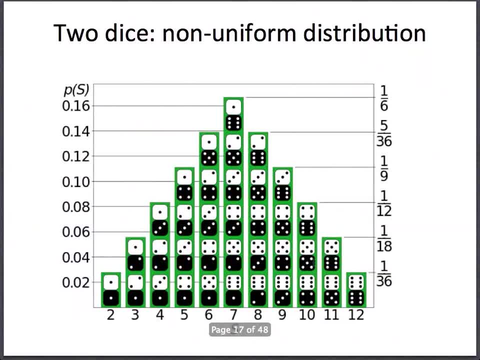 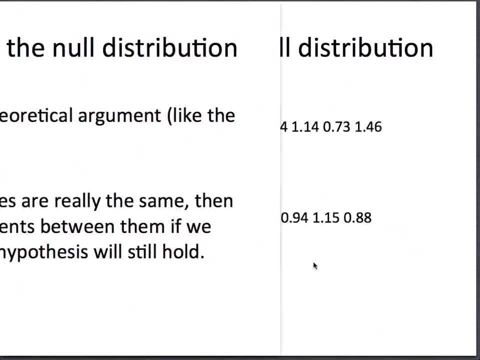 It's just like counting the die rolls here, right? So I asked here: what are all the different ways that I could have landed with two die Here I'm asking what are all the different ways I could have switched the students between the classes. 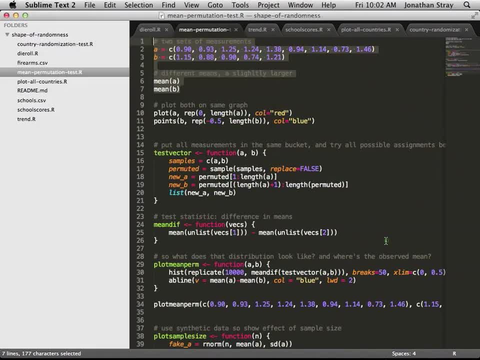 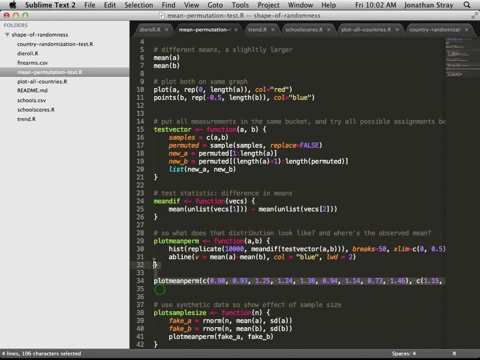 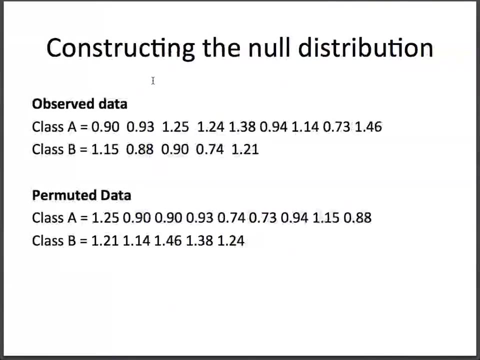 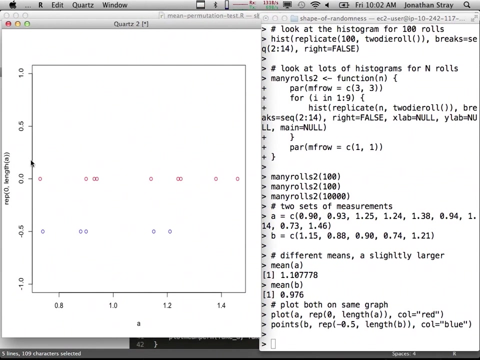 And I'm actually going to draw Okay. So here's sort of what's going on here, right? This is the scores on one class. this is the scores on the other class, And it looks like the scores in the red class are kind of higher. but what are the other? 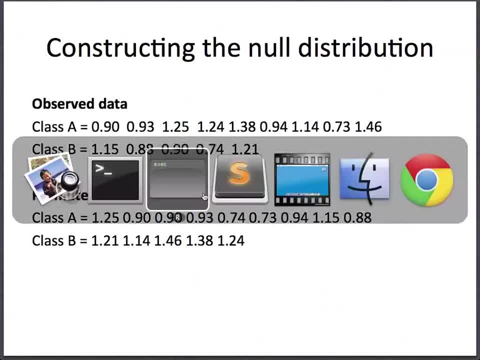 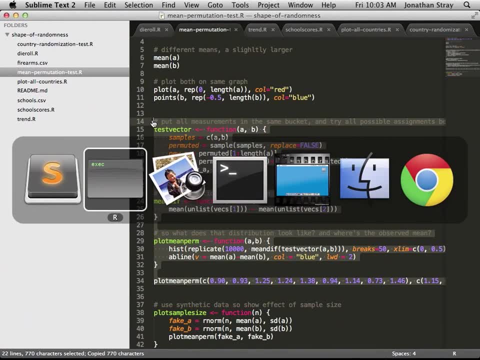 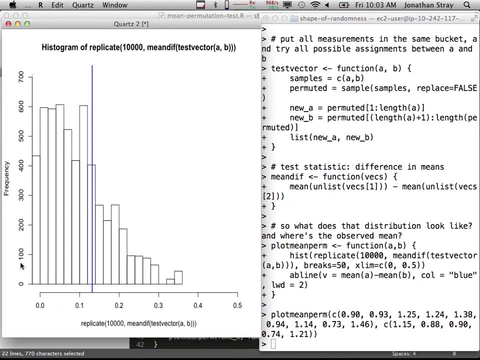 the odds that that happened by chance? And to answer that question, I'm going to scramble them, all the different ways they can be scrambled, and plot a histogram of the outcomes. So what I've plotted here is I've taken the average of one class minus the average of 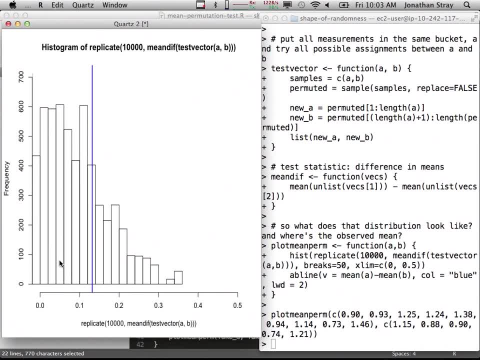 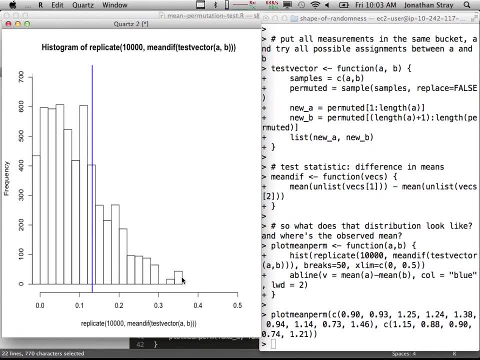 the biggest difference I can get is like if I take all of the top scores and I put them in one class and I take all of the bad scores and I put them in the other, But mostly I get a different somewhere here. this blue line, is that the difference? that? 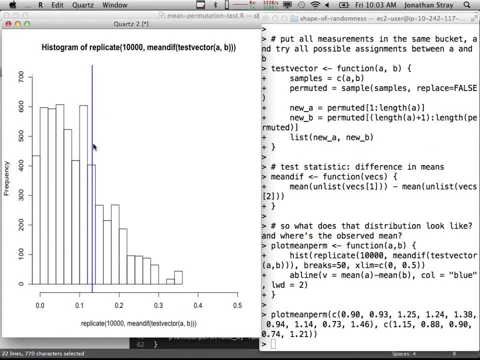 we actually saw between the two classes. Does anyone want to want to guess Like? okay, Now I've shown you this fancy plot. You know why am I plotted this this way? What does it? what does it mean to look at it this way? 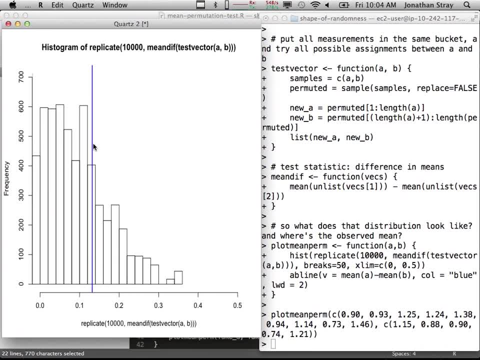 Doesn't it show that the actual result isn't the most likely thing to happen by chance, right? Yeah, it isn't the most likely, But it's not the least. I guess it's, maybe it's So the question I want to ask is: how often am I going to see a difference between the two classes that's at least as big as what I saw? 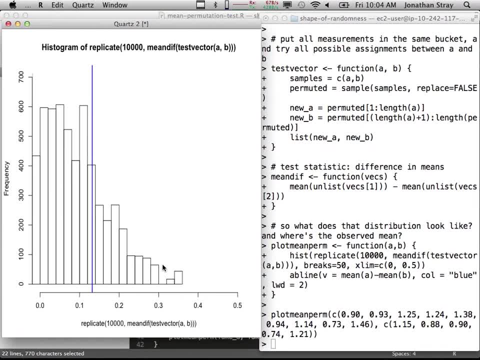 And the answer is: well, all of these cases here, everything to the right of the blue line, that tells me how often I'm going to get the scores looking much better in one class than the other class, just by chance. And this is like what? a third of all of the cases here. 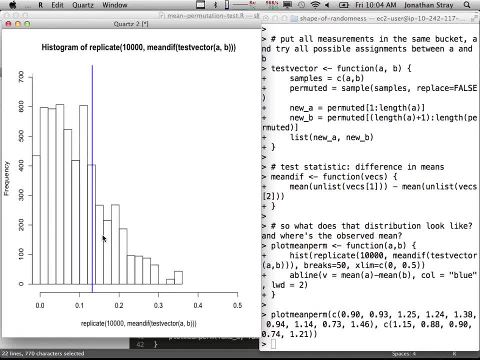 So you're looking at the area right, because each of these counts one possible outcome. So you're thinking of the area under these bars versus the area of these bars. So Does this mean that if you mix the kids, so you've got the kid, the teacher, the class with the ten kids? 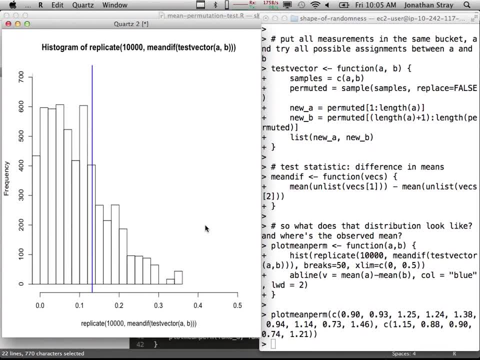 and then you've got a class, a bigger class with more kids, and the kids with the bigger class got the lower scores. and if you mix them up, what it looks like is that if you were a kid who was in class B and you were all of a sudden in class A in the smaller class, statistically I could be totally wrong. 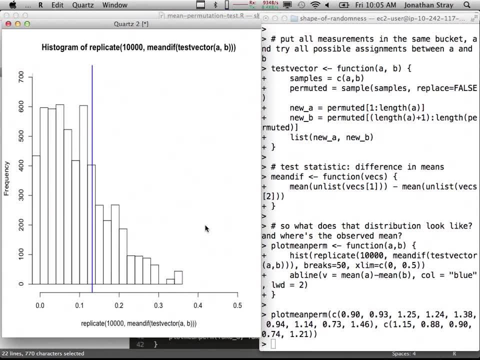 It looks to be like the kids in class B are smaller Right, And they're still not performing at the same level as those in class A, Despite the fact that they didn't switch. but I could be, So we're doing a sort of thought experiment here. 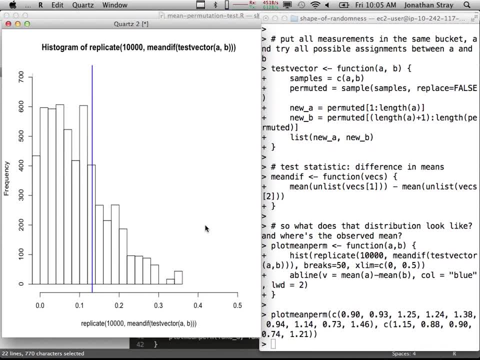 We're saying how often if the students, if all of the students, actually have the same experience and it doesn't matter what class they're in, how often if I take a set of students, these grades, how often am I going to see that the smaller class has better grades, just by chance? 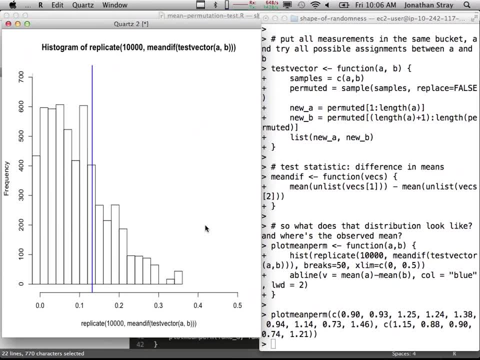 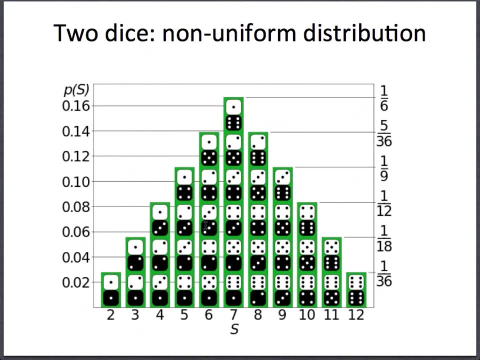 Right, And so I'm counting. it's exactly the same logic as counting the number of ways that I can roll the die. What I'm doing is I'm listing out every possible way that I can split the students between these two classes, So you know, this person could be in this class or they could be in this class. 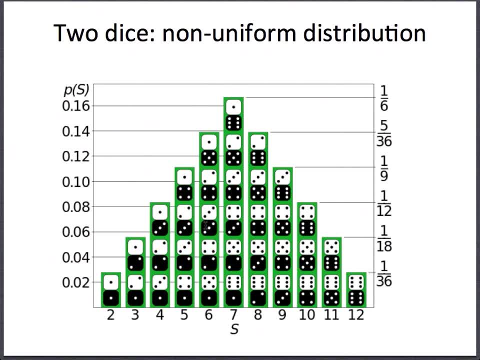 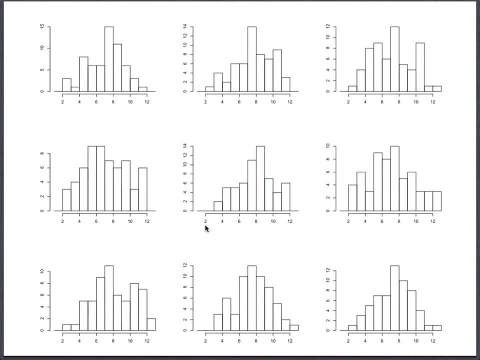 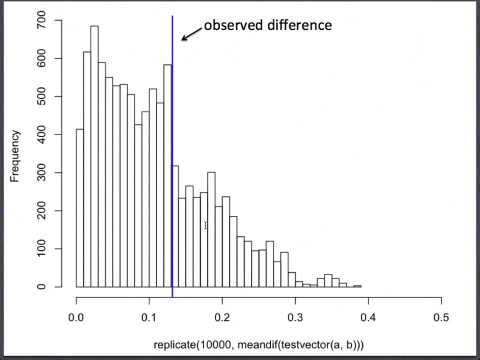 and then that person could be in this class or this class, and this person could be in this class or this class And I'm saying for each of those I'm asking what's the difference in the average grade? Exactly, yeah. 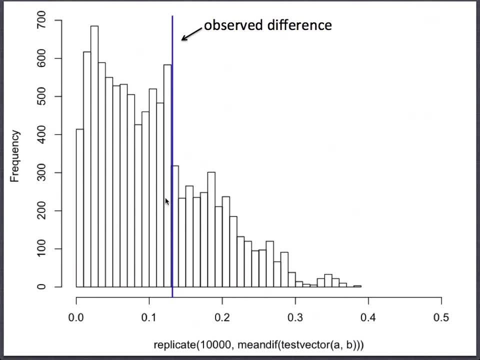 So, you know, most of the time I see a difference around .1 between these two classes. Sometimes I see a difference as big as .4.. And you know that's very unlikely right? So there's- look at this- 700 cases up here and here. 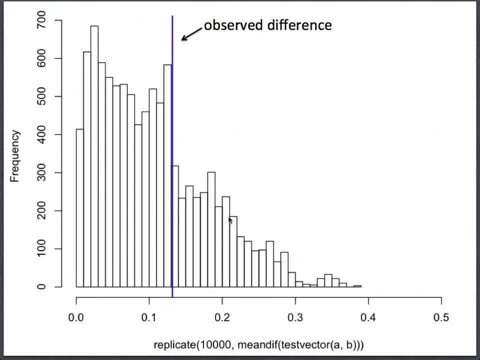 It's like 10 or something And there's thousands of cases overall, right, The total number of cases? oh, I got 10,000 different here, right? I was just thinking like if you put that blue bar and visualize like another blue bar a little to the right of .2,. 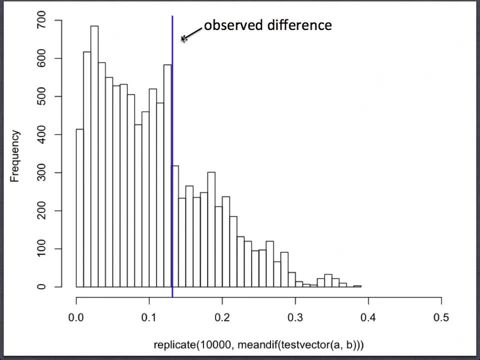 what difference is that? But this is what we actually saw. That blue bar is the scores we actually got right. So when I look at this, what it tells me is that you know half the time, a third of the time. 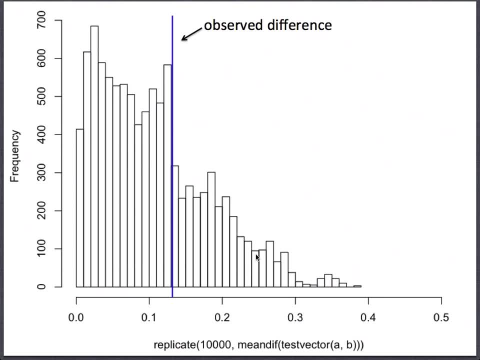 all of those cases to the right of that bar. I'm going to see, just by chance, something at least this good. So if I might have seen a difference between the two classes 30% of the time, is that evidence that smaller classes have better teaching? 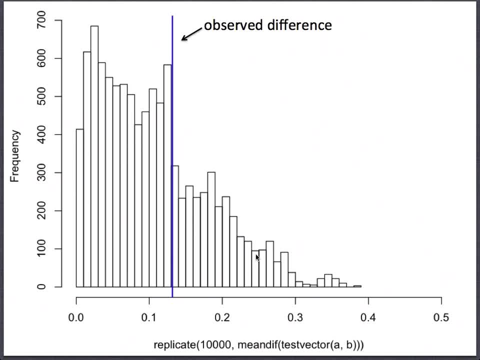 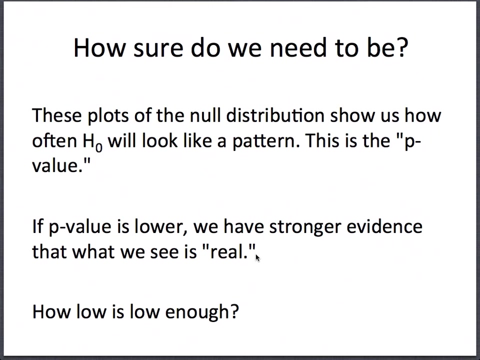 It's very weak. Yeah, Yeah, What you're looking for. generally, let's ask: in science, what's normally the threshold for the possibility of a chance result? Does anyone know? So that leads to the question: right, How sure do we need? to be right? 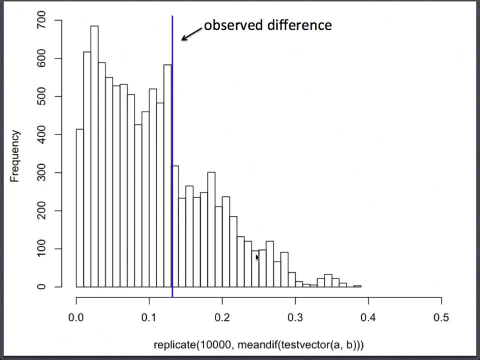 So we know that, as this bar goes to the right, there's going to be fewer, it's going to be less and less likely that what we see happened by chance, right? So like the bite of the muffin example, right, Where as the number of blueberries you got in one bite, gets bigger. 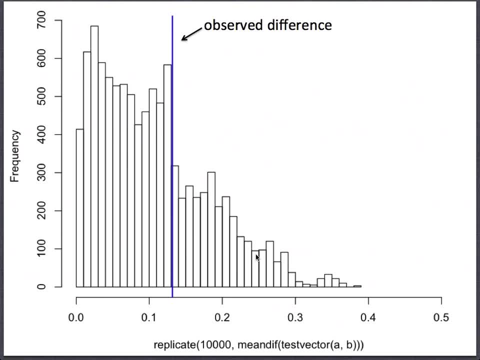 it's less and less likely that you closed your eyes and took a bite, as opposed to, like, picking the muffin with the most blueberries and taking the bite with the biggest bite right. So this is a way to calculate what are the odds. 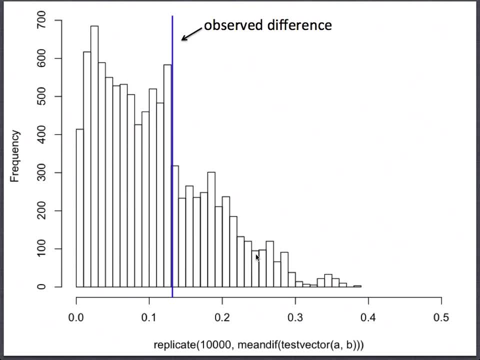 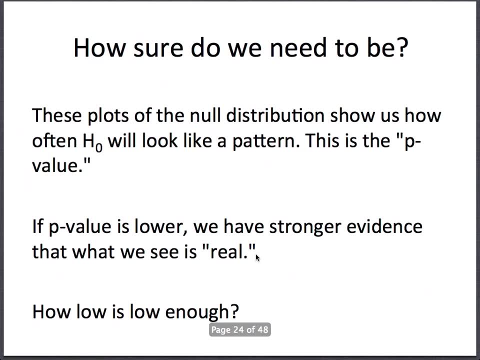 This is the fundamental question you should be asking: What are the odds? this happened by chance. How low does that number need to get? There's actually a generally accepted answer. Oh no, that's not quite where we're going. So you've seen p-values in papers in statistical testing. 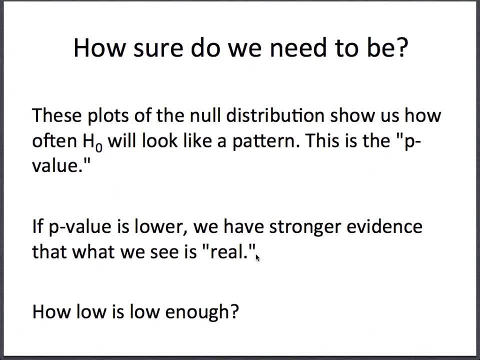 What the p-value is is the calculated probability that the result they saw happened by chance, And normally you see p smaller than 0.05, which means a 5% chance. That's generally considered publishable. It's also arbitrary. 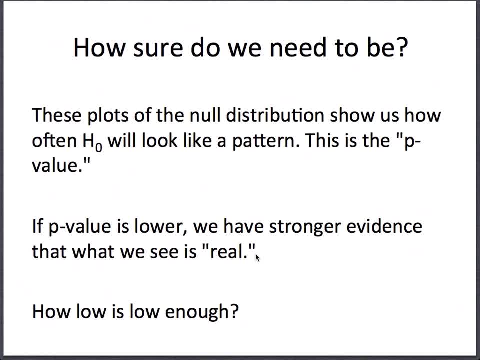 Why not? Why not 1%? Why not 10%? You sort of had to pick a standard. What's that? What was it? 5% chance, So 0.05.. I'm sorry, I just want to. 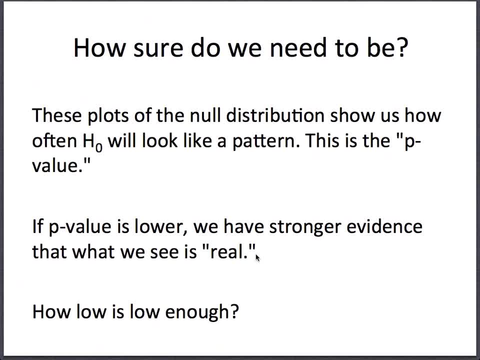 That means there's only a 5% chance. that, Exactly, Yeah, So it's 95% likely to be possible. It's 95% likely to be non-chance. OK, Right, And you still may be misunderstanding something. 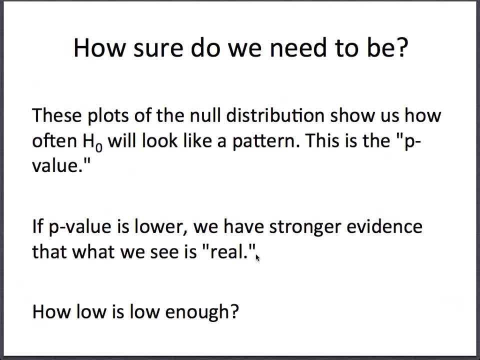 Yeah, But the first thing you want to rule out is chance Right Now, just like our loaded die example, if we have a lot of data, we can detect very small loadings on the die. So there's two different concepts here. 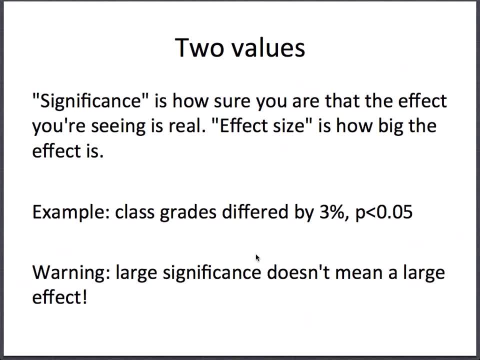 This p-value thing, this how, what's the likelihood it happened by chance. that's called significance, And so you're going to see things in science papers: significant to p smaller than 0.05.. What does significant to p smaller than 0.05 mean? 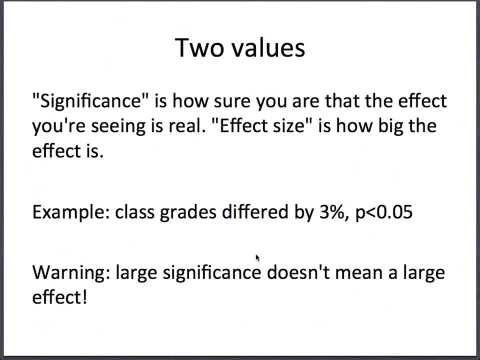 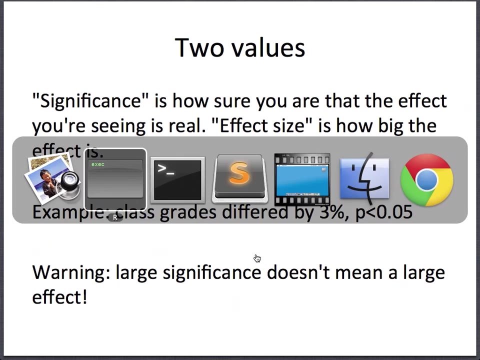 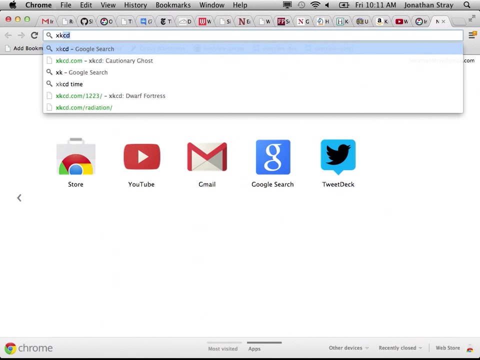 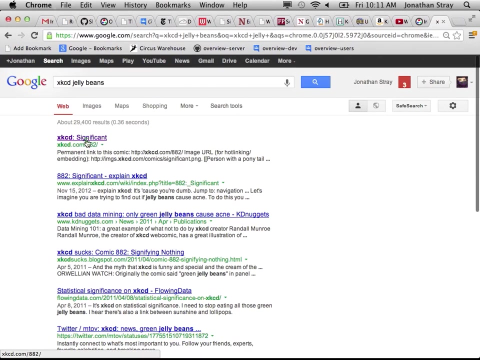 Does anyone want to translate that in English? It means 5% chance that it happened randomly, Right? So 5% chance that What you're seeing is just luck. I'm going to go to my favorite teaching tool, XKCD, which is a geeky web comic. 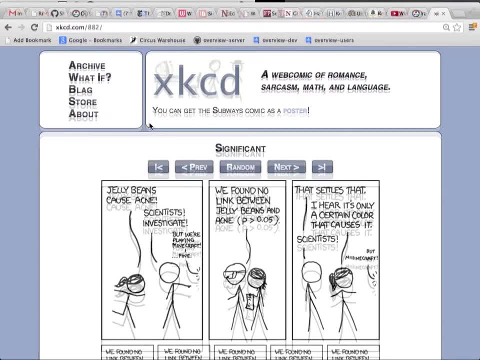 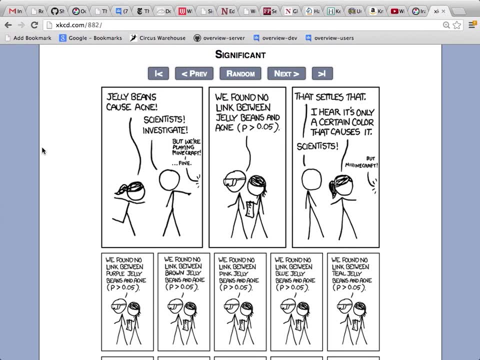 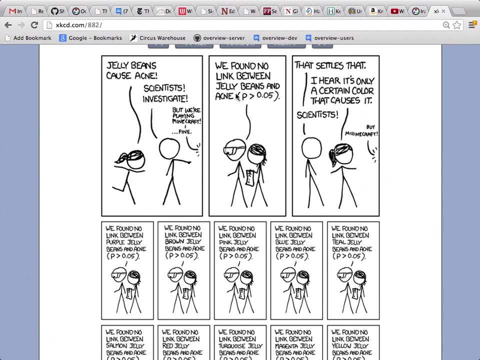 They have a beautiful example of this. OK, So two scientists trying to figure out: do jelly beans cause acne? No, We found no link between jelly beans and acne. p that should actually be smaller than 0.05.. Right, 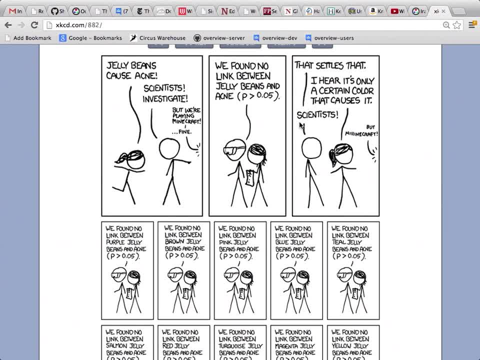 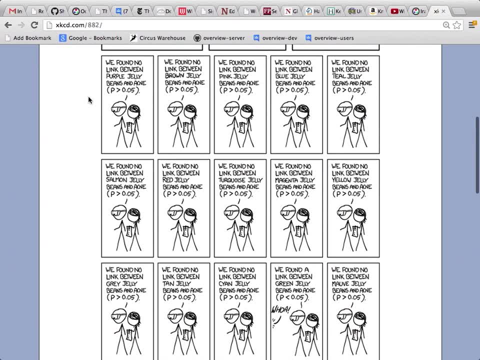 So they did the experiment. The answer is no. But then somebody says: oh, but it's a particular color that causes acne. And so they test all the colors: Purple jelly beans- No. Brown jelly beans, No Red jelly beans. 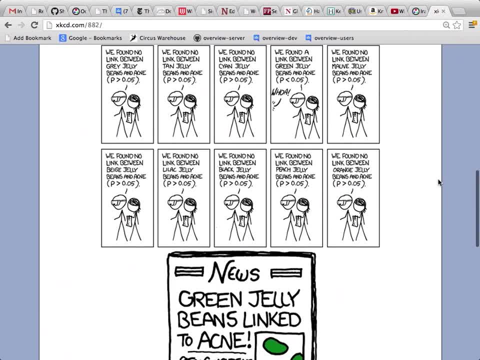 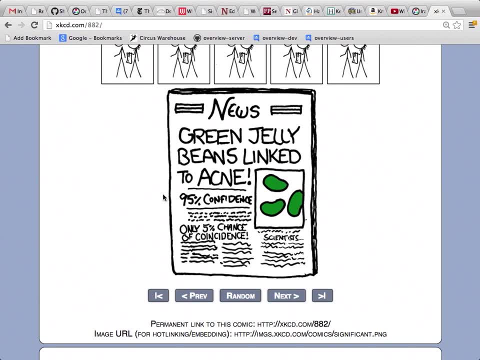 No, But then they try it. If you count, there's 20 of these Green jelly beans. 95% confidence, Only 5% chance of coincidence. That's what it means. So if all of the p-value calculations that you see in science are working correctly, 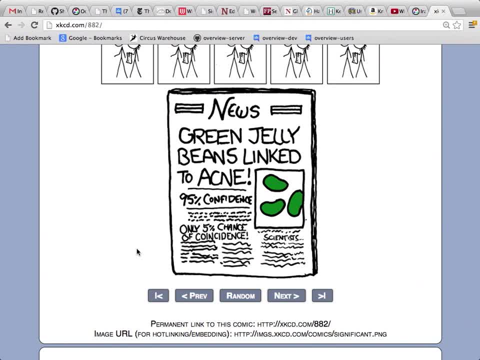 one out of 20 scientific results should be wrong. Is that a high or a low number? I don't know Right. Should we say that only something with 1% chance of being wrong is publishable? Well then, we'd get a lot less science done. We'd throw away a lot of things that are true that we just don't have enough data to prove. In fact, we suspect that it's greater than 5% of results that are wrong. There's a bunch of work looking at replicating studies and various statistical properties. 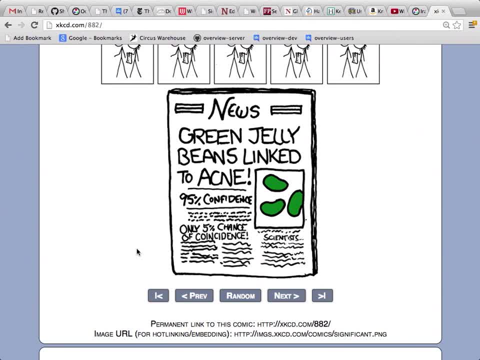 We actually think it's a lot higher than 5%, But nominally, what the discipline has been aiming for with these types of statistical tests is a 5% chance of error, And so that's why we're all asking these questions Now. but there's two numbers here, right? 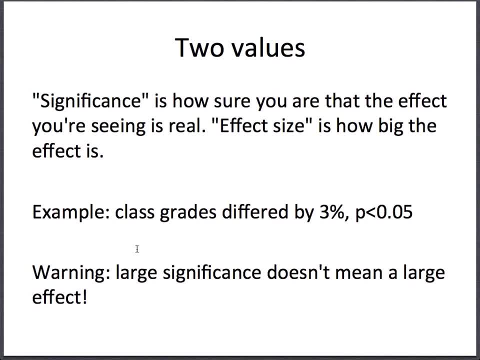 One is significance. There's this other number, which is effect size, And so you're going to see something like this: Class grades differed by 3% p smaller than 0.05.. This tells you what the likelihood that it's just random is. 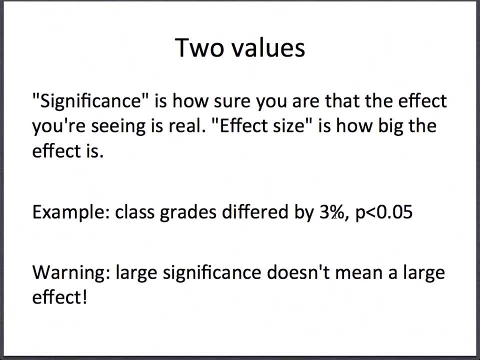 That tells you how big the difference is. They're different numbers, right. You can have a very large effect And And A small significance, right? So we see a huge difference, but we think it's quite likely it's due to chance. 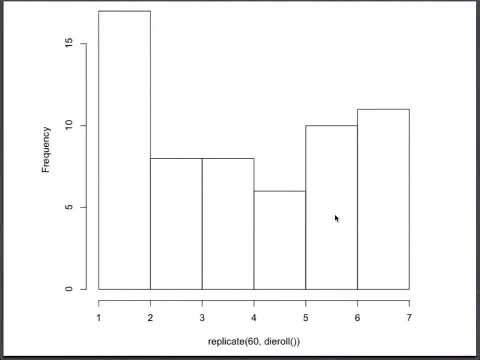 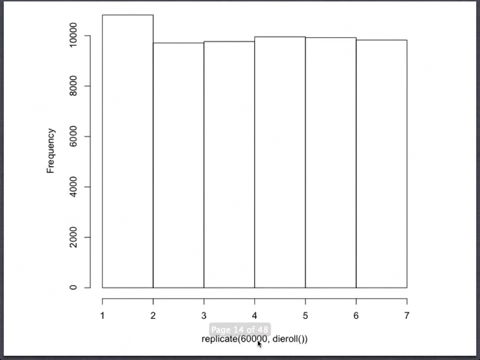 So that was what we saw with this loaded die right: Big effect, small significance, because, well, we know from our tests that you're going to see this about 10% of the time, Or you can have a tiny difference, but be really sure, which is what we saw here. 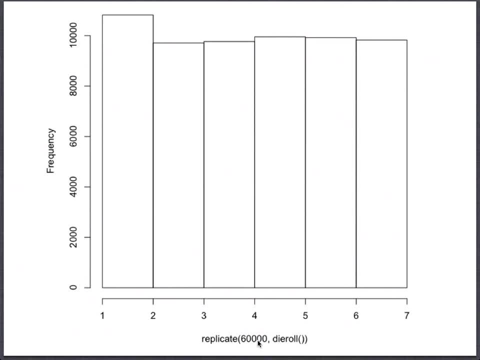 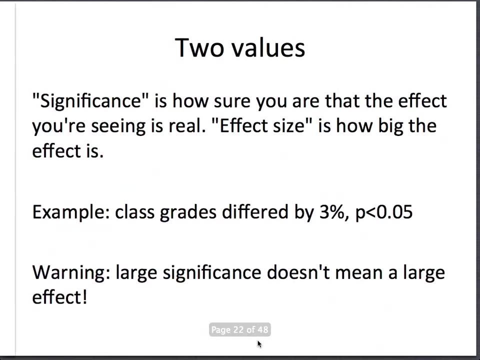 So whenever you're doing Yeah, Okay, Yeah, we're going to have to cut a few things, So whenever you're doing statistical testing, you end up with two numbers And what you really want for your story is a big difference in high significance. 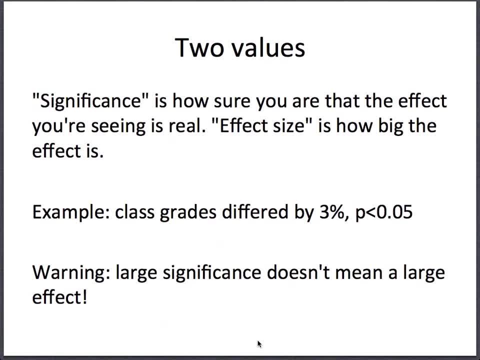 So, first of all, something with really low significance, right? So if there's a 30% or 40% chance that this is just random, can you use it? No, you can't use it. If there's only a 1% chance that this is random, you can use it. 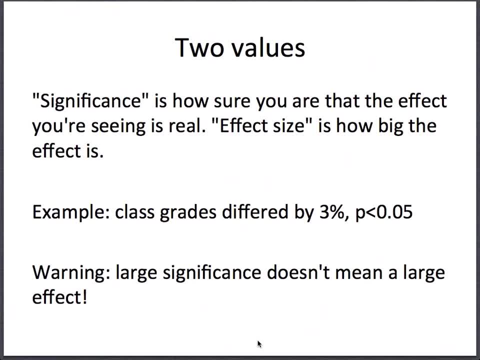 But maybe it's a difference it doesn't care about, right? Maybe we know that eating broccoli reduces cancer rates, but it reduces the risk by, you know, 5% over everyone else, And we're sure Because we have lots of data. 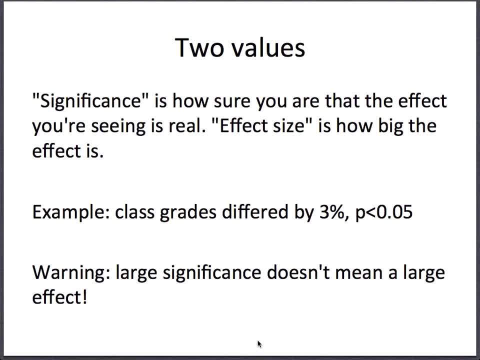 But we also don't care, because it's just not a very big change. So what you're looking for is big effect, size, high significance, Make sense. Don't confuse the two, right. So just because we're really sure, doesn't mean it's important. 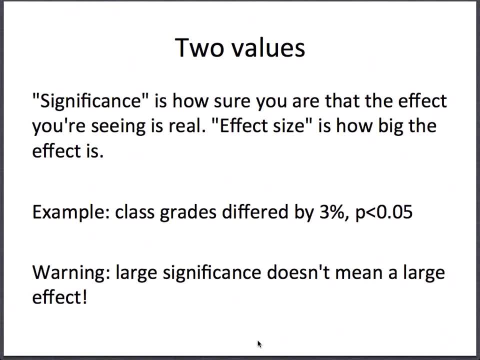 It just means we're sure, But we might be really sure that it's a very small difference, Which is good science, but not necessarily interesting, Right? So you've all heard about negative results in science, right? Negative results are important. 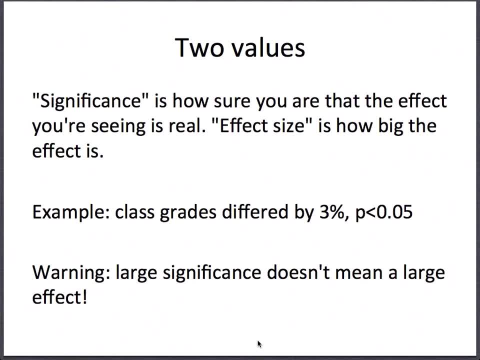 It's important to know that eating broccoli won't help your cancer risk, And you want to be sure about whether it does or not. But probably not. interesting science journalism, Unless, of course, everybody thought that it did, in which case it is. 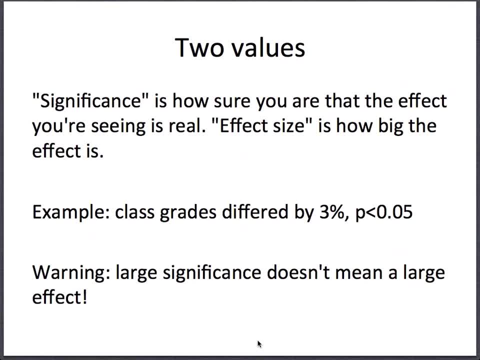 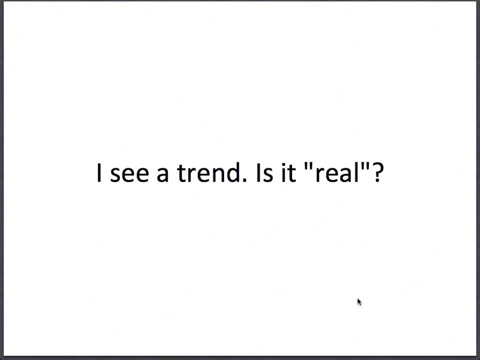 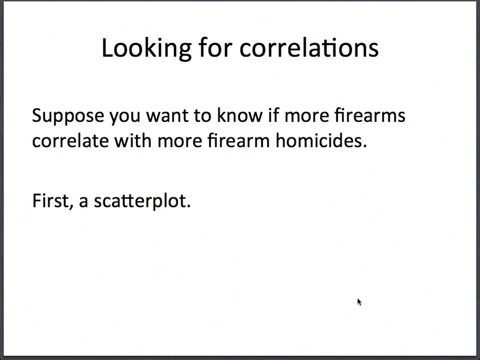 So there's two numbers. So here's a basic question. when you look at data analysis, I see a trend. Normally how you look for trends is you look at a scatter plot. So this is a story that I actually worked on because of all the gun violence stuff recently. 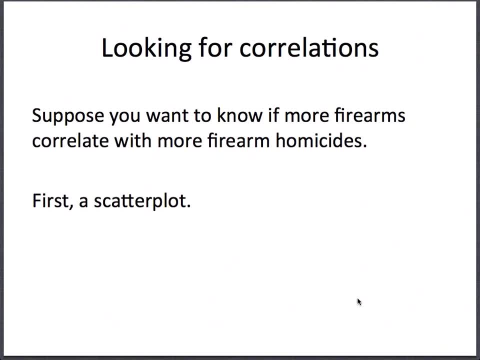 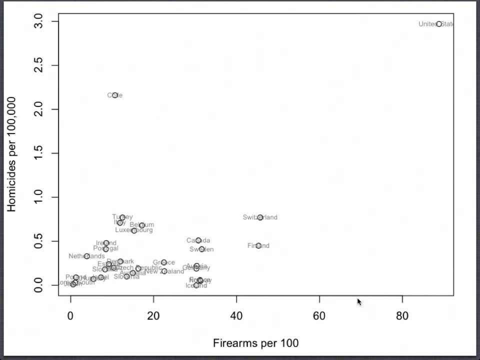 Trying to look at: do more firearms correlate with more firearm homicides? So I plotted, I took all of the data for all these different countries. This is just developed countries, Because actually developed in different parts of the world have this pattern looks different. So right away I had to make choices about what subset of the data I used. 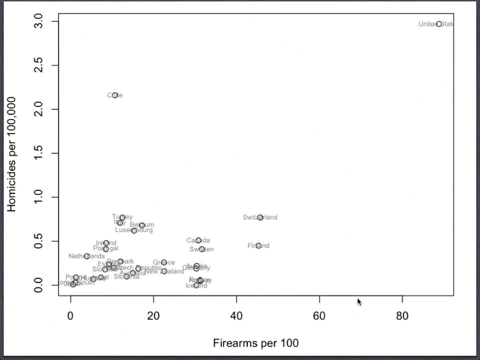 Which you should all be suspicious of. Anytime you hear somebody excluded something from analysis, you should ask why. You should ask if it would change the result. So this is this earlier step of interview, the data. But let's say for the moment that comparing just developed countries, 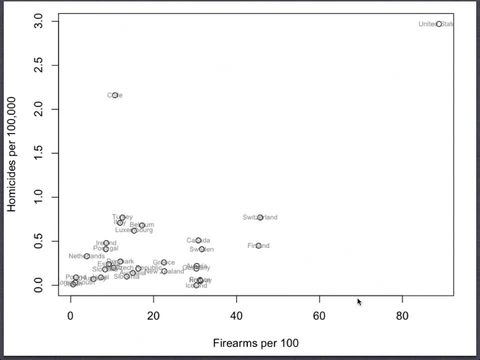 Developed countries to developed countries is justified, All right. So firearms per 100 people, Homicides per 10,000.. What do you see? Tell me what, just in words. What do you? what do you see when you look at this graph? 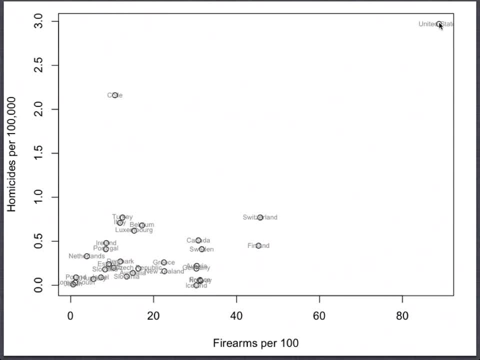 So here's the US. Well, for one country, you see this one country, which is the US, Which is a huge number of firearms and a huge number of firearm homicides. Okay, So where here? That's Chile, That's Switzerland. 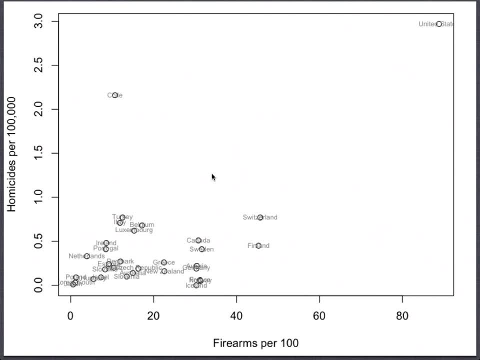 That's Finland. Switzerland has a lot, of, a lot of guns because they have a militia. They don't have an army. But You know they have half the number of guns but only a quarter of the number of homicides. So do you think there's a pattern here? 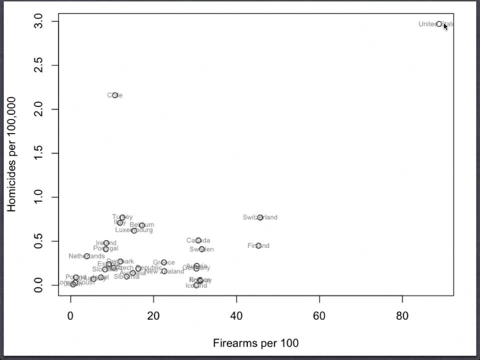 What about the rest of the world? Right, The US is here, but maybe it's weird in some way If I, if I take the US out, is there still a pattern? Not really, Yeah, So let's. 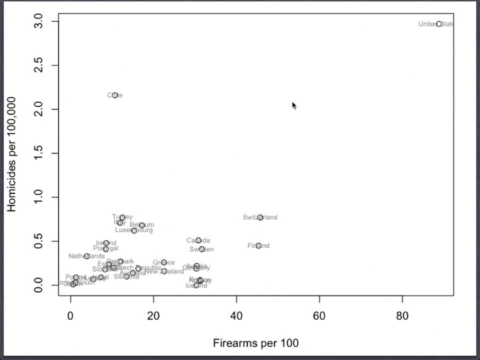 How would I, how would I do a statistical test? How would I get an idea of whether this relationship is random or not? Anyone got a? got an idea? Isn't the idea that, for a given number of firearms, how likely are you to see X homicides? 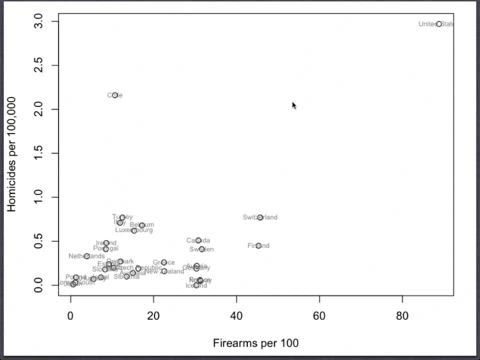 And how likely is it to the chance that you would get a lot of homicides with a certain number of firearms? Well, what I'm looking for is: I want the chance that if there's no relationship at all, if I'm just, if the number of homicides is just a roll of a die, what's the chance that I'm? 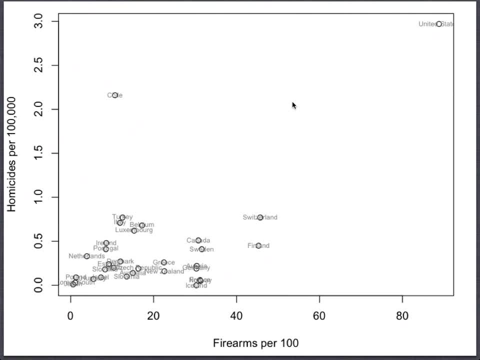 going to see this pattern by chance? Yes, Sorry, you had a question. I was wondering if. Does this include? I mean, does this include the? Does this include the death by firearms illegally acquired? Is that, Yeah, All cases. 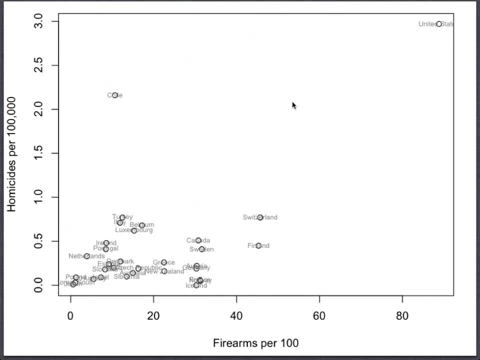 Do you make the difference in this, This data? No, it's, it's just death by firearms Full stop. It's it's annual, It's annual rates. It's it's 2011 data, I think, And it's it's it's population, adjusted on both axes. 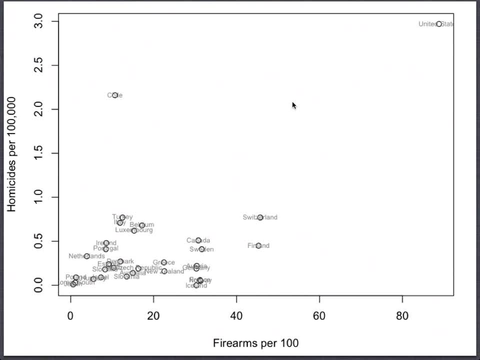 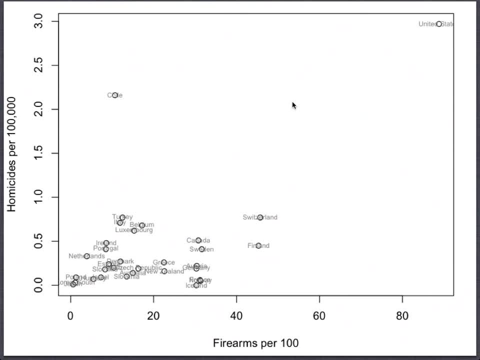 Can you make a comparison within the same country that used to have would allow civilians to have guns, and then change the law and then see in the pattern there happened there where there's Yeah, but then you have to ask the question: how, how likely am I to see that pattern by chance? 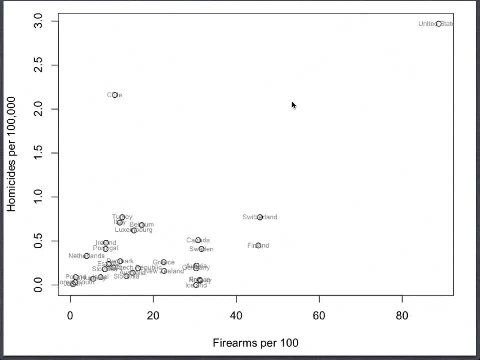 And you know if and also what other factors right. So if there's all of these other things that are going to change the level of gun homicides, how do I know that? what I'm looking at is because the regulation change and not because of? 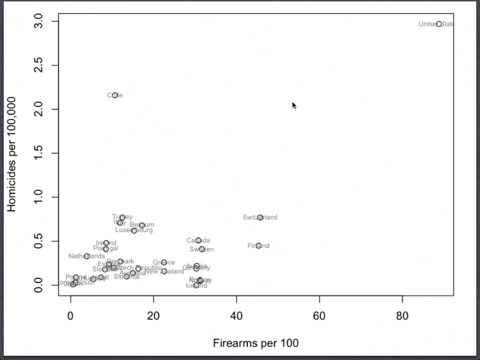 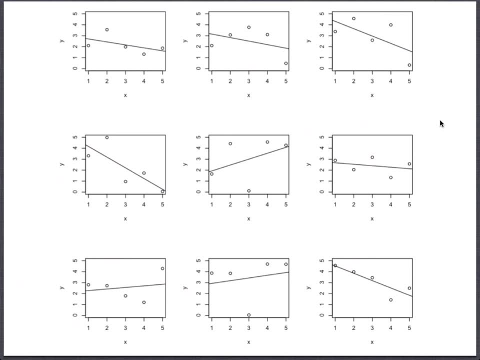 something else We're going to get into cause in a second. So here's the trend equivalent of the charts I showed you rolling the die. what I've done is I've drawn five random points And then I've drawn a line through them, right So? 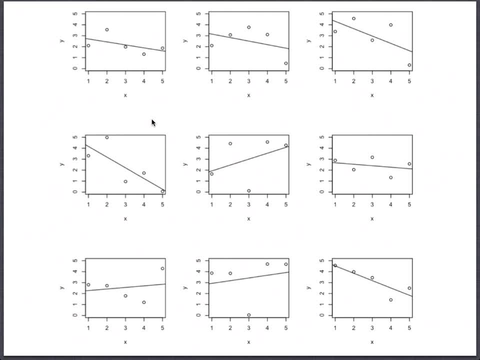 just 12345.. And then I've chosen a random value and I've drawn a line through it. How many of these charts would you say look like Like there's a solid trend? Yeah, lowest Right Looks like there's really a trend going on here. 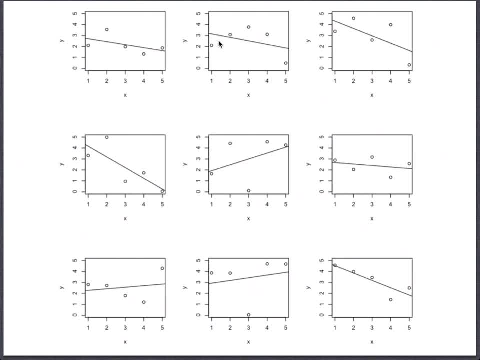 Or maybe this one right. So maybe this isn't the line, Maybe this is. imagine these are car crashes at an intersection. Oh, they went up for a while And now they're going down. The City Council has really done a great job. All right, So you really? 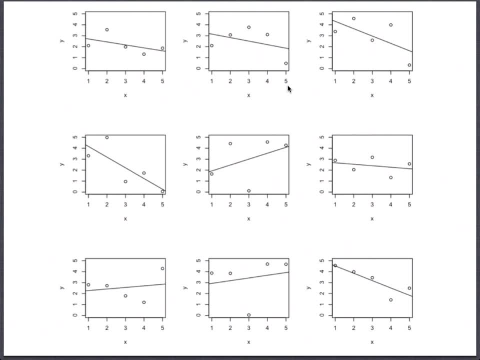 want to write that story, But what I'm trying to tell you is, if you only have five points you're going to. these are all random, Right, So so I'm gonna say about two and nine. Yeah, sure, if you have it. 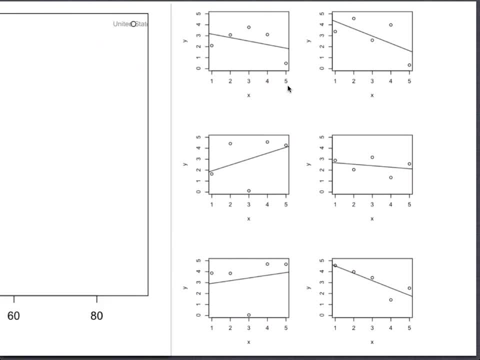 For what? Which one? This one One year, one year, one year. So can you do this for the last 10 years? Sure, although something may have changed over the 10 years. So, but I'm looking at a different variable, right, I'm imagining. 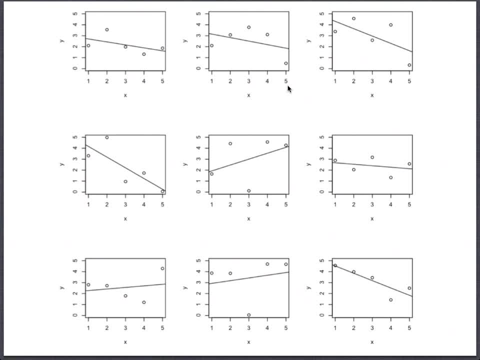 that each of these is one year now, like I'm counting number of car crashes, Okay, And so I plot them and I see that there's a steady downward trend. But what is the chance that I'm going to see a steady downward trend just by chance? Somebody actually give me a. 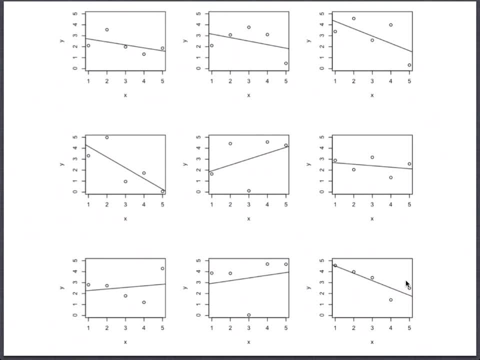 number from from this chart, you should be able to give me a ballpark number. How often am I going to see a steady up order downward trend, just randomly? if I take five numbers, Oh, like to turn on. So what is that in terms of percentage? 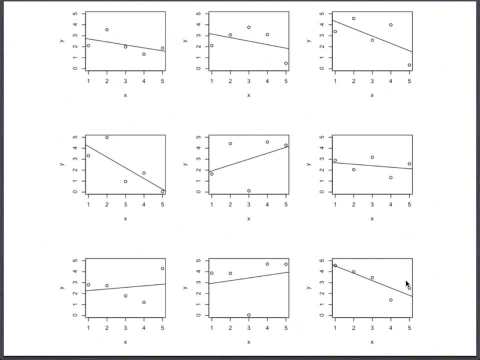 Yeah, 2320, odd right, Something over 20.. All right. So is that, if you see a trend with only five numbers, Is that statistically significant? No, no, Because this is like the p value, Exactly. So if you're going to see it look like that, one out of 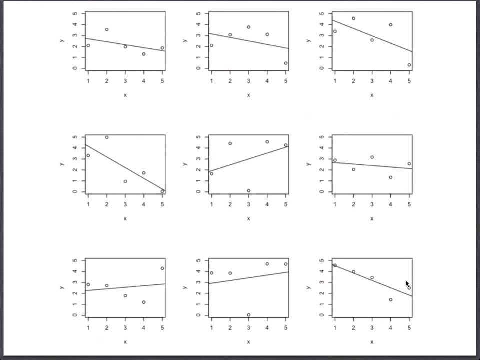 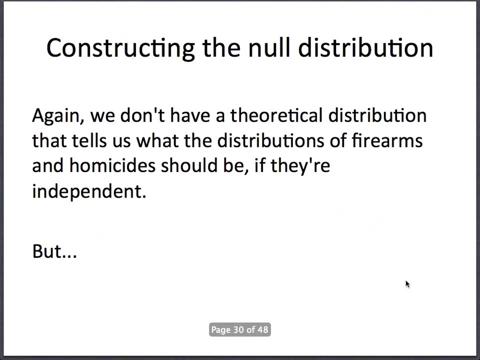 five times. it's not really a story. The p value is too high Exactly. The chance that it's going to look like that just randomly is much too high. Now for firearms. I don't know what it theoretically should look like, But 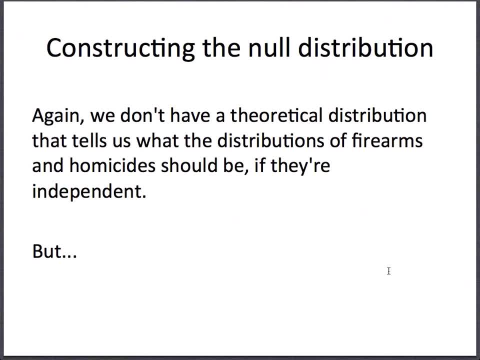 I've got this trick, which is, if there's really no relation between the number of guns and the number of murders, then if I swapped the number of murders, just switch them around between the data, right? So I take Chili's number and I read, and I: 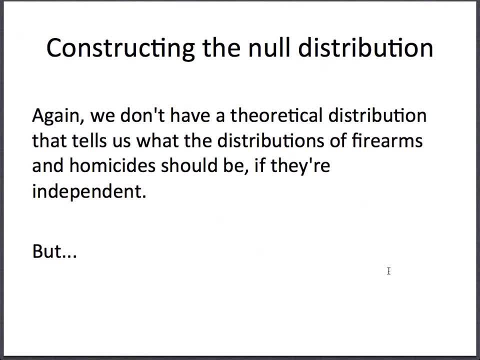 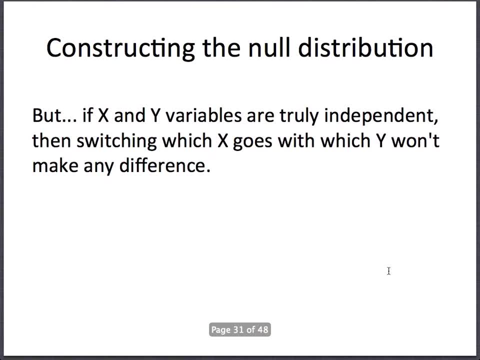 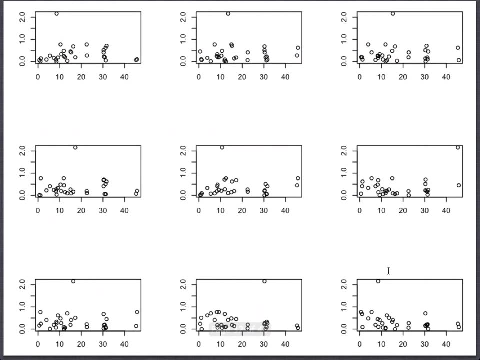 give it to Argentina, and I take Germany and I reassign it to Canada. It shouldn't make any difference. I should see the same pattern. So that's what I've done. This is the same idea, but now I've just scrambled all of all of the. 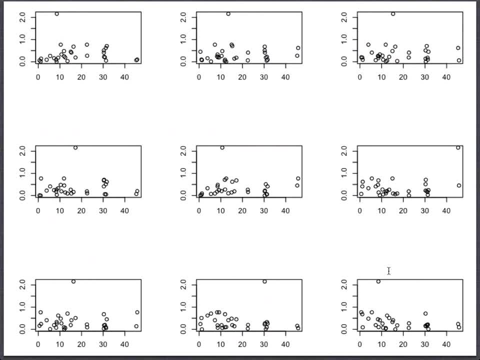 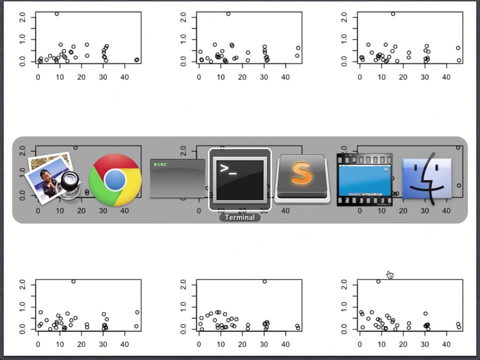 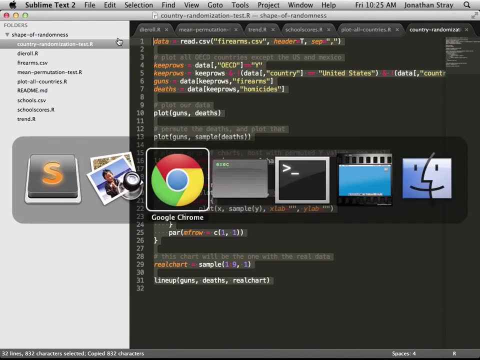 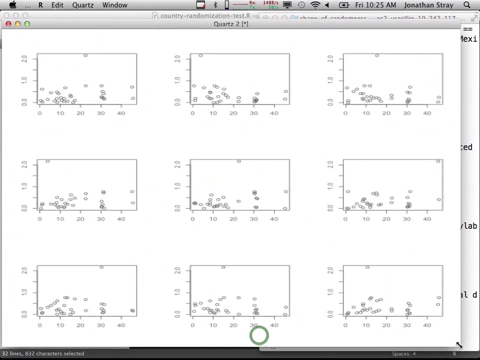 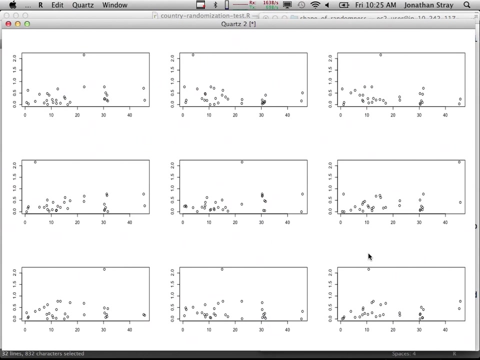 country labels. So which one of these is the real data? In fact, we can do this experiment right now, Okay. Okay, So here we go. One of these is actual data on gun deaths versus firearm ownership, And the rest I've made by scrambling the numbers right. So I've reassigned to the countries randomly Which one is real. 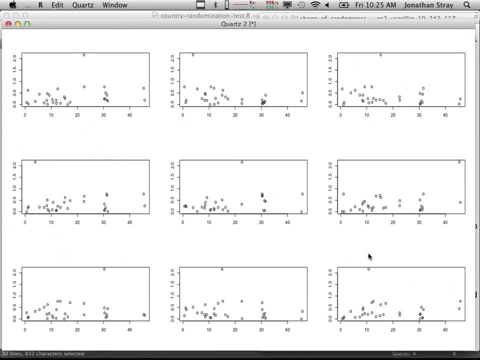 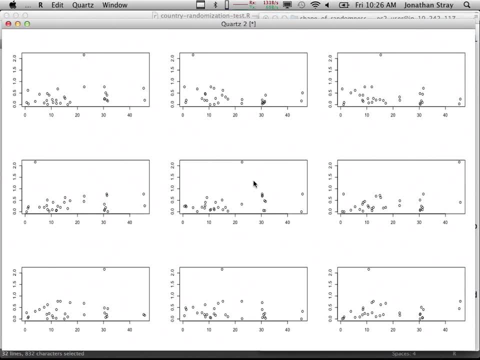 I'm a bit lost. I don't understand any of these, This way of scrambling that. Why are we going to get some tests done? you're going to get something to eat. I don't understand this SEBASTIAN DETERDING- Why we scramble it. 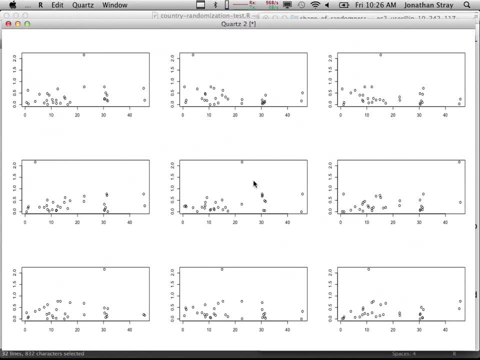 Yeah, It seems easier when it's going to the kids at the school- SEBASTIAN DETERDING-. So what we're trying to do is we're trying to say, OK, suppose there's no relationship between the number of gun deaths. 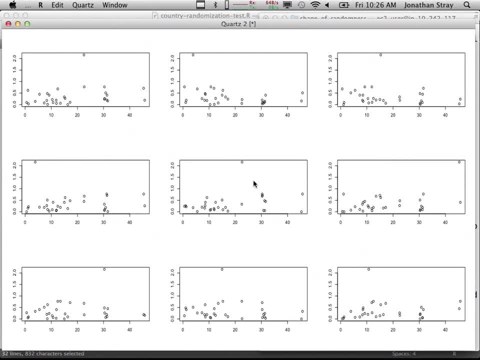 and the number of guns. Well then we should see the same pattern. The plot should look the same If we switch all of the numbers between countries. so if there's a very clear relation, like, say, there was a very clear upward trend, 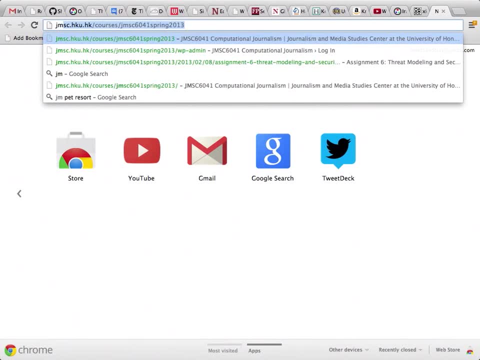 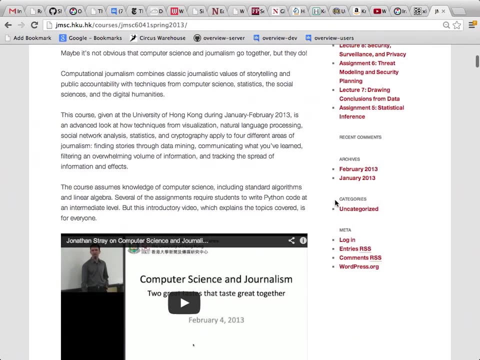 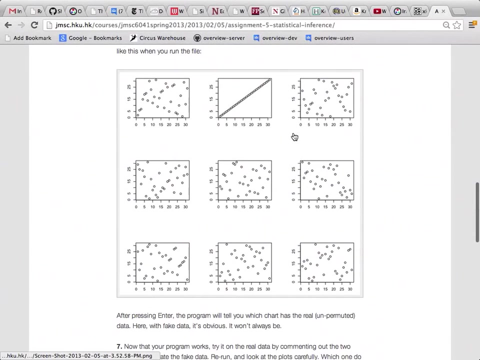 So here I've actually got a picture of this. This is a course I taught in Hong Kong. I actually gave this as an assignment, All right. So here's an example where- OK, which one is the real data and which ones are the scrambled ones. 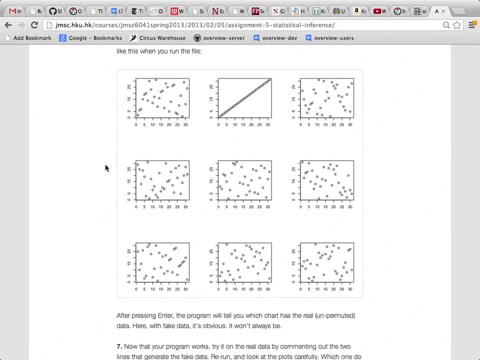 Anyone want to guess which one is the real data from that? The top center, SEBASTIAN DETERDING-. Yeah, So perfect correlation here, right? So this is a very clear pattern If I take it and I scramble which number. 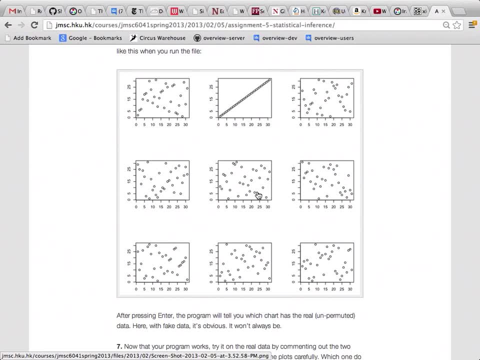 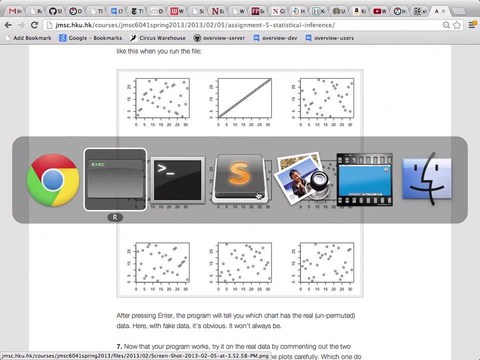 goes to which country. it's easy to tell that it's scrambled, So you never get that. You never get that straight line by chance, And so that means there's a very low probability that that straight line happened randomly, which means it's very strong evidence. 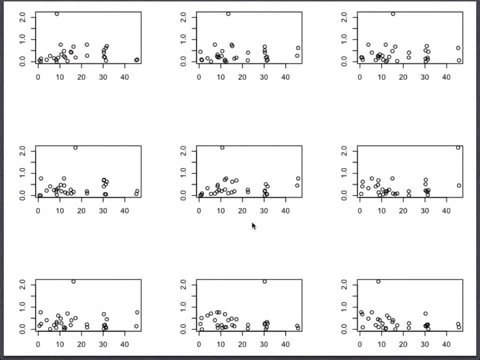 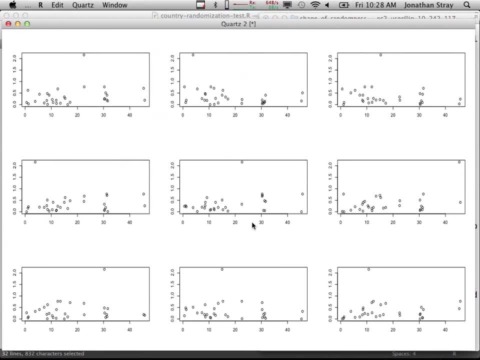 But here with the real data. one of them scrambled, Or sorry. actually, here we go. That's our experiment. One of them was scrambled. They're not that different, SEBASTIAN DETERDING- They're not that different, exactly. 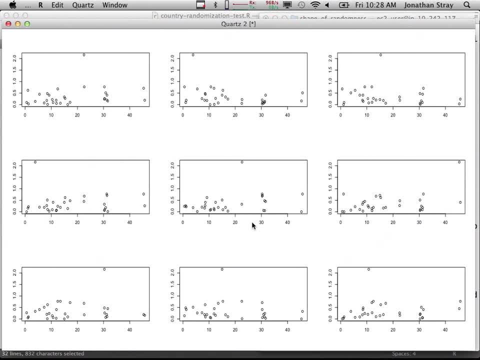 Which means that the US is still up there, regardless of who's scrambling the data- SEBASTIAN DETERDING- The US is still up there, So we can definitely say that the US is an outlier. It's different from all the other countries. 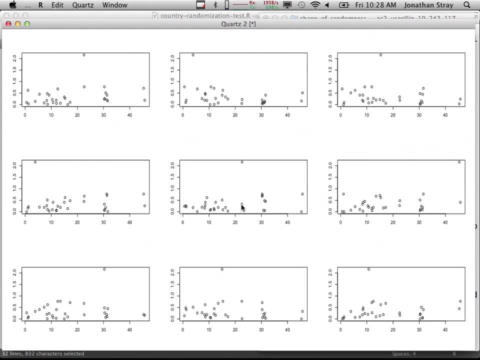 But that's different than saying there's a trend, Because all of these look the same. if you can't even tell the real data from the randomly scrambled data, that's very strong evidence that there's no trend, Because the real data that you looked at 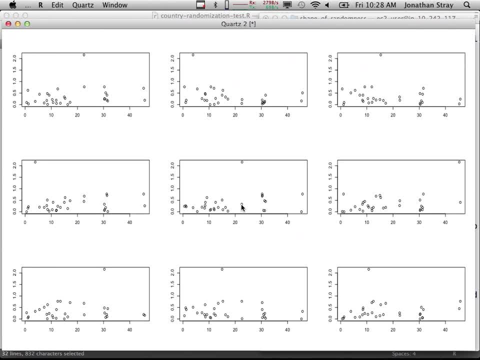 the real data. SEBASTIAN DETERDING- Yeah, It's likely that. I mean it looks so similar to the data that was just produced randomly. SEBASTIAN DETERDING- Mm-hmm, Yeah. 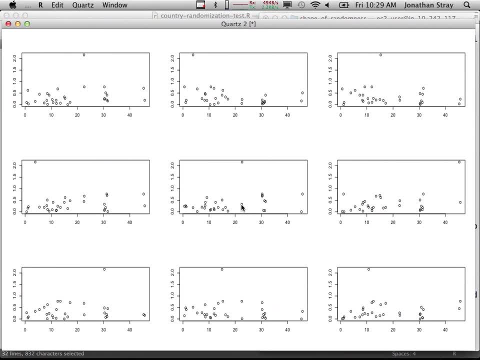 Yeah, SEBASTIAN DETERDING- Exactly. So you can just show that there's a good connection between these five sources. SEBASTIAN DETERDING- Exactly. SEBASTIAN DETERDING- Exactly. 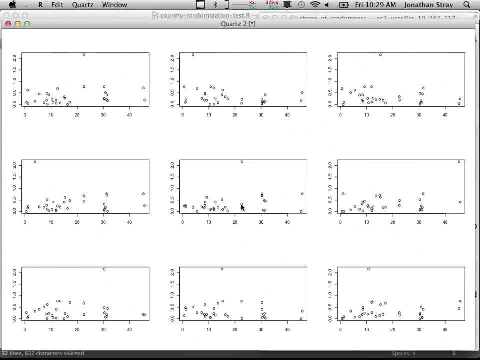 At least in this data, Or that. there's some other thing that goes into this. Then there's some other variable, SEBASTIAN DETERDING- Well, there's many variables. Yeah right, Exactly So, just with these two variables. 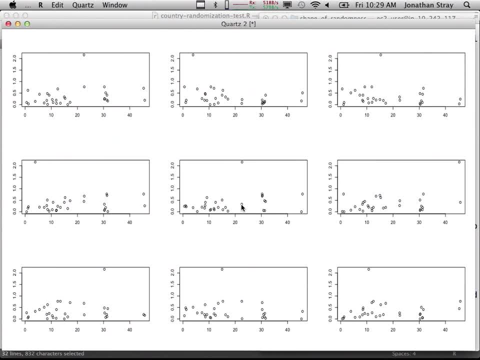 SEBASTIAN DETERDING- But these two variables, aren't it Right, right? SEBASTIAN DETERDING- Yeah, Right, But in homicide, there's many, many variables, right? It cannot be only whether you have a gun in your hand. 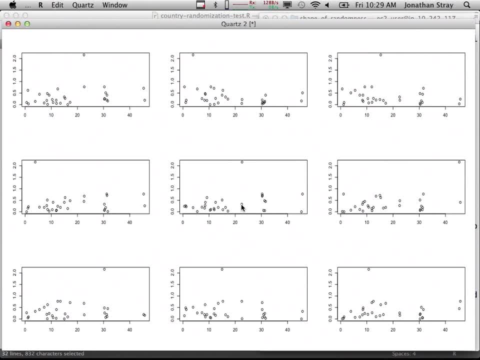 or not, or in your drawer or not. SEBASTIAN DETERDING- Right, I mean it's linked to a lot of many, many variables. But even in and therefore, because countries are very different- variables it's. 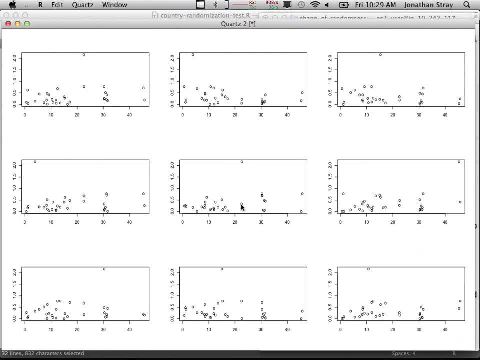 really difficult to get a plan, and a plan that's impossible to get, a plan, But isn't valuable the fact that there is, So it may be. so here's the story you can write. The US has both way more guns and way more gun violence. 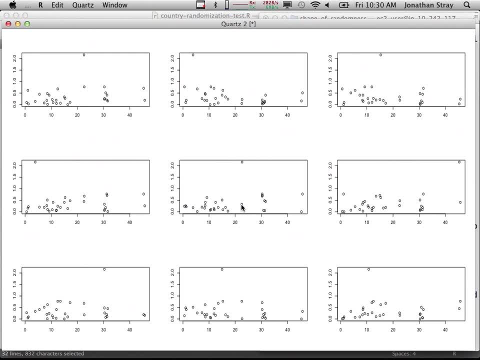 than any other country, But there's no evidence that a larger number of guns is the cause of more violence internationally. It might be the cause in the US. It's not a cause, It's internationally, because there's no pattern right. 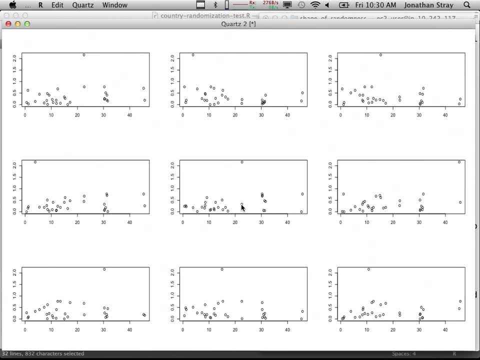 It's not a pattern, It's an outlier. Does that make sense? So you have to be very careful to avoid misleading your readers. You can say the US has the highest number of guns and the highest rate of gun violence, but that's not a trend. 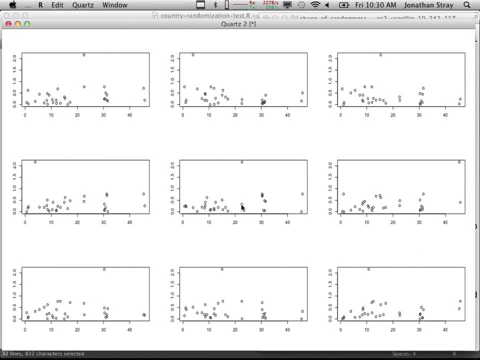 It's one point, SEBASTIAN DETERDING- Well, because you don't kill a person just because you have a gun. So obviously there is something else in play. But doesn't this? but given the huge difference, doesn't this? 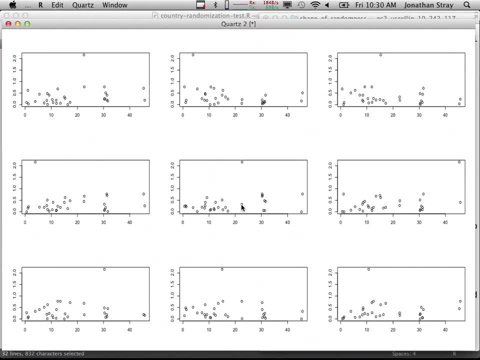 SEBASTIAN DETERDING- Mm-hmm. SEBASTIAN DETERDING- Mm-hmm. Doesn't that show that if you have a higher number of guns, do we have a higher number of homicides? 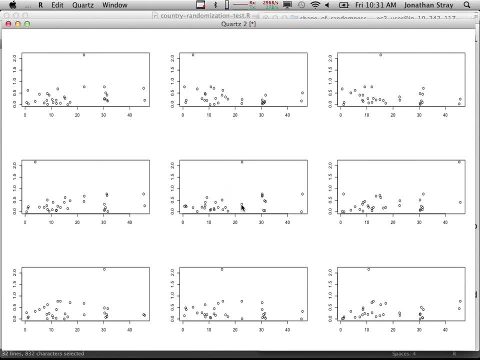 SEBASTIAN DETERDING- No, Absolutely not, Because we can't tell the real data from the fake data. So you're saying: But there is one thing that doesn't change, even when you change the data, which is the fact that everybody else is sort of this big distance. 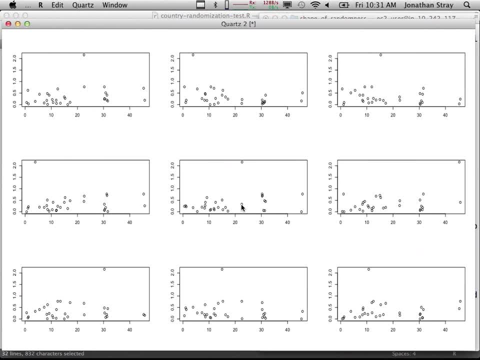 I mean SEBASTIAN DETERDING-, But the US is only one point though, So there's not a trend technically, SEBASTIAN DETERDING- Yeah, And furthermore you don't even know cause, right? 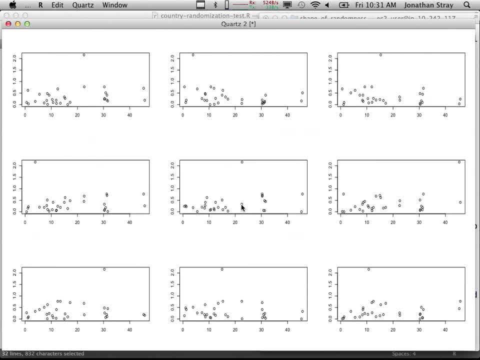 Maybe people buy more guns because they're living in a dangerous place, right? So we have two problems: We have to show that the pattern is not due to chance, which is everything we've done so far- And we have to show that causality. 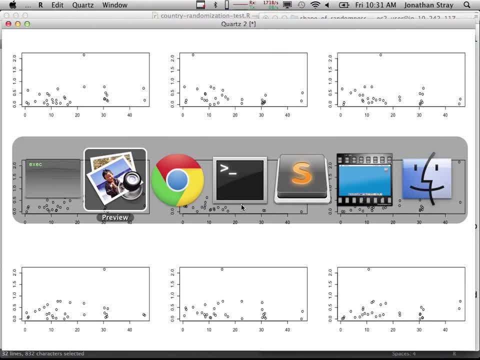 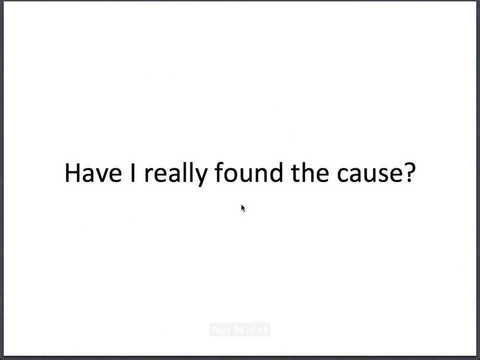 runs the way we think it does, And I'm actually going to jump ahead to talk about causality, because we're almost out of time. We're going to skip all of that. Have I really found the cause? So far, we've talked about correlations. 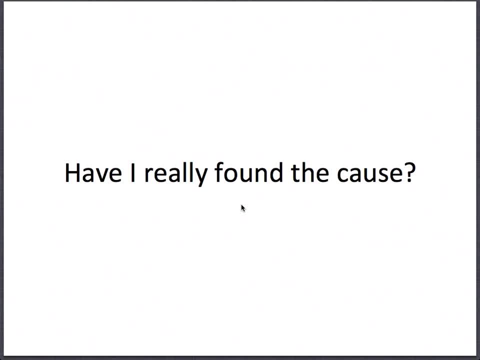 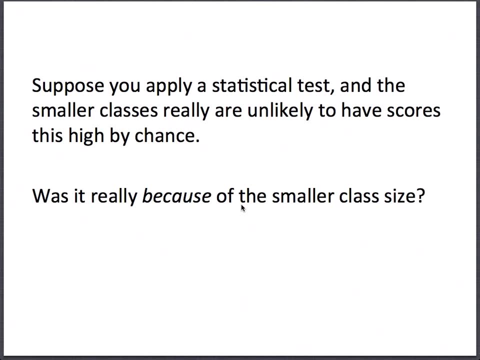 You've all heard correlation, causation. You've all heard correlation is not causation, right? So this is going back to our class example, right? So say we've done the statistical test. We're like you know what This? seeing this much of a difference between the two. 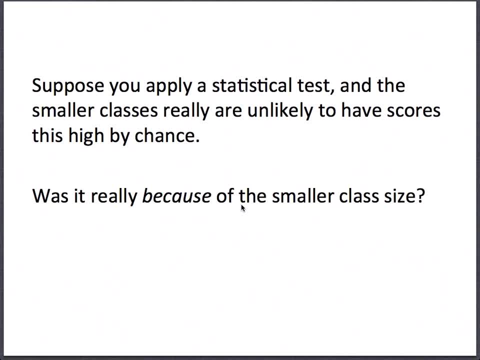 class scores only happens 3% of the time. This is statistically significant. This is a real effect. This class is doing better for reals, Not by chance, we think. But is it really doing better because of why we think it is? 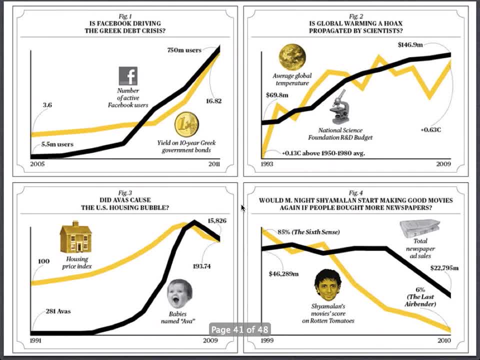 The problem here is that we will make up stories, So look as the number of Facebook users goes up, the Greek debt crisis gets worse As the-. I'm sorry, I'm sorry, I'm sorry, Sorry, I'm sorry. 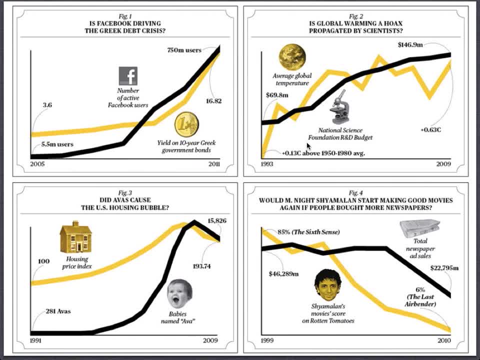 These are correlations. As the NSF budget goes up, the average temperature rises. right, So just be. I mean this is silly, but just because you have a pattern doesn't mean that you have cause. It's just a pattern. So correlation is not causation. 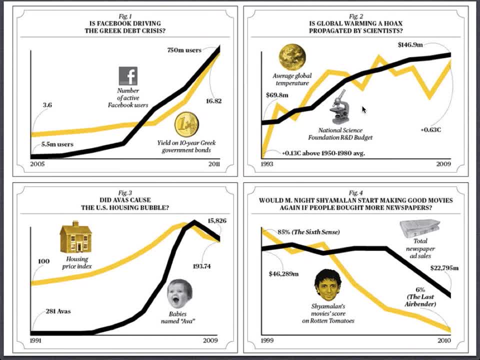 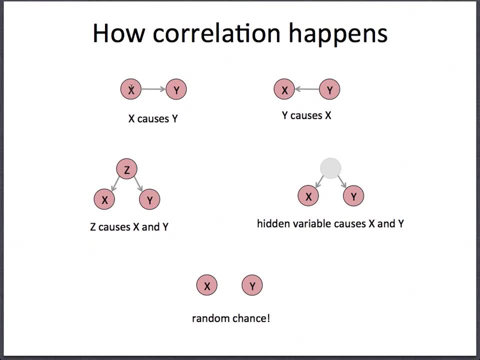 So when you see a pattern, there's only a small number of ways that pattern can occur. This is the one we want. Smaller class size causes better scores. Now, better scores cause small class size. That doesn't really make sense. 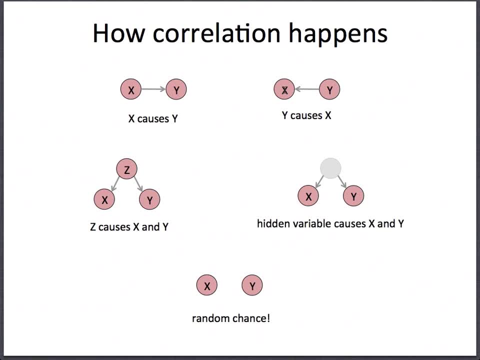 But think about the gun example. A more greater number of homicides causes more people to own guns. That's actually plausible. Maybe people are buying guns because they're scared And you want, or you believe it's the one on the left. but you have to rule out all of these other cases. 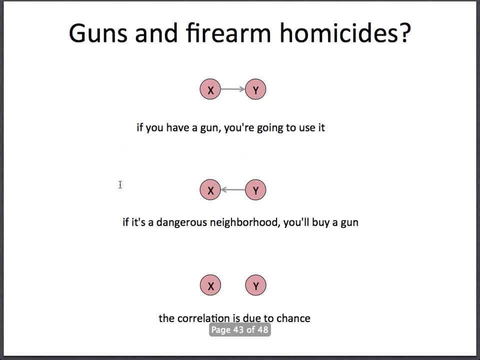 There you go. So that's what we want. If you have a gun, you're going to use it. Here's the other direction. If it's a dangerous neighborhood, you'll buy a gun. Here's another possibility. Perfectly random, right. 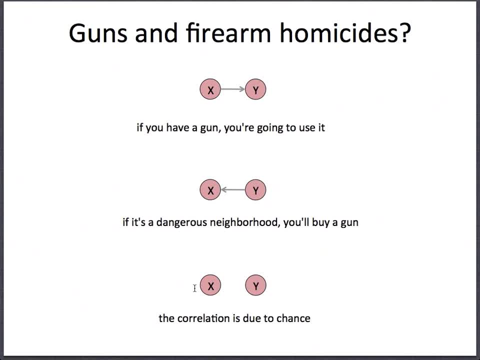 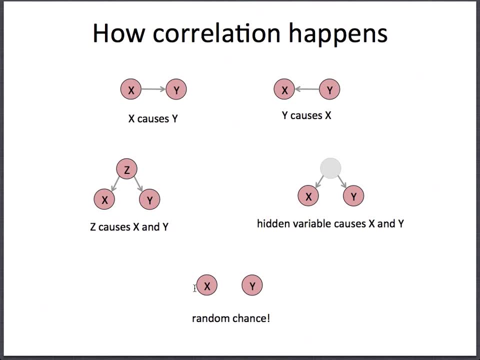 So this one, this bottom one, is what we're ruling out with statistical testing. right, We're ruling out that the relationship is due to chance. Well, we're not ruling it out, but we are putting a bound on the probability. 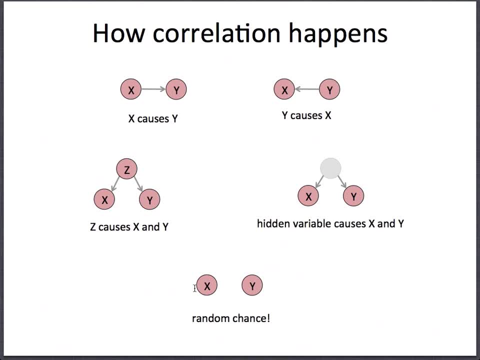 We're saying there's no more than a 5% chance, or 10% chance or whatever percent chance that this is random. That's everything we've done so far is to put that bound. But now we have these other possibilities that we have to rule out as well. 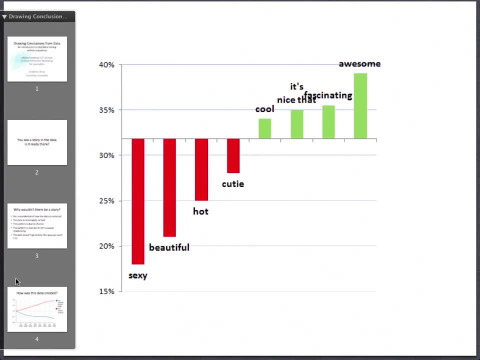 Does anyone read the OK Trends blog? while that was running, It was the data scientist from OKCupid talking about how to make OKCupid work, And one of the things they did is they looked at the response rate versus the words. So if you put the word sexy in your first message, 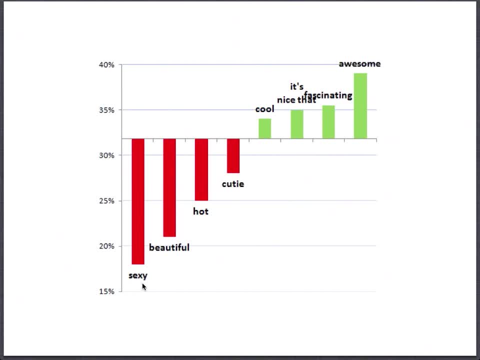 you're going to get 25% or yeah, exactly, Whereas if you put the word awesome it's much higher. So it's very tempting to make a little causal story right If you put the word cutie in your first message. 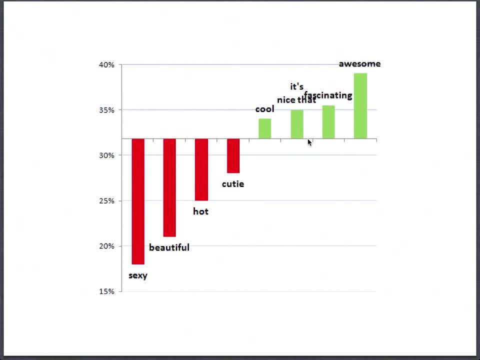 this is men writing to women. The woman's going to. she's not going to write back. That's the story that you want to tell. So if you put the word cutie in your first message, this is men writing to women. The woman's going to. she's not going to write back. 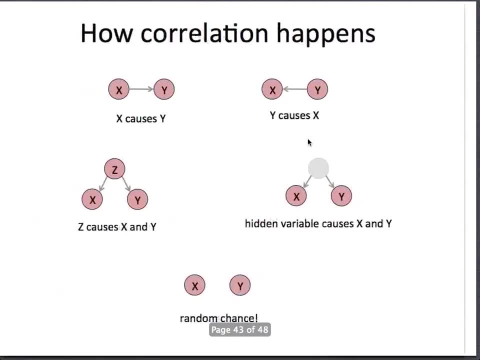 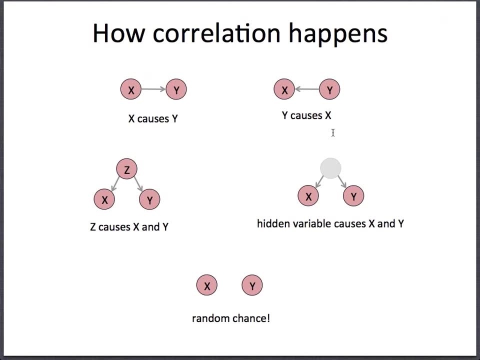 But it could be all of these other cases. Now, obviously you write the message first, so the backwards causality can't happen. She didn't. her not writing back doesn't make you put the word cutie in it, because one happens. 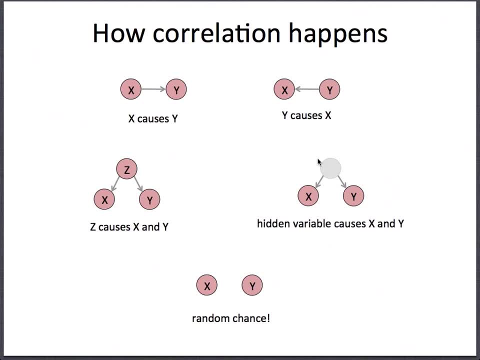 So if there's a temporal order, you can rule out causes sometimes, But what's actually going on in this case is this other thing, There's something else. These two are the same, except sometimes you can see what it is and sometimes you can't. 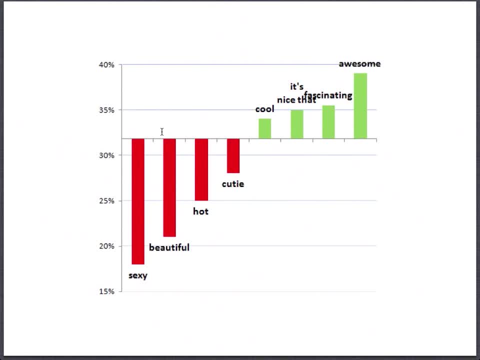 So in this case we're looking for a variable that causes both her not to write back and a guy to use the word hot. So what's the variable that causes both of these things? Maybe hot people are being besieged by lots of notes. 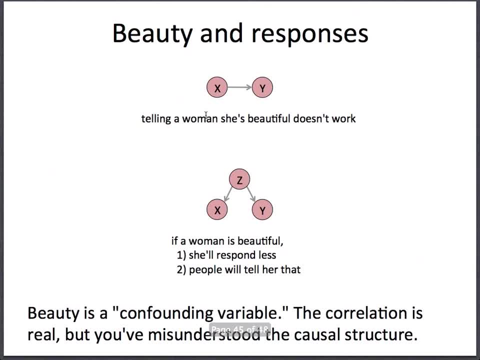 Right. So we look at the data and we think it's this. But what it actually is is this: So this is called a confounding variable. So just because you have a pattern and you've proved the pattern isn't by chance, 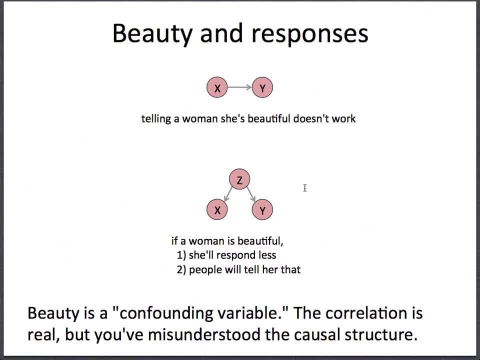 the next step is you have to. you're gonna wanna tell little stories about cause, But there's. you gotta make sure you understand the structure of the causes And luckily there's only five cases, That's it. So you have to rule, you have to figure out. 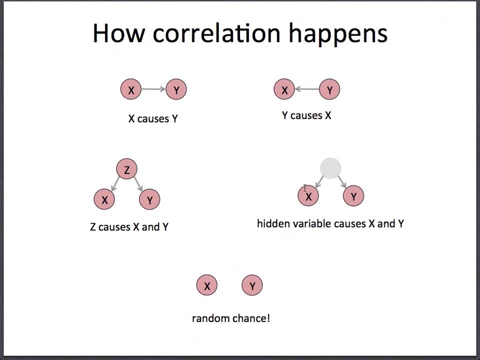 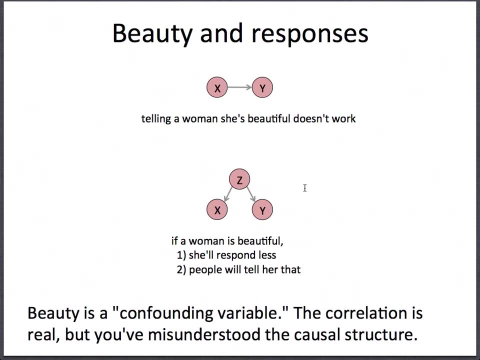 which of these it is, And that means you have to find evidence that it's not these other things. But doesn't that change, I mean? I mean there could be many other reasons, besides the two reasons we put down there, Why she's not responding. 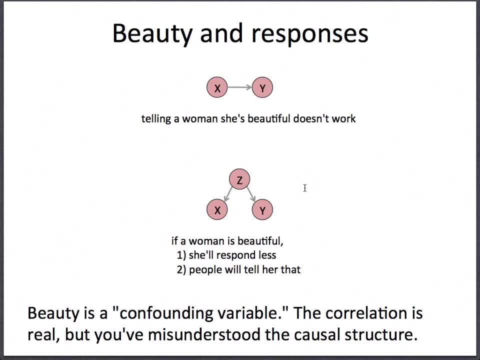 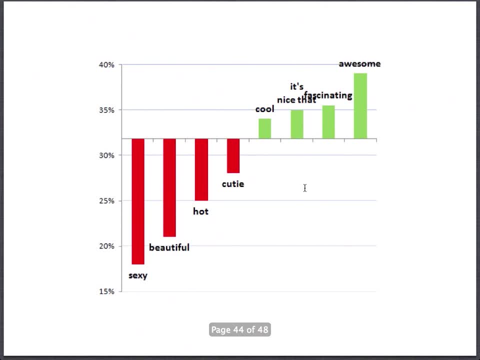 I mean you know. so I mean there are a lot more variables than There's tons of variables. but you're asking the question: Why do I get this relationship? So I've got, I've got two variables: response rate and whether or not I use the word beautiful. 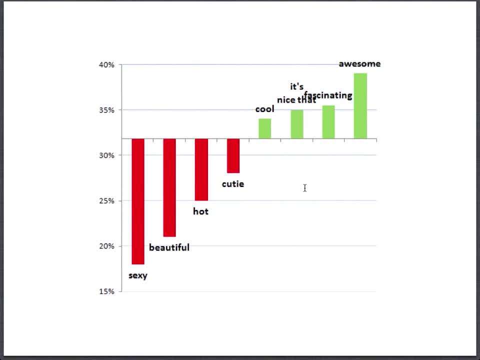 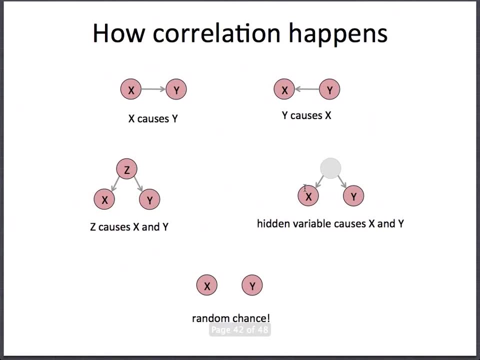 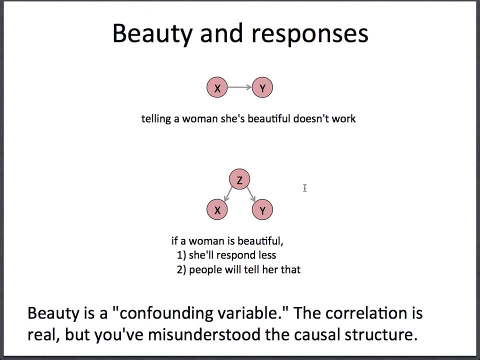 Yeah, And I know there's a pattern, Why, And there's really only a few possible cases, These are all of them, And what you think is telling a woman she's beautiful doesn't work, but what's actually happening is because she's beautiful. 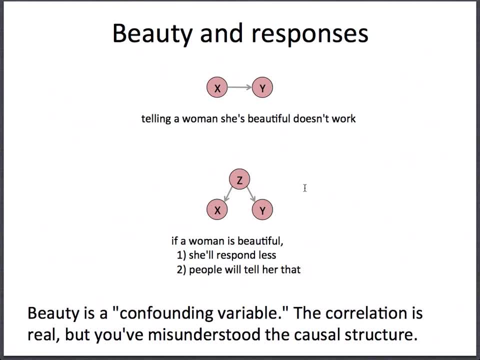 that causes both a lower response and someone to use the word beautiful. So you gotta work out which structure it is. So you gotta work out which structure it is, And normally the way you figure it out is by ruling out the ones that it can't possibly be. 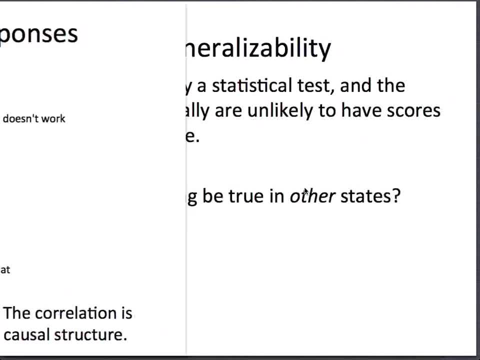 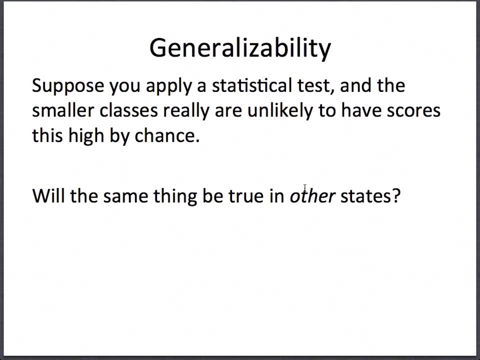 Anyway, we are. We are at time, In fact, they've even stopped filming. So there's one more idea which we're not even going to get into. Yeah, they took away the camera. We're over that much running over. 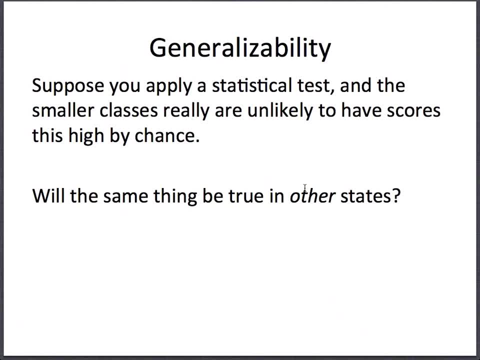 Which is generalizability, right? So this is the idea. Just because you know that a smaller Say. you've done all this work. You've seen a relationship between class size, size and grades. You've shown that the relationship is very unlikely to happen by chance. 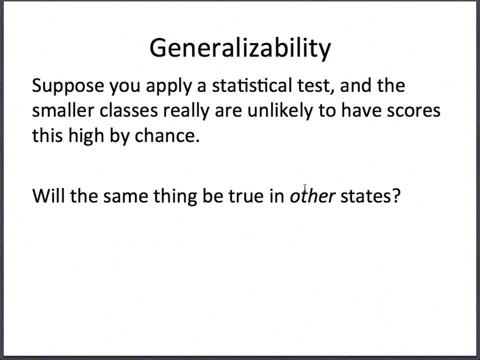 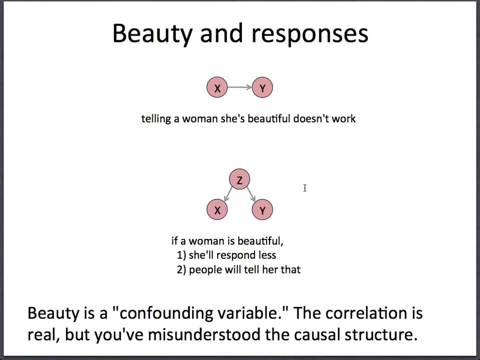 You've shown that the causality runs the way that you think it runs, which is actually very hard to do. You've proved that it's not because better. So for the class size example, right, Maybe it's better funded schools have better trained teachers and smaller class sizes. 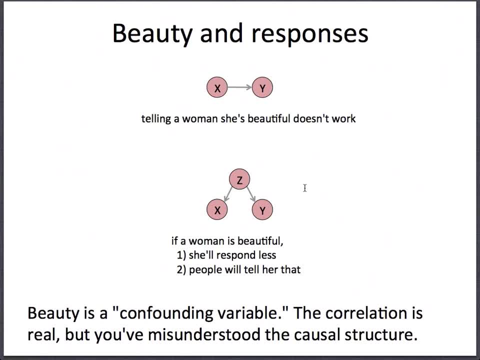 And so the fact that you see a small class size correlating with higher grades doesn't mean that they're getting higher grades because it's a smaller class size. It's just that the better funded schools also pay better teachers, right? So you've got sort of three steps here. 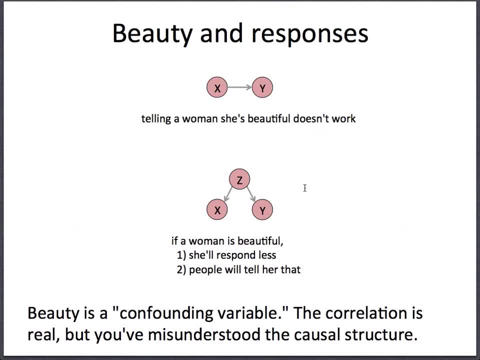 First you have to prove that the pattern doesn't happen by chance, Then you have to prove that the cause is the way you think it is, And then you have to ask yourself: am I going to talk about these schools, or am I going? 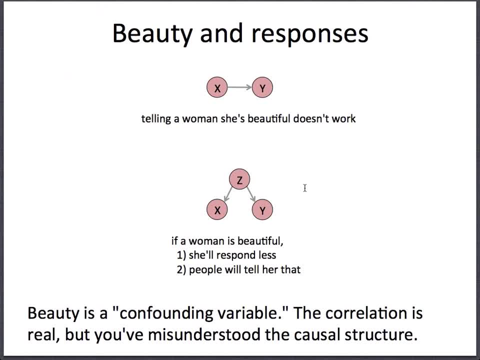 to try to make a point about everything, Because if you're writing a story saying I don't know, I don't know, I don't know, In Rhode Island, smaller classes cause higher grades. Are you implying that it's going to work in Texas as well? 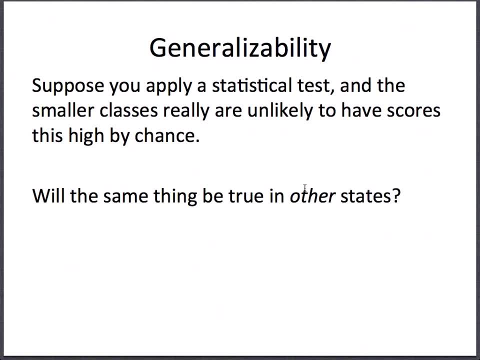 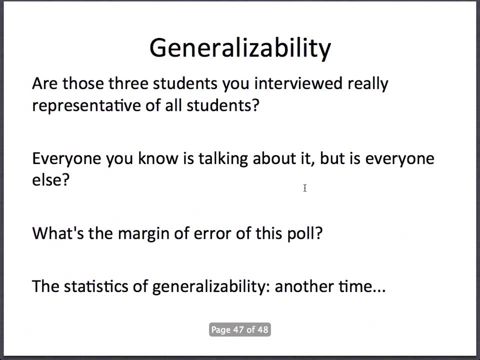 And so you have to think about the generalizability of your results, and that's this whole other tricky area, And statistics can help with that too, but we're not going to talk about it today. Generalizability comes in a lot of different forms. 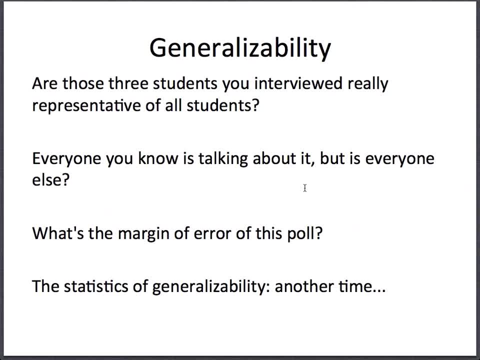 If I interview three people, do they really stand in for this whole group of people If you start to think, well, this is common sense, common knowledge. Everyone believes this Really Because the people that you know are going to be a certain type of person. 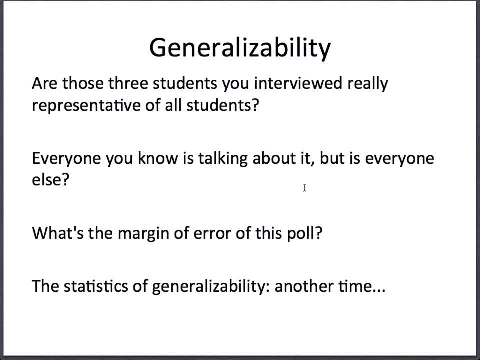 People grouped together with people like them. Margin of error of a poll: same thing. I asked 500 people. This is where statistics comes in again. Is that really representative? The margin of error of a poll addresses this problem of generalizability. 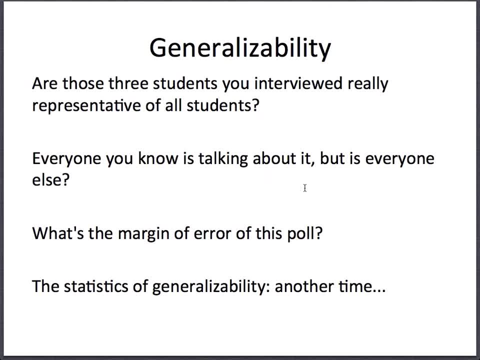 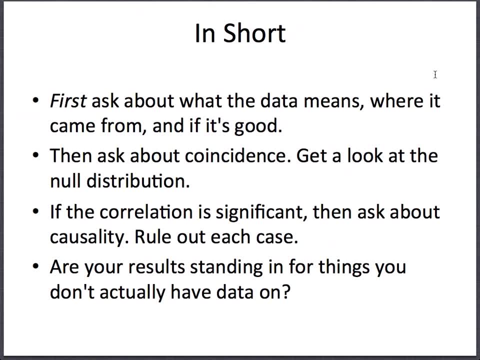 It gives you a chance that the errors It doesn't generalize, but we're not going to talk about that today, Anyway. so this is the short version of how to know if what you're looking at is really there. The first thing you have to do is be skeptical about where the data come from. 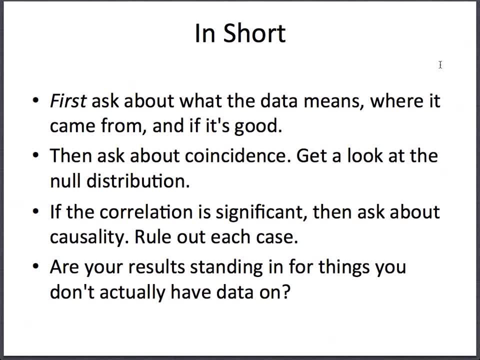 Then you have to establish if the pattern is there by chance or not. And then, even if you do have chance, very often what you really want is a cause. A cause is a whole other problem. And then are you going to imply, or will the reader assume, that these results hold in other? 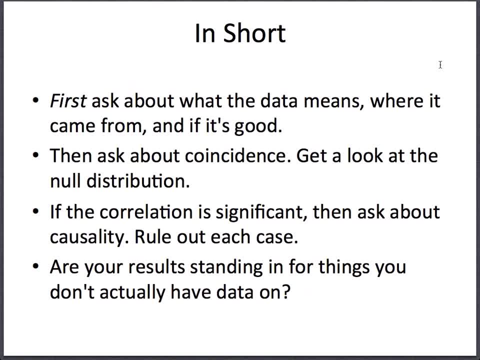 places And if you actually don't know, in Rhode Island putting students in smaller classes in groups grades. we don't know if this will work in California because X, Y, Z. So you have to think about all of the implied generalizations. 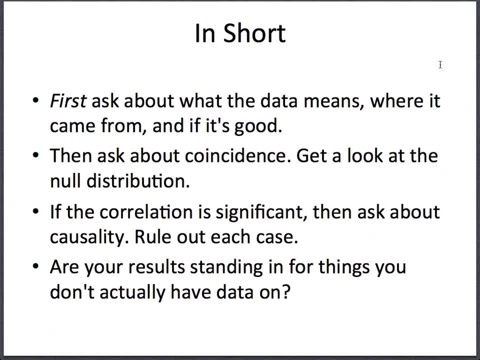 Maybe something completely different, And we see this all the time. right, Environmental policy in one country is going to be different from environmental policy in another. So just because carbon markets worked in Europe doesn't mean they'll work in China necessarily. Now maybe they will, but the point is, you have to make an argument for each of these. 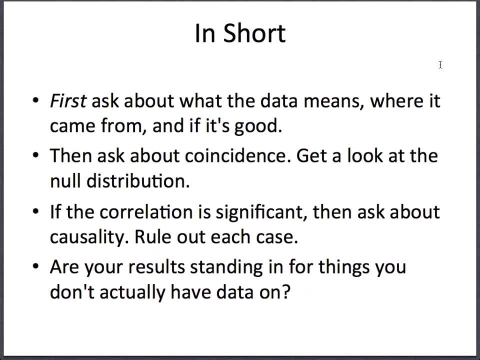 steps. If you miss any one of these, it's very likely you're going to end up with stories that just aren't true. What's that? It happens all the time, But I mean, how can we apply these practical terms? Our situation would be: we get data, we can get more data, but we don't. as you said, 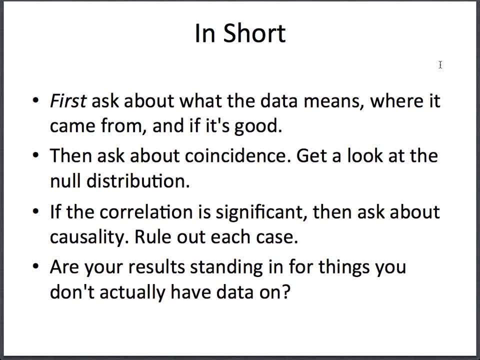 produce data unless we have a way to do the thing which was the best- Go ahead, Okay. kind of things that you showed us. So how can we actually practice what you're telling us? Well, so the shortest answer is: you can say no right. 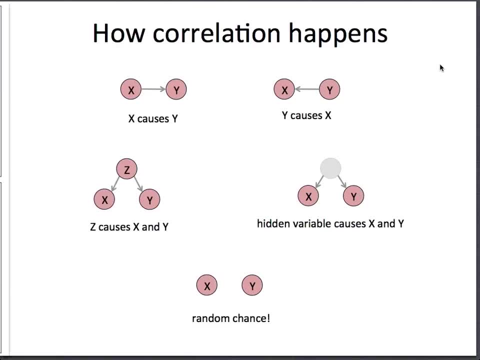 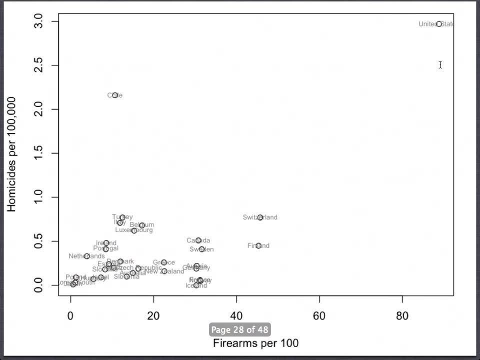 So someone comes to your editor, says: you know, I've looked at this chart of gun violence. Where is it? And man, look at that. Clearly the US is way up there. and then there's this trend, And it's your job. 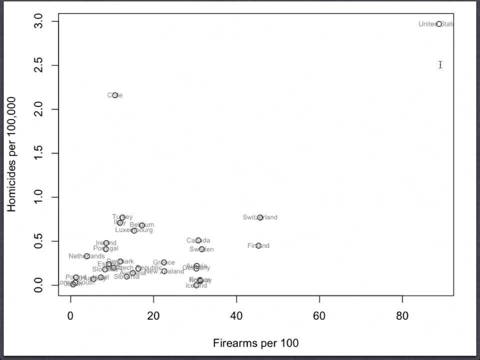 What's that? You can use the line of best fit, GABRIEL KREIMAN- Right, So you can put a line of best fit and, yeah, it goes up, But the thing is how often you know. 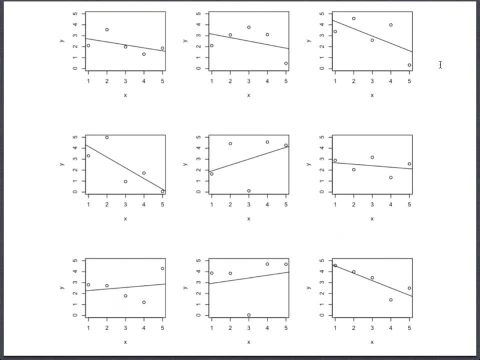 Right, But then I should be able to do something like this, which I'm not. GABRIEL KREIMAN- Right, So use data. I mean you cannot not use data. You have to interpret data as the reality. 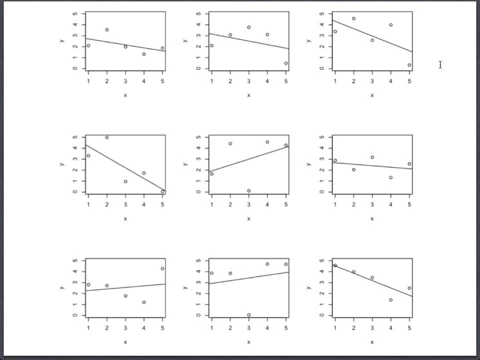 And I personally don't know how to use the software that you just showed, which is very useful, But it's a little bit, you know. So how can I, now that I know where the problems are, how can I put it into a positive way? 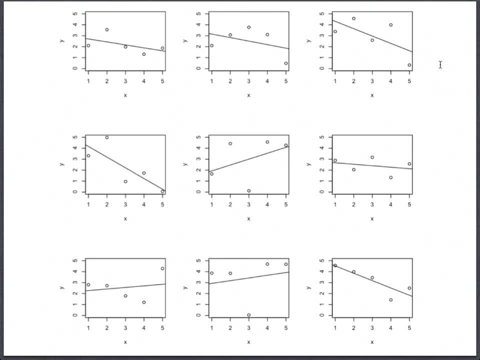 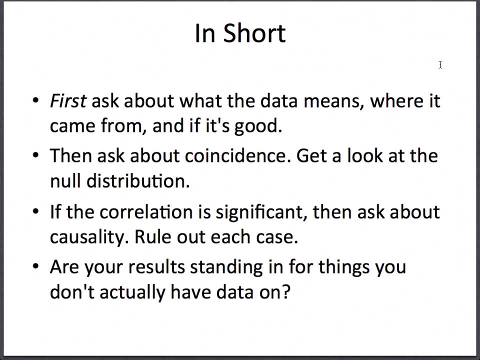 and say: I still have to use data. How can I be reliable? GABRIEL KREIMAN- So I think your job as a reporter is to ask these questions and make sure they have good answers, And maybe you can't do the statistical testing yourself. 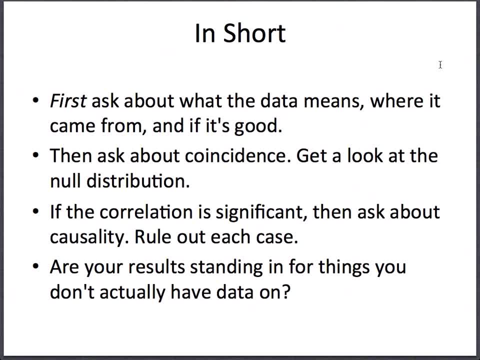 but somebody needs to have done it. So that's either the scientist who wrote the paper, the think tank who's making the claim, or, if there's someone in your newsroom who can do the test, they can do it, Or you find a statistics professor. 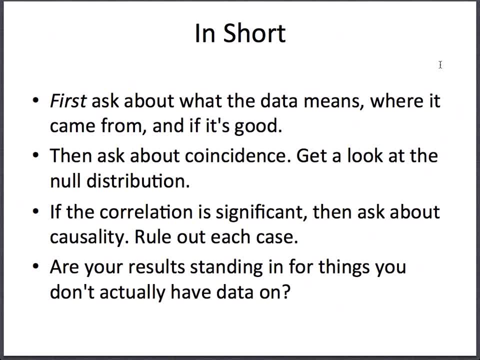 A friend of mine calls this: consult your rabbi When you have a question about the statistical validity. you need to find a rabbi. You need to find an expert who understands the problem and can help you with it. But even if you're not doing the tests yourself, 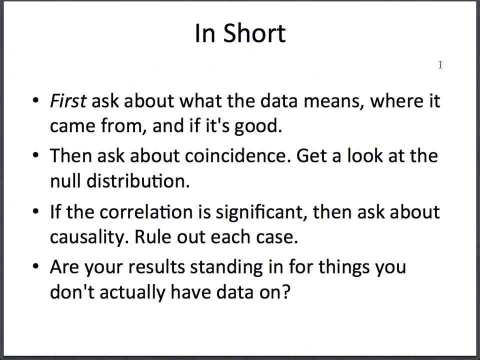 you need to ask these questions. These are the places where you need to be suspicious as a journalist. And maybe that means sorry, we just got to kill the story. Maybe it means the story has a different headline. Maybe it means you find more data. 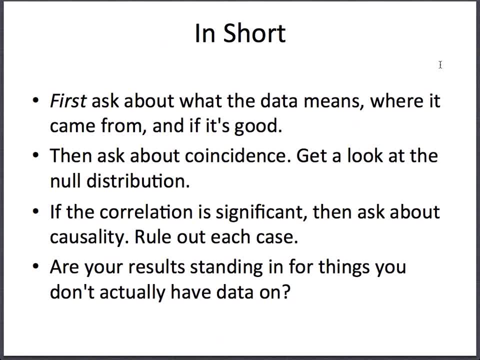 Well, I think any journalist is going to be skeptical of data that they've received If they're decent. they go to a number of different people and say: does this seem true to you, Does this seem possible, Does this seem probable? 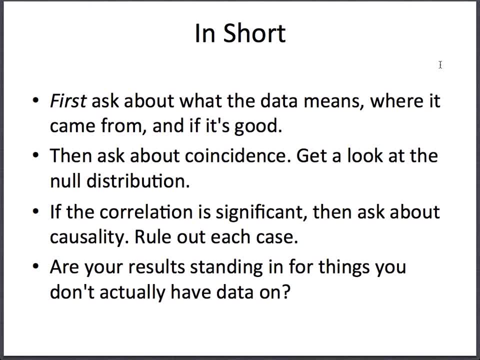 But there is a lot of assumption And especially when someone comes out with something, there are 50 other And if you look at it that way, sometimes you just need one interview with an expert to say nobody's looking at these variables. 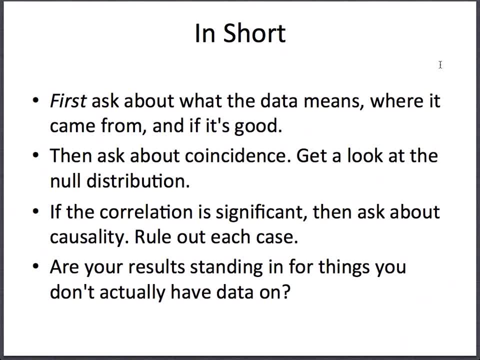 Right, But ask these questions. When someone says: I see this pattern, did it occur by chance, And does the cause work the way I think it does? So yes, asking experts is good, But how you tell if the expert's giving you good answers? 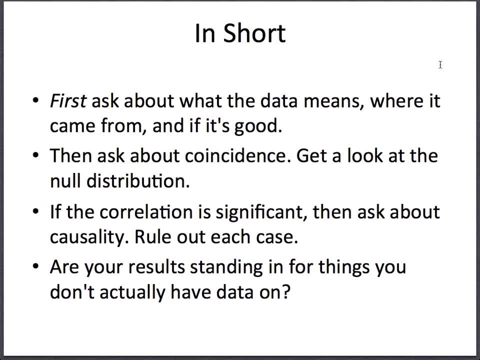 they have to be able to answer these questions. How did I collect this data? What's the odds that I'm going to see this pattern by chance? And I don't mean like, what are the odds? This is not a rhetorical question. 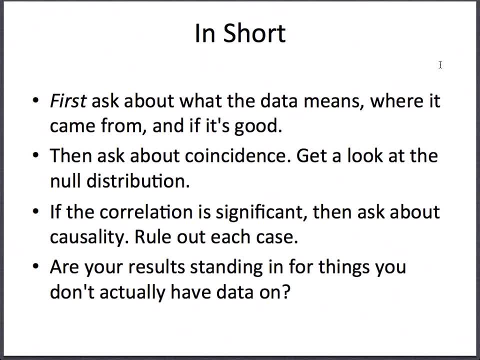 What are the odds is not a rhetorical question. What are the odds is a question that should have a number as an answer. Anytime someone comes up to you and makes an argument about this- couldn't possibly be a coincidence- say oh yeah. 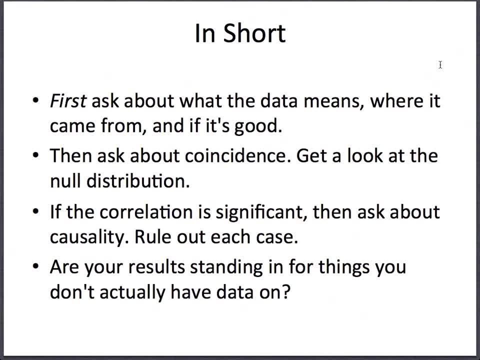 What's the number? And even if you can't calculate it precisely, estimate it. Is it a 50% chance, Is it a 10% chance? And generally in science, a less than 5% chance is what you're looking for. 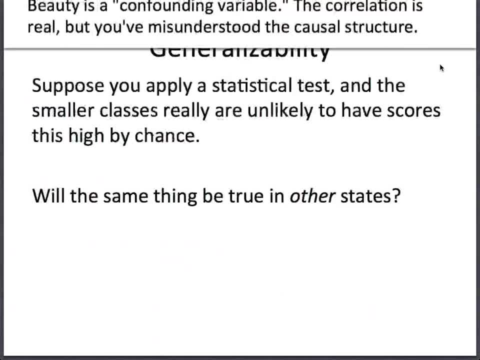 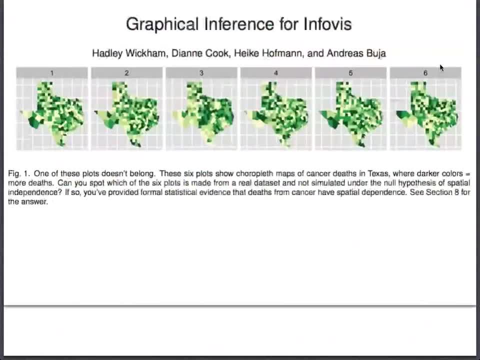 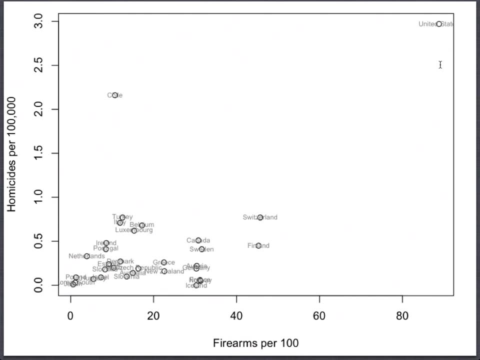 And then there's this causality problem. These charts seem hilarious, But when I show you the gun violence chart, it doesn't seem hilarious. Just because it seems like it makes sense doesn't mean it's true. So you've got to figure out. 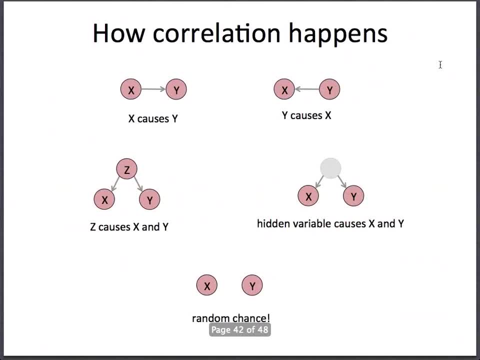 Even when the pattern is real and not a coincidence, you've got to figure out which one of these cases you're in. Luckily there's not very many. You've got to rule them out. And that doesn't even put the political layer. 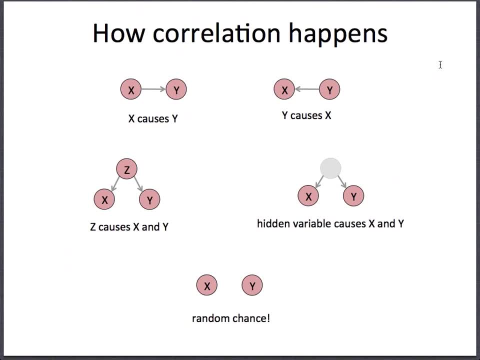 on top of it all- I mean I'm looking at your gun violence things which could be interpreted by one a policymaker to say x and another policymaker to say y. So you've got to, But only one is right. 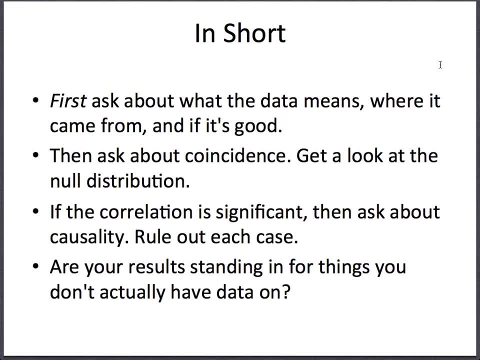 Oh, I know that. I understand that. Yeah, No, I get it. Yeah, I'm curious to know what you think of the story that comes out every single year, which is gun violence. so far, our homicide rate is down this year compared to last year. 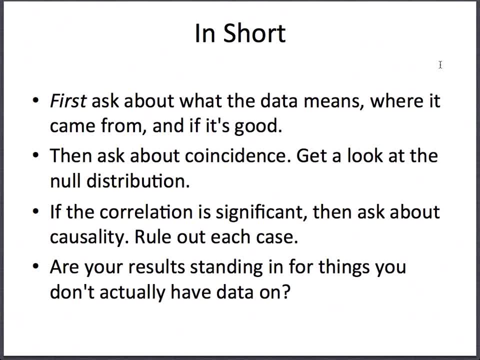 Homicide rate is currently up this year compared to last year. It happens every city, every government, So that's fine. I mean that's a worthwhile thing to report. Where you can get into trouble is gun violence is down this year. 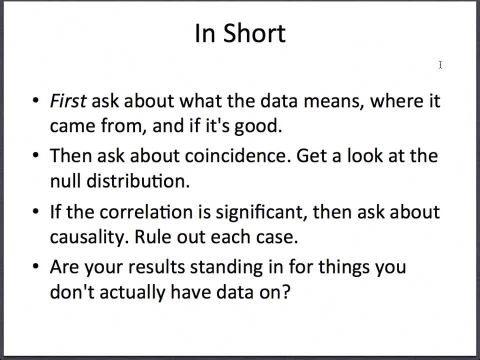 because, And with one year of data, you can almost never say why. But a really good question to ask is: what's the natural variability right? It's that if gun violence has been between 90 and 100 for the last 10 years and now it's 200, that's interesting. 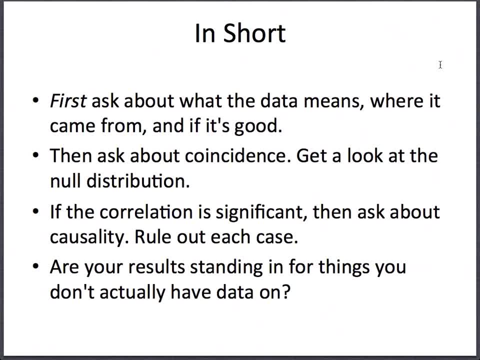 Because that's not likely to happen by chance, right? But if gun violence was 98 last year and it's 92 this year, and it's been between 90 and 100 for the last 10 years, I don't know, And I've actually done this. 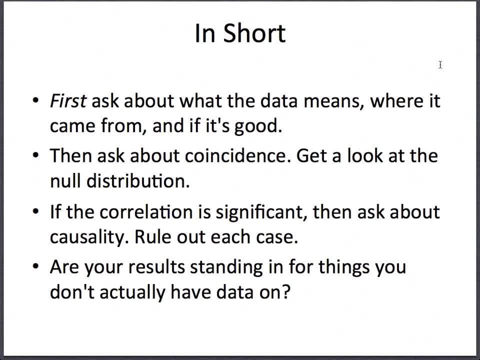 Mother Jones collected data on the number of deaths from mass shooting incidents, And a lot of people are saying it's higher than it's ever been. Well, that's true. However, there's so much variation that that could very easily happen by chance. 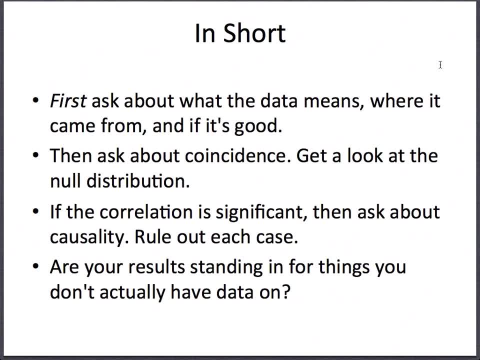 I actually did that statistical test that I showed you where. I just swapped the years and said: how often do I see an increasing trend? And I saw an increasing trend about a third of the time. So I was like, OK, I don't think that's a trend. 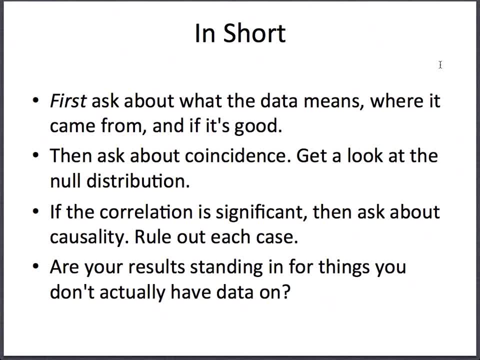 And the cause will creep in right. Because you'll want to say- and financial stories are the worst- energy stocks moved, went significantly lower today after. and they never say because, because they know better than that, They always hedge it. 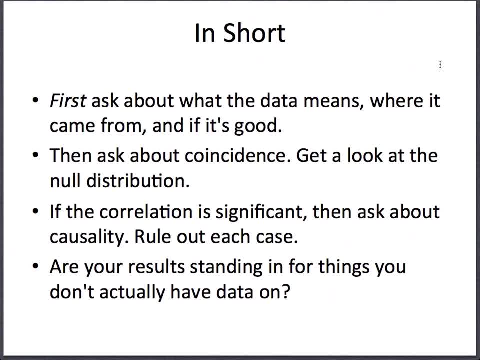 And after announcement of weaker employment figures. After doesn't mean anything, But in the mind of the reader, after means because So don't do it right. It takes a lot of guts as a journalist to say: we don't know. 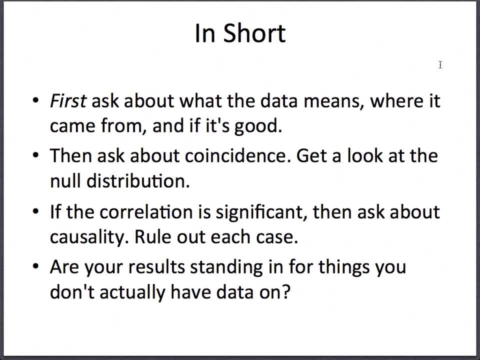 But that's part of, I think, what journalism can learn from. science is we can't tell is very often the most honest answer, And if you can't answer these questions, that's what you've got to go with. Can you try to prove the contrary? 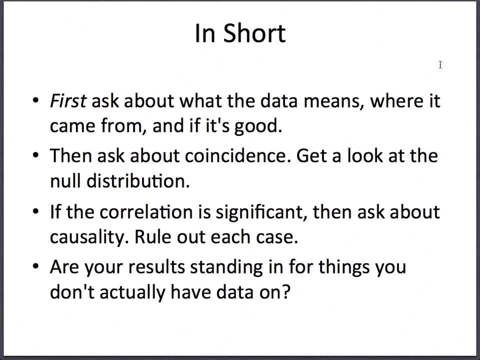 to see if it really counts, For example, in the case of gun violence, to look at which country regulated gun violence and see the immediate result of this. I mean, you wouldn't have one country, but Mm-hmm, Mm-hmm. 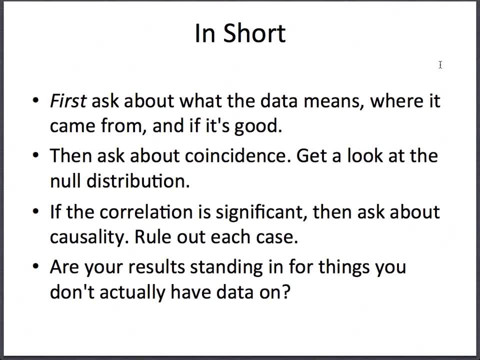 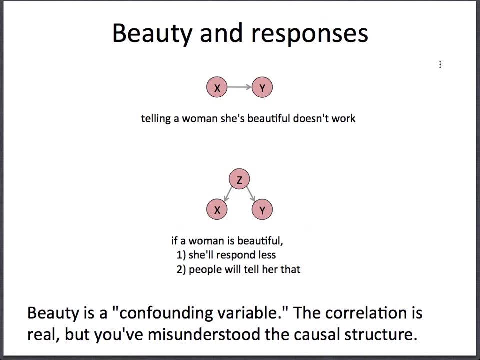 Mm-hmm, Mm-hmm, Mm-hmm. If, in all those countries, the gun deaths decreased, wouldn't that be an interesting indicator? Maybe- Unless it's this problem again right- There may be something that made the countries have. 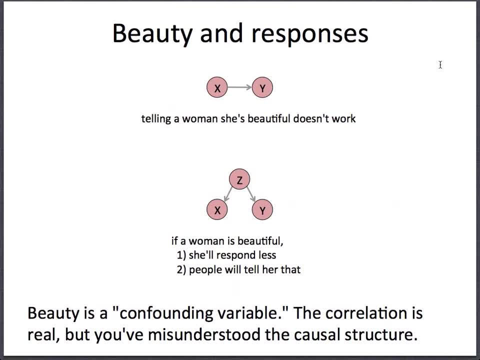 higher regulation and made the gun violence decrease. You can never get away from this, right, Mm-hmm You? The short answer is no. You always have to do this. Now, if you can make an argument, why there's no other reason? 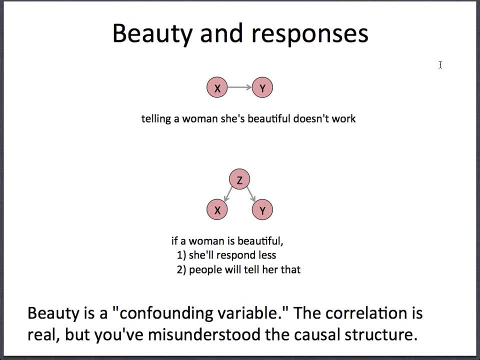 that the gun violence levels have changed, then you've got something. But that's a very hard argument to make And in fact researchers have been working on this problem for decades And it's hard. We're not able to conclusively say that the you know. 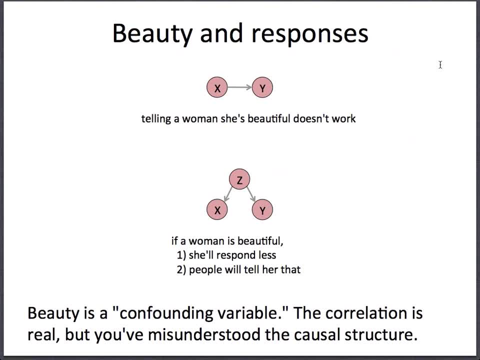 any particular policy or cultural factor has an effect. No, but you might have, I mean you might have you know countries that have managed to decrease the- you know- gun death? Maybe it's not only by you know, by regulating strictly. 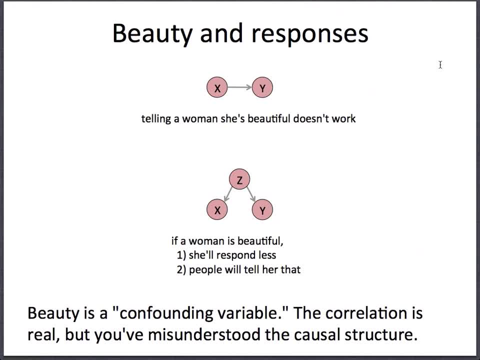 Mm-hmm, But it's still worth seeing what has been done. Yeah, absolutely, Or you take that: just take only the country that experienced gun death decrease and see if there is a pattern. Mm-hmm And the things that you know. gun control might not be the only thing. 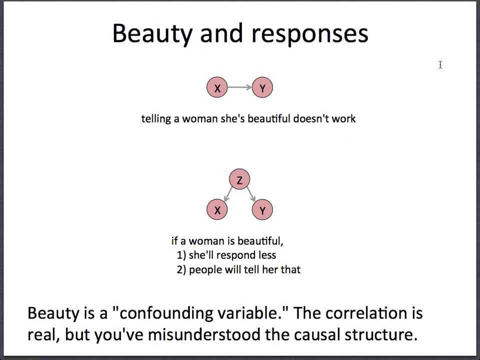 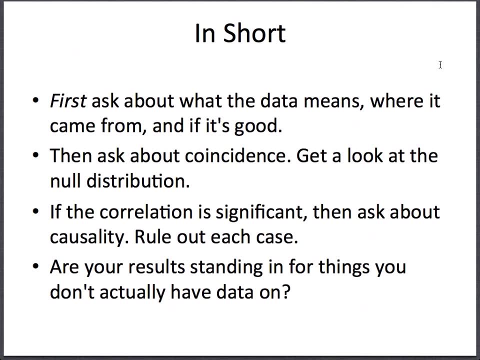 but doesn't that say something? Maybe You still have to put it through. Look, it doesn't matter what you do, You have to put it through these tests, right? It doesn't matter what it is, It can still be by chance. 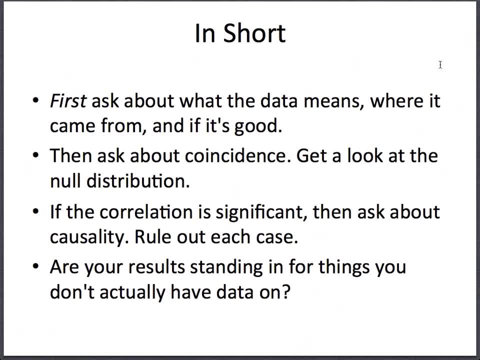 You can still have the causal structure wrong, It can still generalize wrong, The data can still be bad. It really doesn't matter. You have to ask these questions. I mean now you're asking. I mean you're asking a point which is 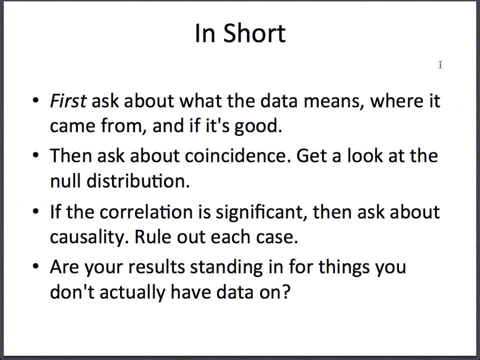 can I look in other directions for other types of relationships? Yes, absolutely, But there's nothing that will get you out of responsibility for doing less, So you could. I was thinking that, being careful that you said so. it would be like a phrase that I hear, would be like: